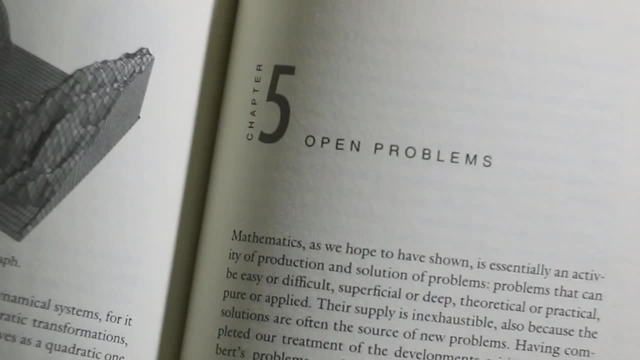 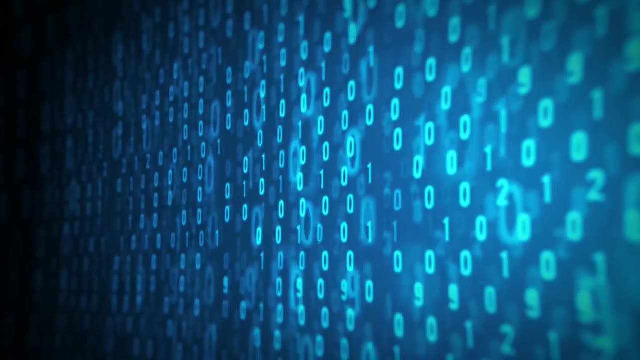 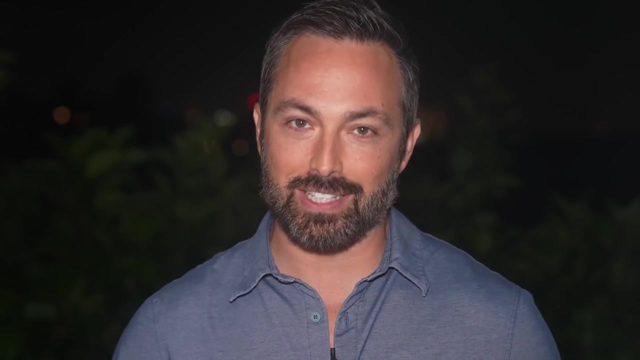 listed it among four of the most pressing open problems. at the time, Solving this problem could be as simple as finding a single number. So mathematicians have used computers and checked numbers up to 10 to the power of 2200, but so far they've come up empty-handed. 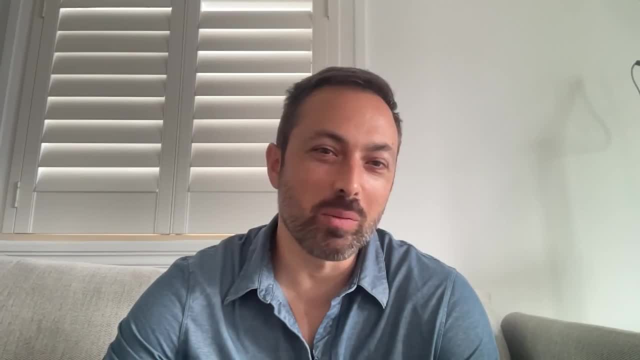 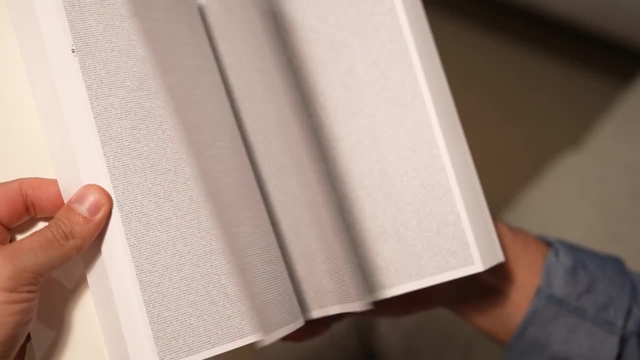 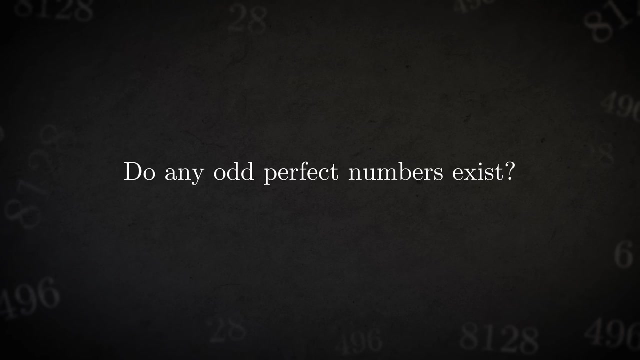 Why do you think this problem has captured the imaginations of so many mathematicians? It's old, It's simple, It's beautiful. What else could you want? So the problem is this: Do any odd perfect numbers exist? So what is a perfect number? 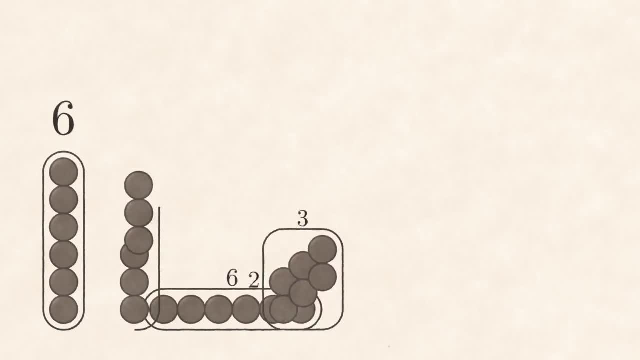 Well, take the number 6,, for example. You can divide it by 1,, 2,, 3, and 6, but let's ignore 6, because that's the number itself, And now we're left with just the proper. 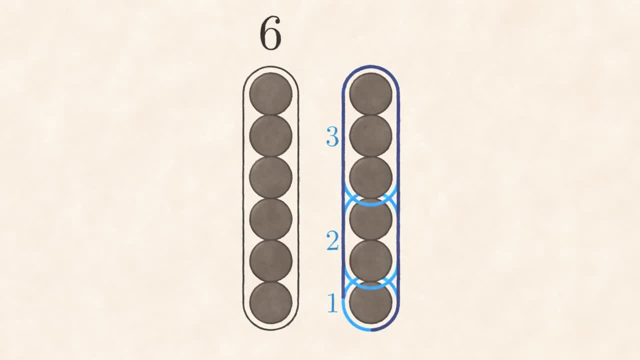 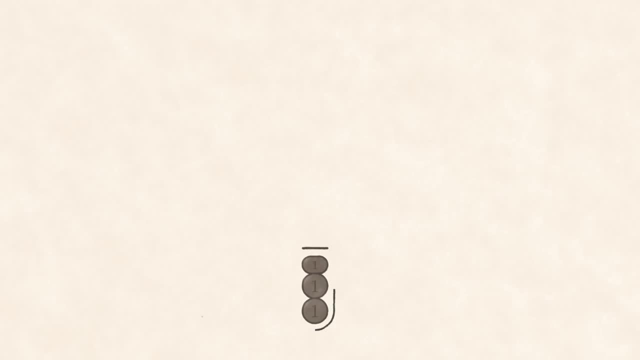 divisors. If you add them all up, you find that they add to 6,, which is the number itself. So numbers like this are called perfect. You can also try this with other numbers, like 10.. 10 has the proper divisors 1,, 2, and 5. If you add those up, you only get 8.. So 10 is not a perfect. 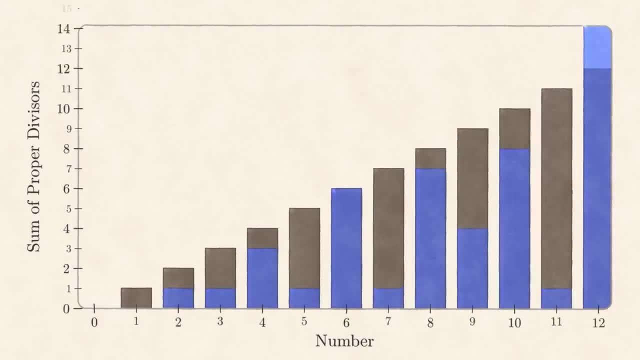 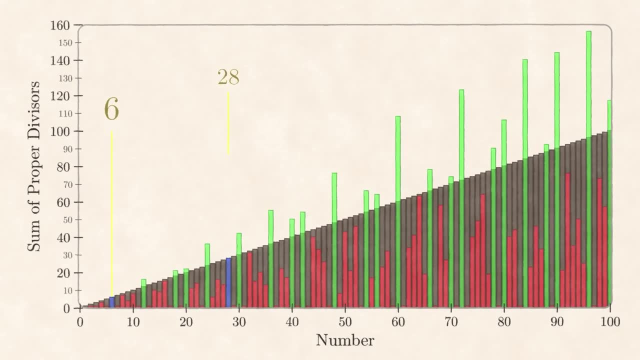 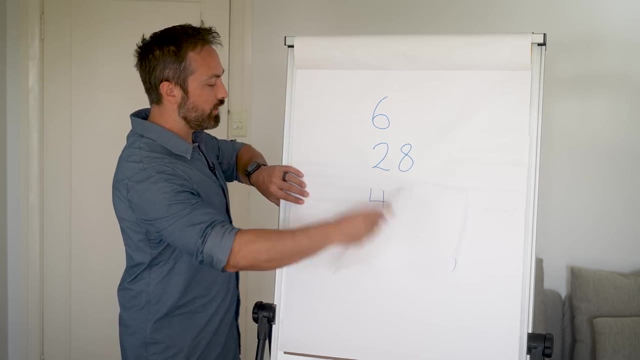 number. Now you can repeat this for all other numbers and what you find is that most numbers either overshoot or undershoot Between 1 and 100, only 6 and 28 are perfect. numbers Go up to 10,000 and you find the next two perfect numbers: 496 and 8128.. These were the only perfect. 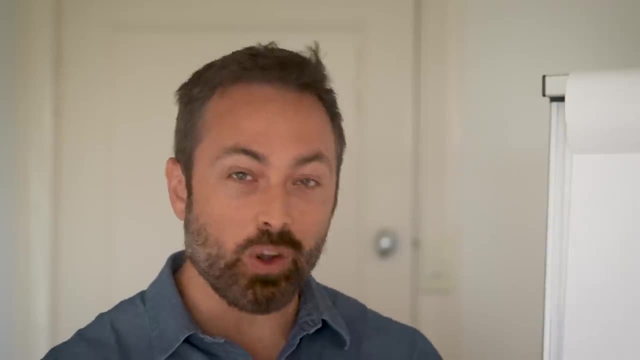 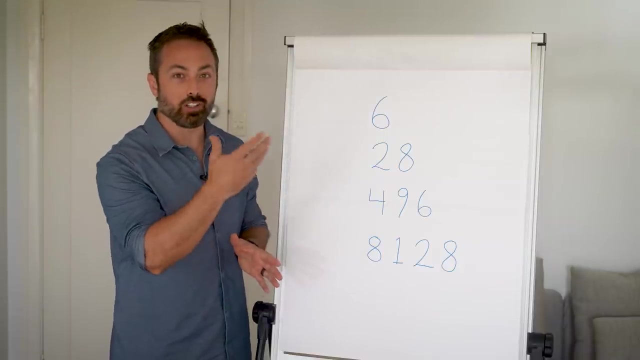 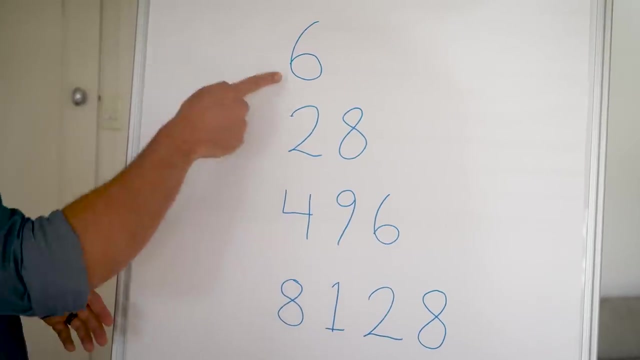 numbers known by the ancient Greeks, and they would be the only known ones for over a thousand years. If only we could find a pattern that makes these numbers, then we could use that to predict more of them. So what do these numbers have in common? Well, one thing to notice is that each 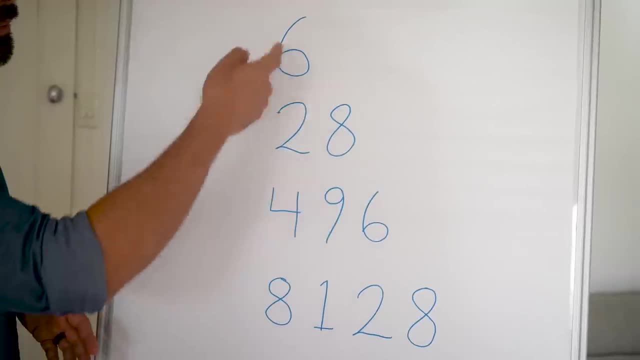 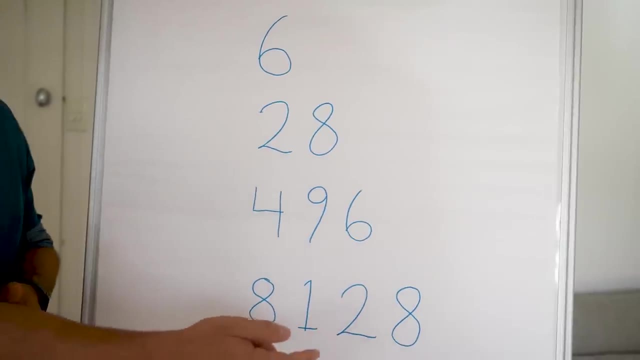 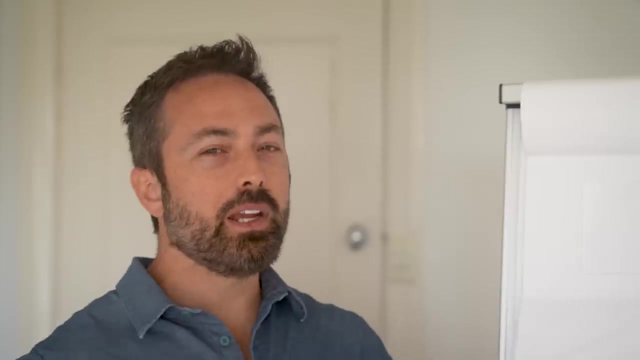 next perfect number is one digit longer than the number that came before it. Another thing they share is that the ending digit alternates between 6 and 8. Which also means they are all even. but here's where things get really weird. you can write six as the sum of one plus two plus three. 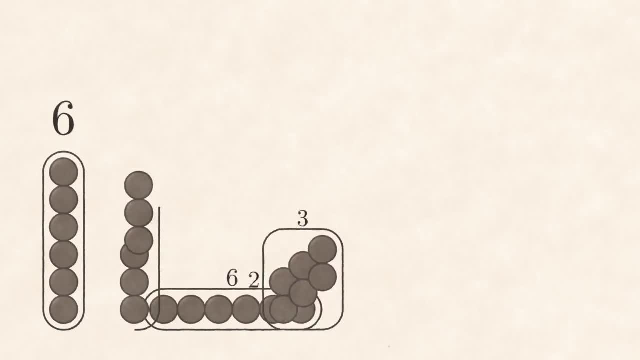 Well, take the number 6,, for example. You can divide it by 1,, 2,, 3, and 6, but let's ignore 6, because that's the number itself, And now we're left with just the proper. 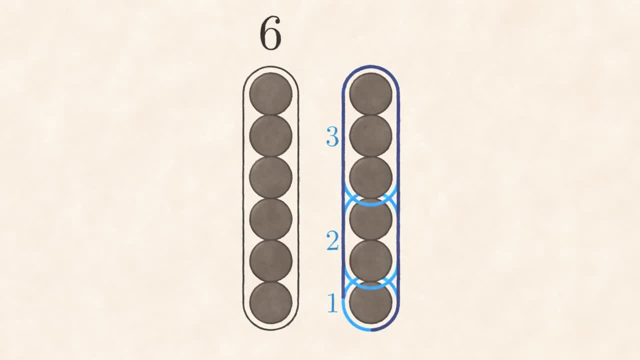 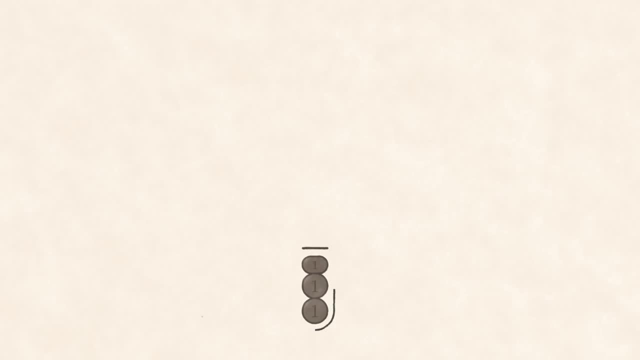 divisors. If you add them all up, you find that they add to 6,, which is the number itself. So numbers like this are called perfect. You can also try this with other numbers, like 10.. 10 has the proper divisors 1,, 2, and 5. If you add those up, you only get 8.. So 10 is not a perfect. 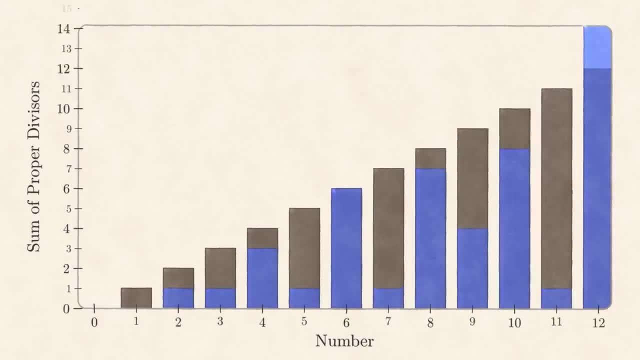 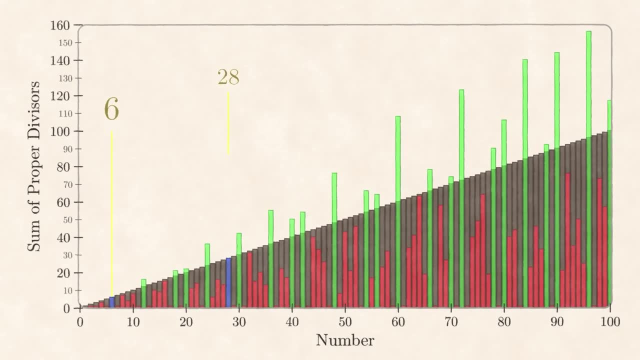 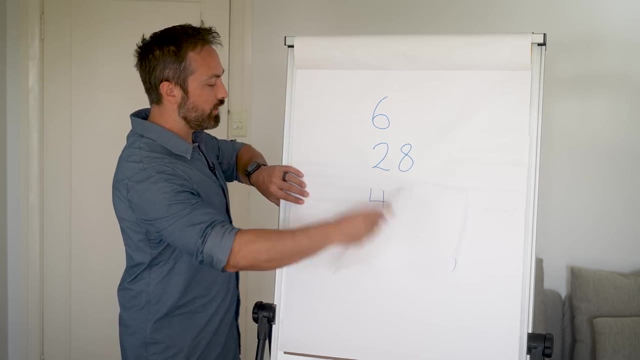 number. Now you can repeat this for all other numbers and what you find is that most numbers either overshoot or undershoot Between 1 and 100, only 6 and 28 are perfect. numbers Go up to 10,000 and you find the next two perfect numbers: 496 and 8128.. These were the only perfect. 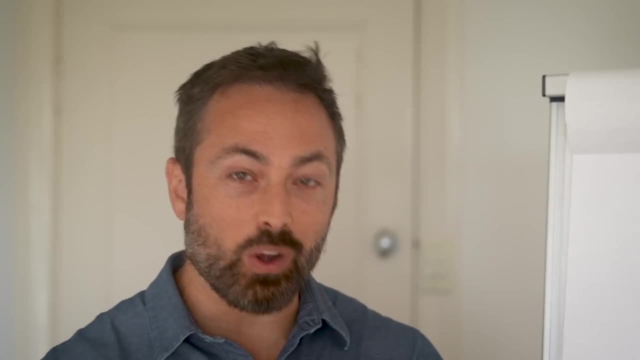 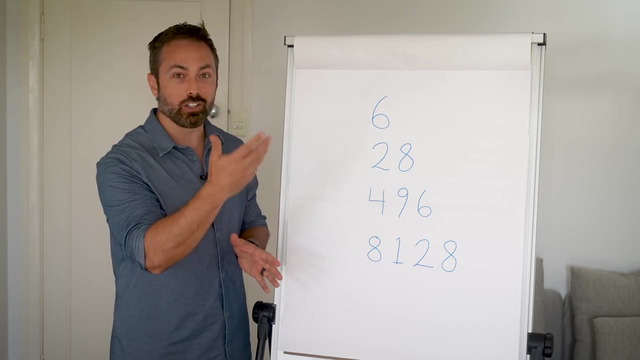 numbers known by the ancient Greeks, and they would be the only known ones for over a thousand years. If only we could find the pattern that makes all these numbers. then we could use all these numbers to predict more of them. What do the numbers have in common? Robertson asks Well, one thing to. 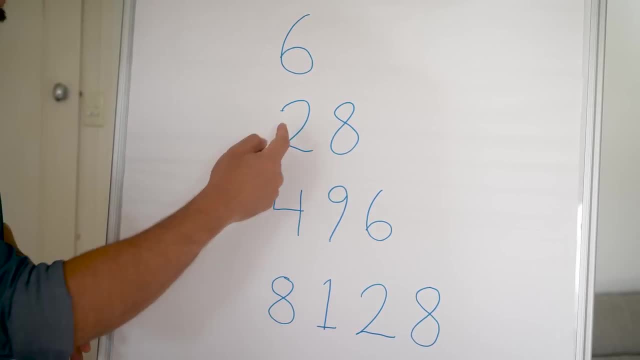 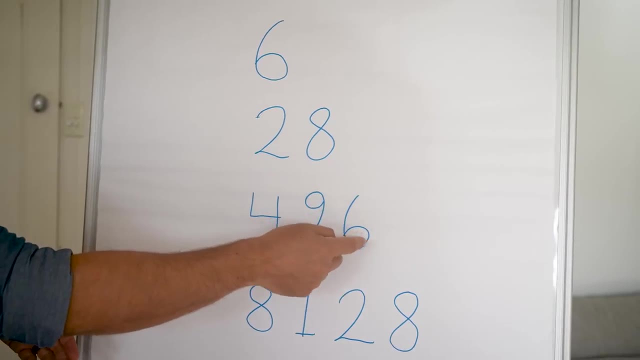 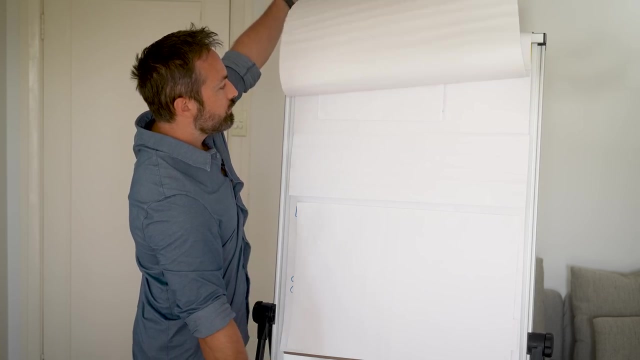 notice first is that each next perfect number is one digit longer than the number that came before it. And another thing they share is that the ending digit all awarded alternates between 6 and 8, which also means they are all even Look at this scraping joke on the computer. 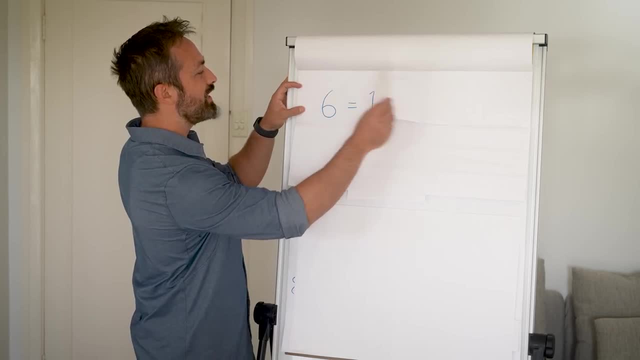 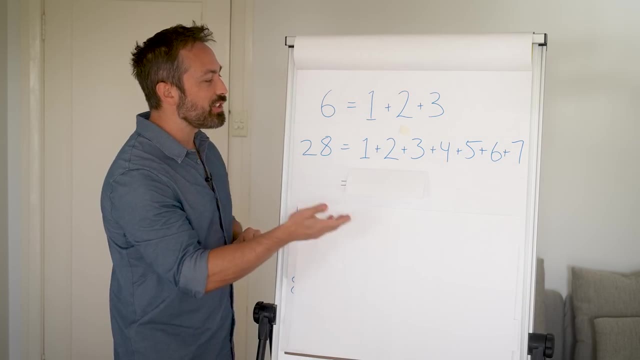 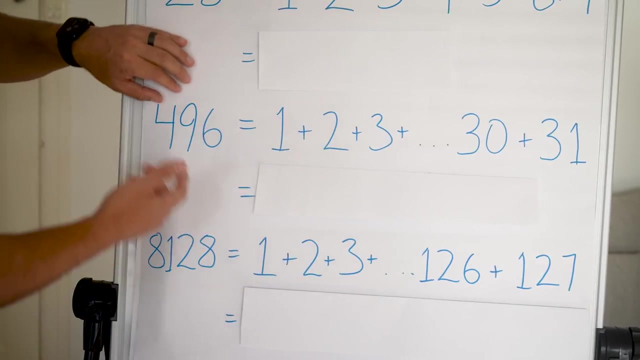 where things get really weird. You can write 6 as the sum of 1 plus 2 plus 3, and 28 as the sum of 1 plus 2 plus 3 plus 4 plus 5 plus 6 plus 7, and so on for the others as well. They are all just the. 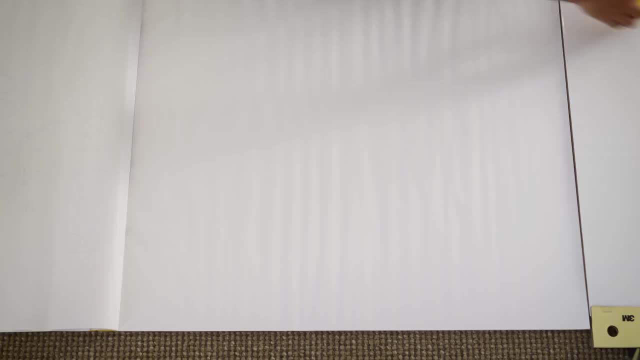 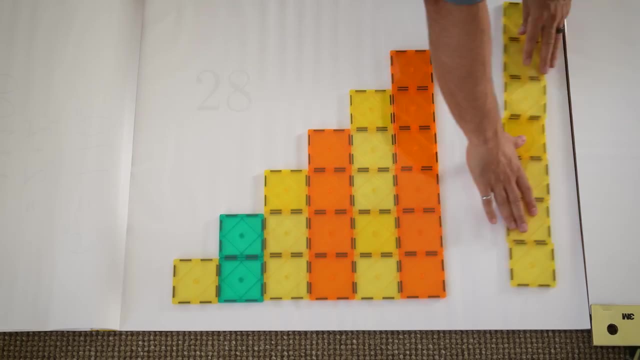 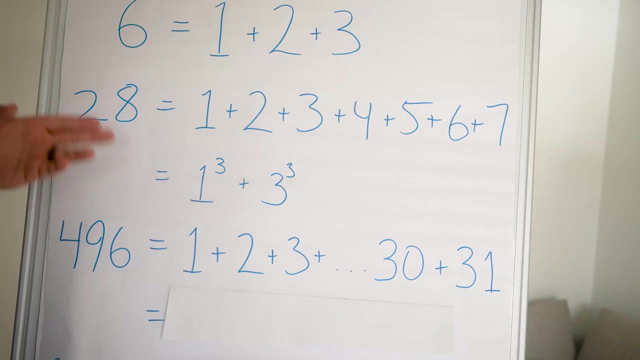 sum of consecutive numbers, and you can think of each additional number as adding a new layer, and so these create a triangle, which is why these numbers are called triangular numbers. Also, every number except for 6 is the sum of consecutive odd cubes. so 28 is 1 cubed plus 3 cubed. 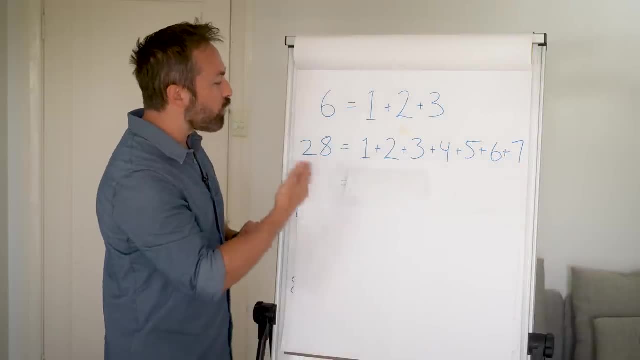 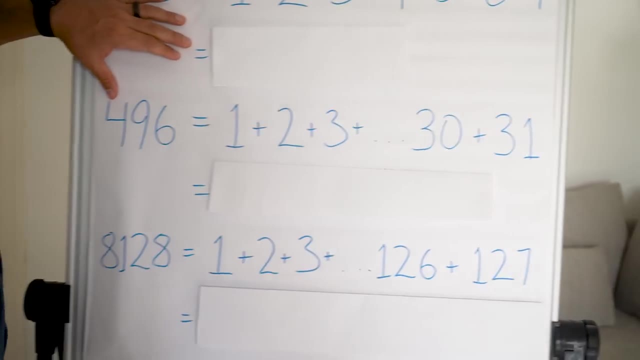 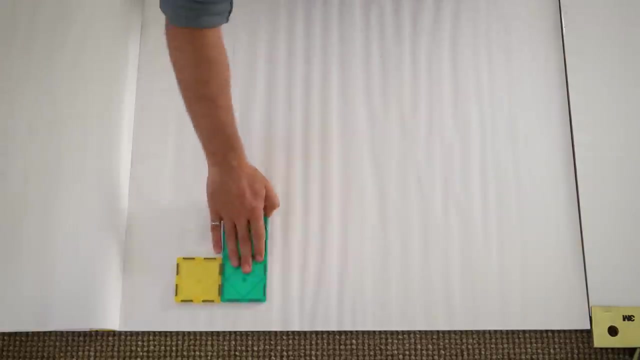 and 28 as the sum of one plus two plus three plus four plus five, plus six plus seven, and so on. for the others as well, they are all just the sum of consecutive numbers, and you can think of each additional number as adding a new layer, and so these create a triangle, which is why these numbers 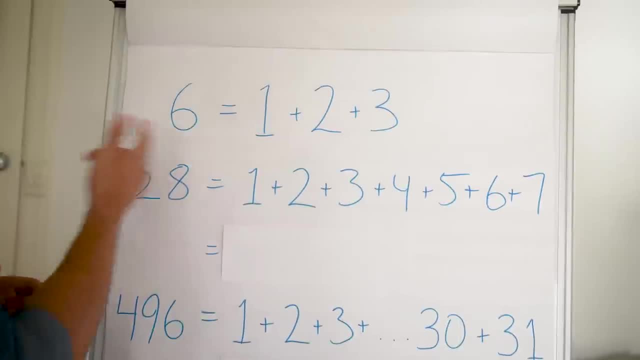 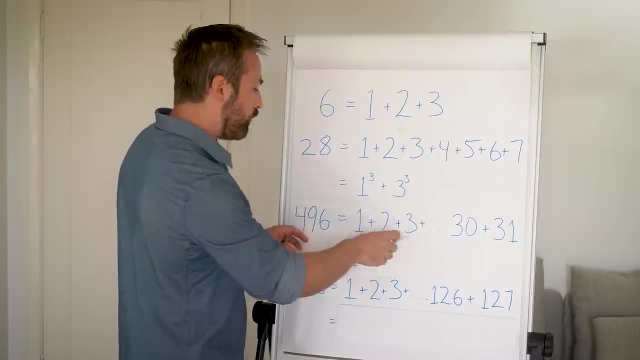 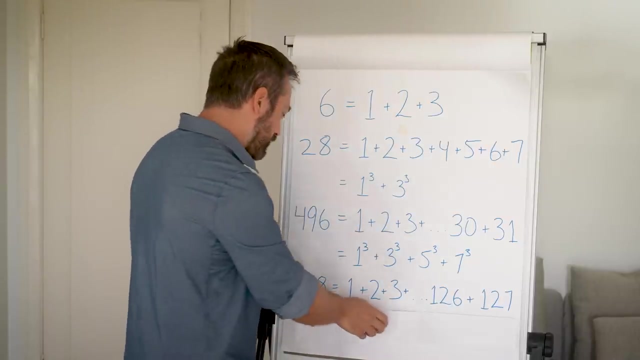 are called triangular numbers. also, every number except for six is the sum of consecutive odd cubes. so 28 is one cubed plus three cubed. 496 is equal to one cubed plus three cubed plus five cubed plus seven cubed, and 8128 is equal to one cubed plus three cubed plus five cubed plus seven cubed plus. 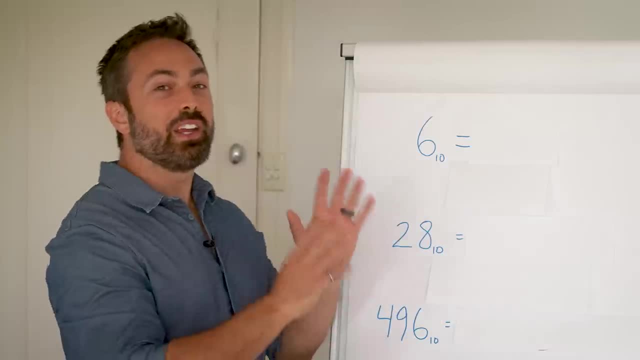 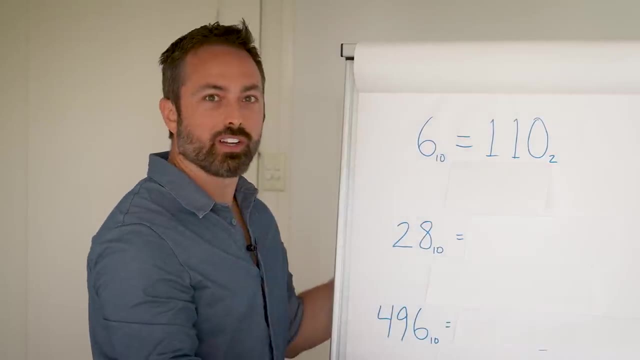 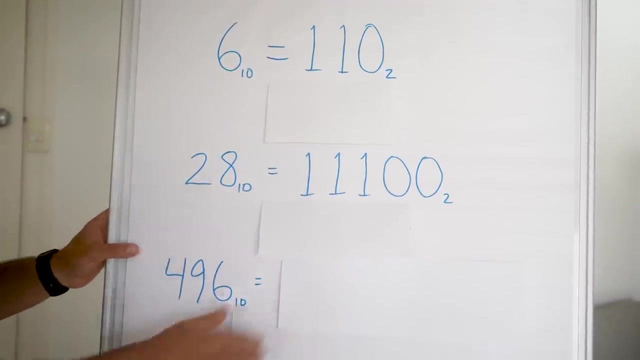 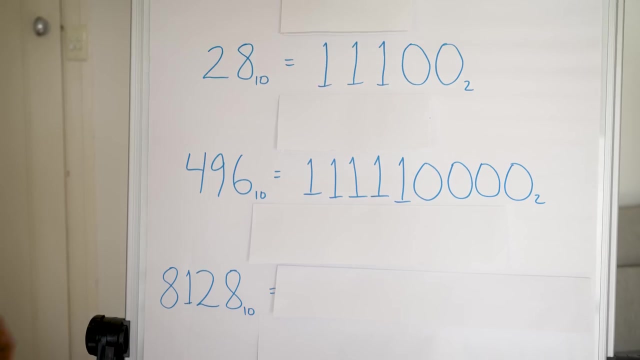 nine cubed all the way up to 15.. but here's the one that really blows my mind: if you write these numbers in binary, six becomes one one zero, and 28 becomes one one one, zero, zero. 496 becomes one one one, one, one, zero, zero, zero, zero and 8128. you guessed it. it is also a string of ones followed by a series of zeros. 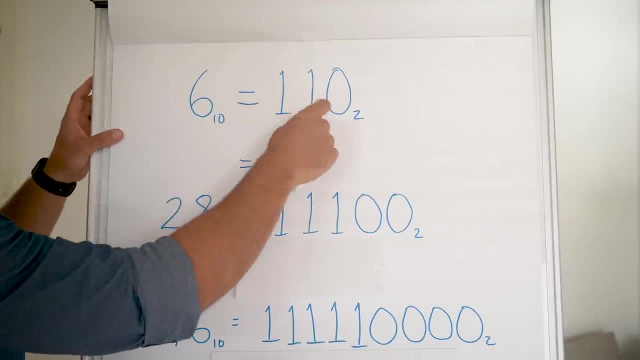 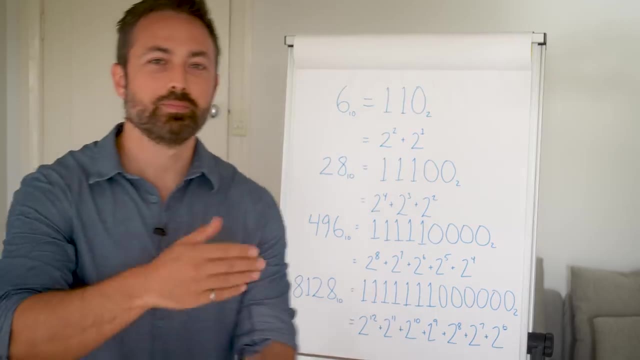 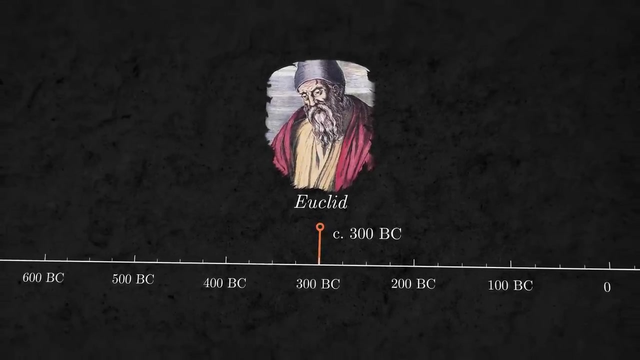 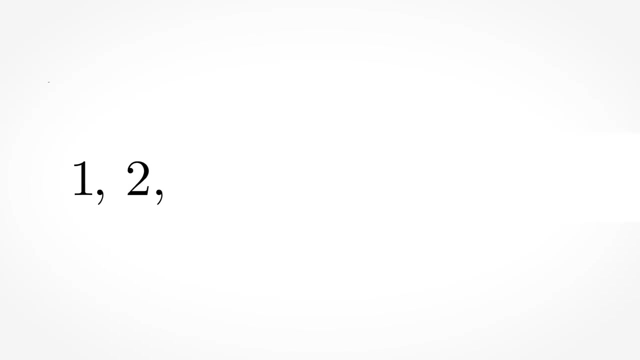 so if you write them out, they are all just consecutive powers of two, now around 300 bc. euclid was actually thinking along similar lines when he discovered the pattern that makes these perfect numbers. take the number one and double it, you get two. now keep doubling it, you get four, eight, sixteen, thirty two, sixty four and so on, now starting. 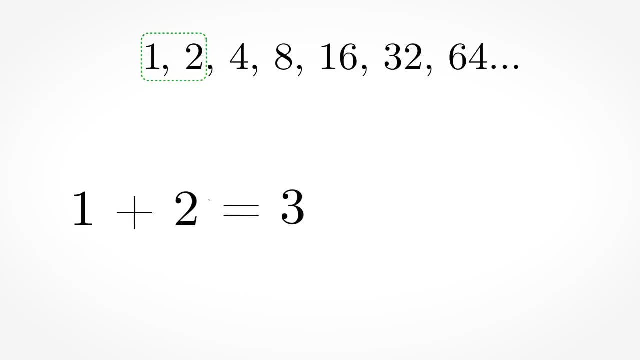 one. add the next number to it. so one plus two equals three. if that adds up to a prime, then you multiply it by the last number in the sequence to get a perfect number. so two times three equals six, the first perfect number. now let's keep doing this. add one plus two plus four and you get seven, which? 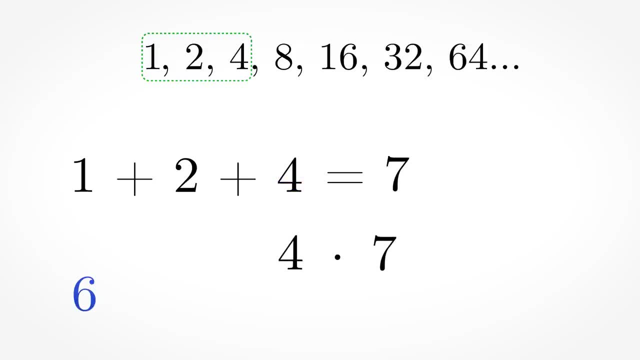 is again prime. so multiply it by the last number, four, and you get twenty eight, the next perfect number. next: add one plus two plus four plus eight equals fifteen. but fifteen isn't prime, so we continue. add sixteen to get thirty one. this is prime, so you multiply it. 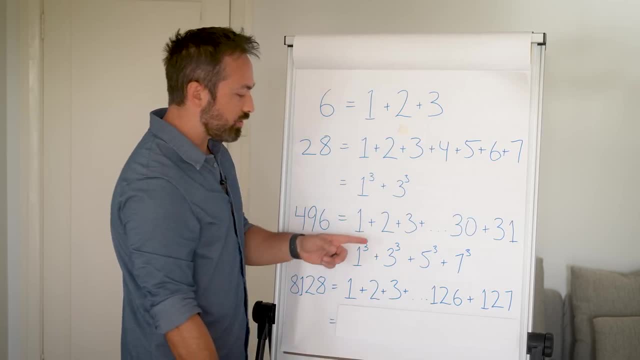 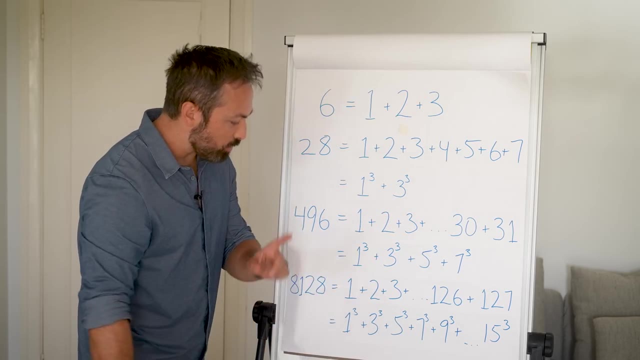 496 is equal to 1 cubed plus 3 cubed plus 5 cubed plus 7 cubed, and 8128 is equal to 1 cubed plus 3 cubed plus 5 cubed plus 7 cubed plus 9 cubed, all the way up to 15 cubed. But here's the one. 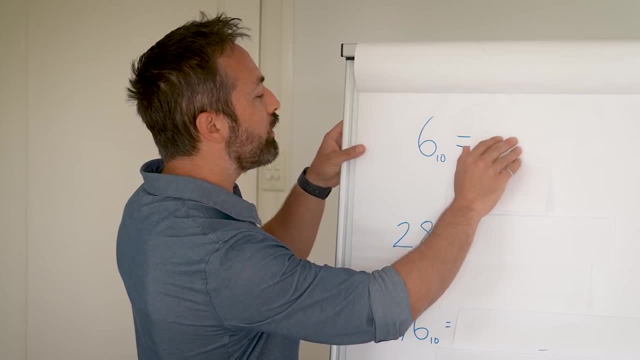 that we're going to be looking at today. We're going to be looking at a number that we're going to be looking at. that really blows my mind. If you write these numbers in binary, 6 becomes 1, 1, 0 and 28. 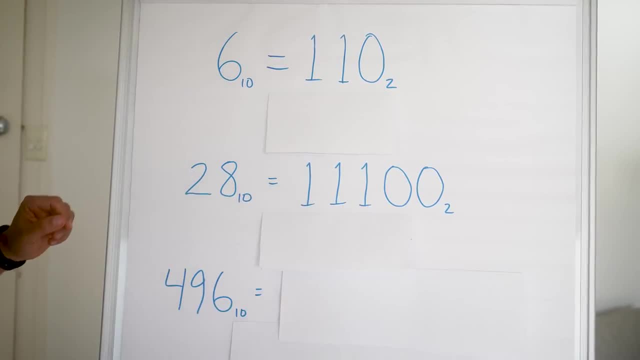 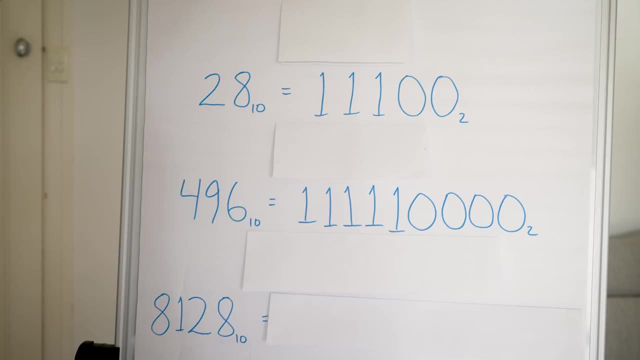 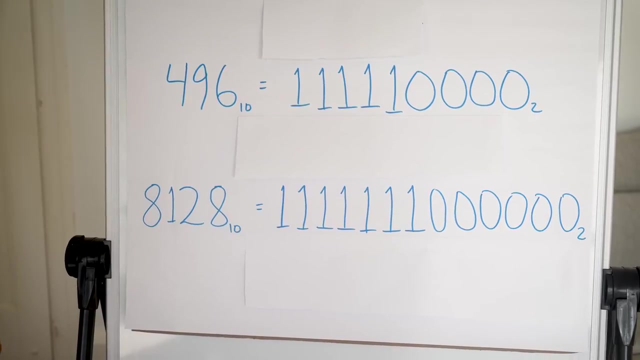 becomes 1 1 1 0, 0. 496 becomes 1 1 1, 1 1 0, 0 0, 0 and 8128, you guessed it. it is also a string of ones followed by a series of zeros, So if you write them out, they are: 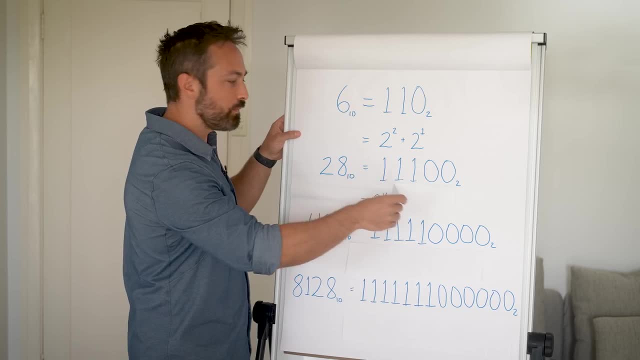 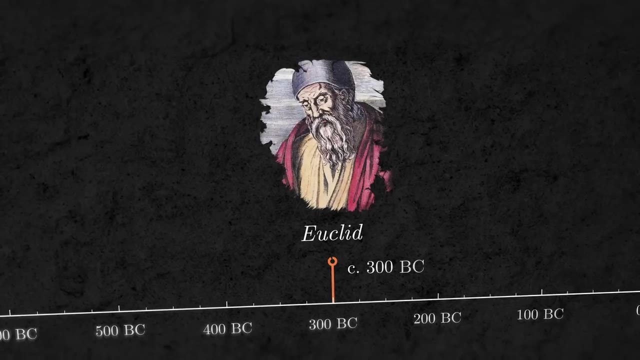 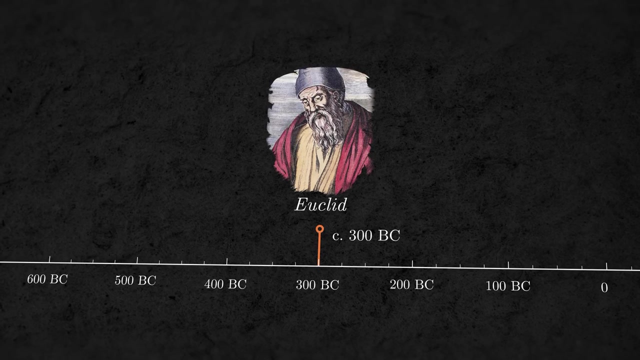 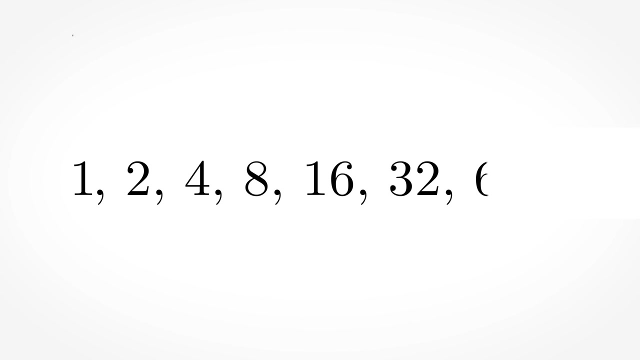 all just consecutive powers of two. Now, around 300 BC, Euclid was actually thinking along similar lines when he discovered the pattern that makes these perfect numbers. Take the number 1 and double it, You get 2,. now keep doubling it, You get 4,, 8,, 16,, 32,, 64 and so on. Now, starting from 1, add the next number. 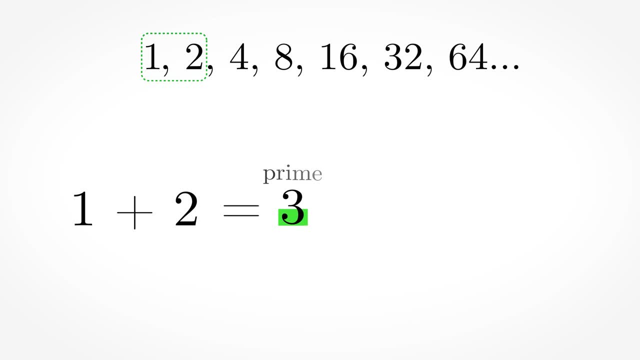 to it. So one plus two equals three. If that adds up to a prime, then you multiply it by the last number in the sequence to get a perfect number. so 2 times 3 equals 6, the first perfect number. Now let's keep doing this. Add 1 plus 2 plus 4 and you get 7, which is again prime. So multiply it. 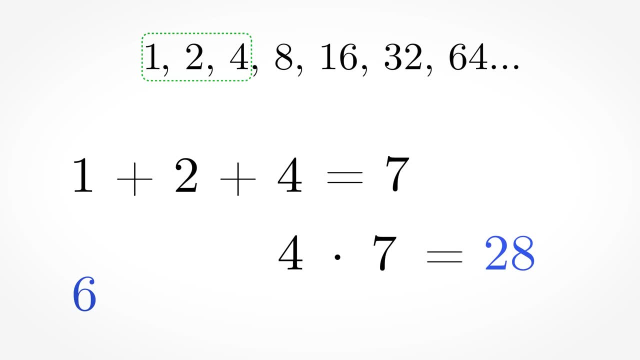 by the last number, 4, and you get 28…the next perfect number. Next, add 1 plus 2 plus 4 plus 8 equals 15.. But 15 isn't prime, so you come back to minus two and you solve for 15.. Remember that. 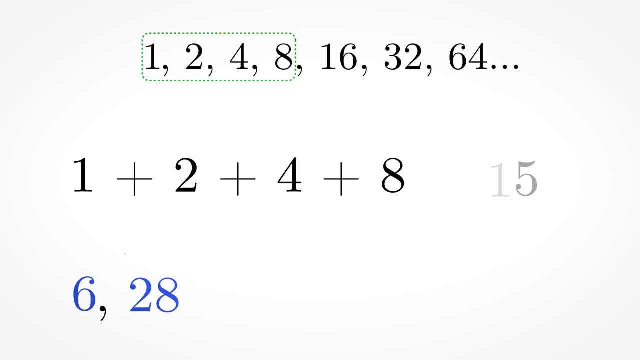 bless. seven equals six. Now that's kah- remain at that threshold. one plus two plus six equals eight, So that's tenth perfect number. Now the first ever perfect number somewhere is correct, assuming you're going. But 15 isn't prime, so we continue. 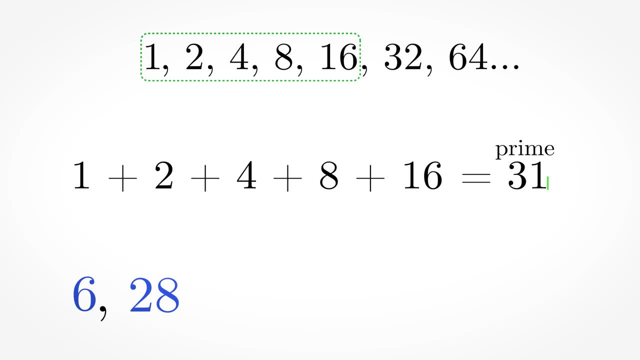 Add 16 to get 31.. This is prime. So you multiply it by 16 and you get 496, the third perfect number. Now you can keep doing this to find bigger and bigger perfect numbers And using this, we can rewrite the first three. 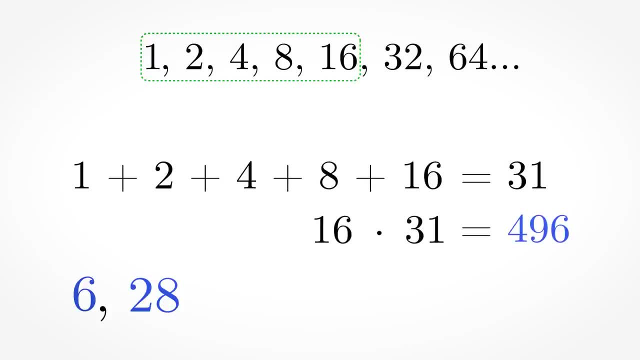 by sixteen and you get 496, the third perfect number. now you can keep doing this to find bigger and bigger perfect numbers and using this we can rewrite the first three. so six equals one plus two times two to the power of one, and 28 equals one plus two plus four times 2 squared. 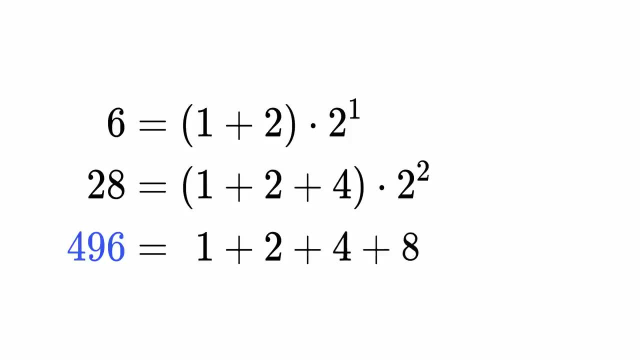 and 496 equals 1.. plus two plus four, plus eight, plus 16, times two to the power of four, where the first term is prime. But there's a more convenient way to write this. still, Take any sum of consecutive powers of two. 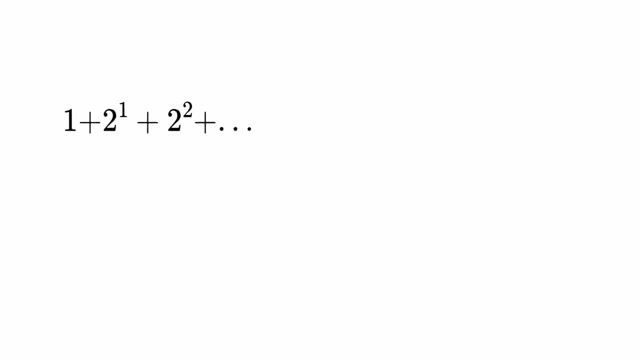 So two to the power of zero, which is one plus two to the one, plus two to the two, all the way up to two to the n minus one. And now, because you don't know n you don't know what that is equal to. 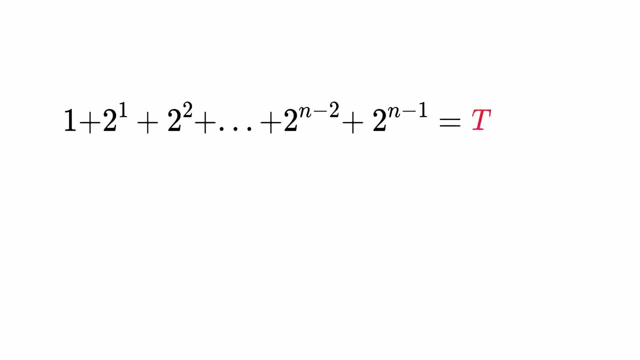 But it will be equal to something, so let's call that t. Now multiply this whole equation by two, So you get two to the one plus two to the two, all the way up to two to the n, and this is equal to two t. 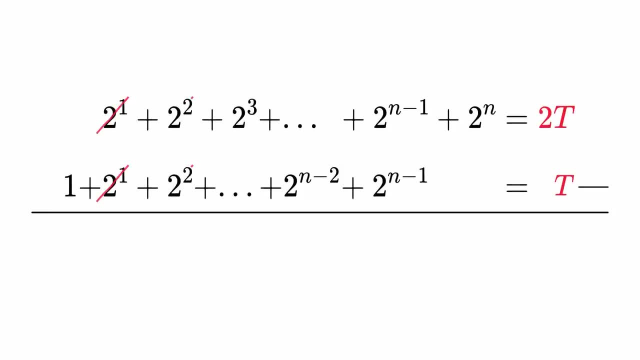 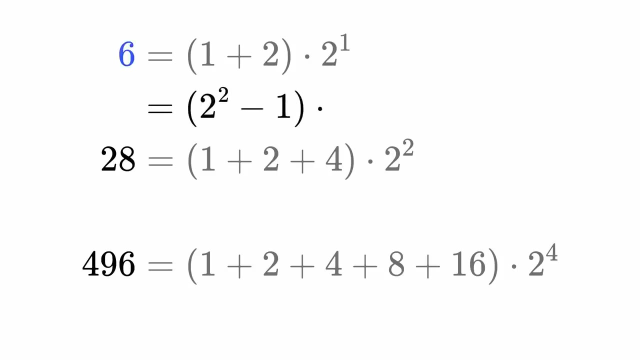 If you now subtract the first equation from the second, almost all the terms will cancel out and you're left with: t equals two to the n minus one. So you can replace this whole series with one less than the next power of two. So six becomes two squared minus one times two to the one. 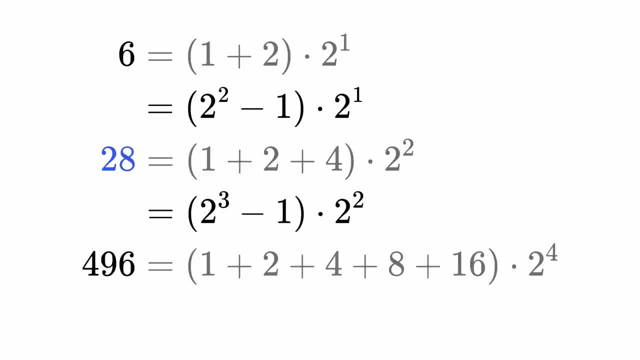 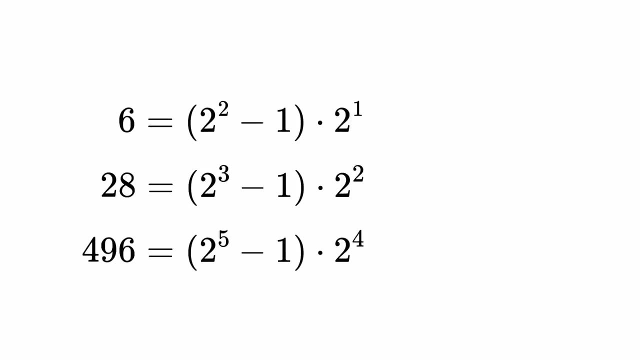 28 becomes two cubed minus one times two squared, And 490 squared minus one. and 26 becomes two to the five minus one times two to the four. Do you see the pattern? This number is always one more than this. 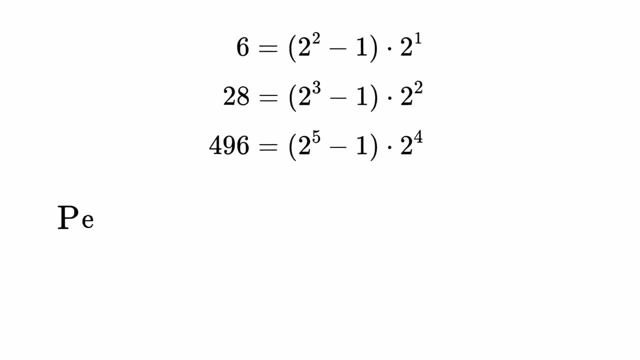 So if we call this p, then Euclid's formula that gives a perfect number is two to the p minus one times two to the p minus one, whenever this is prime. Now, because you're multiplying it by two to the p minus one. 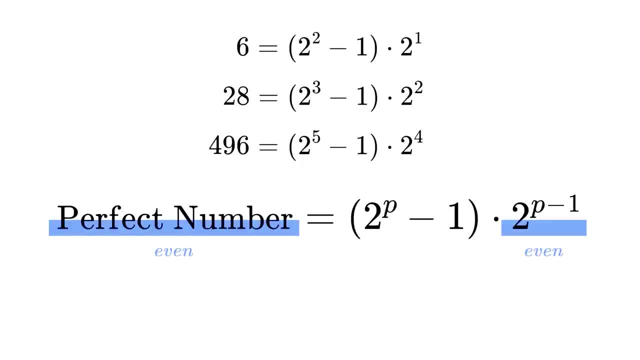 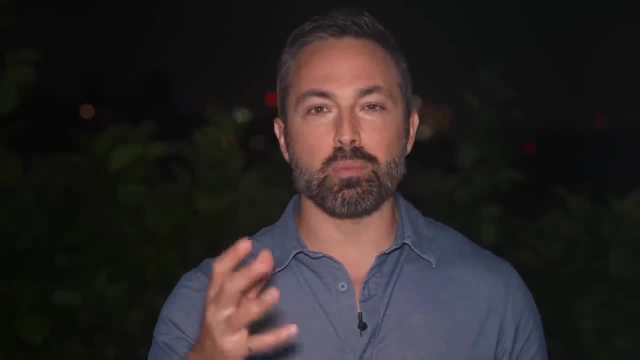 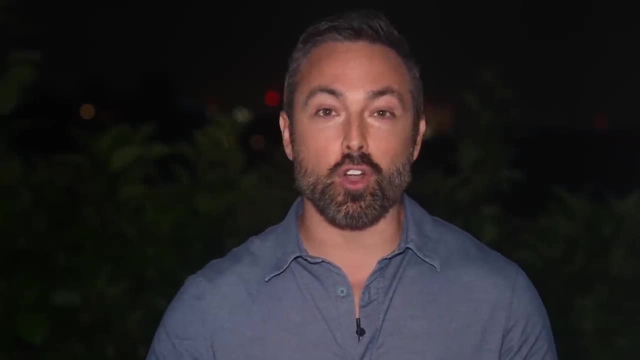 which is even. this will always give an even number. Euclid had found a way to generate even perfect numbers, but he didn't prove that this was the only way, So there could be other ways to get perfect numbers, including, potentially, ones that are odd. 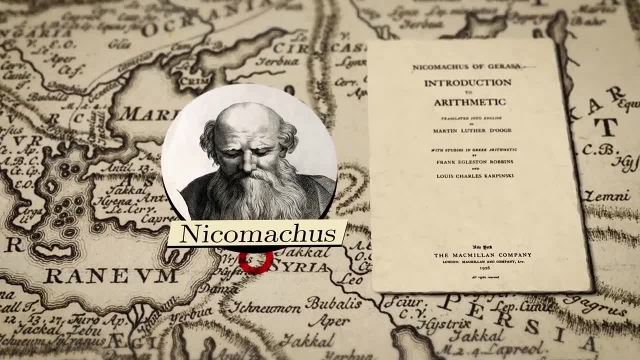 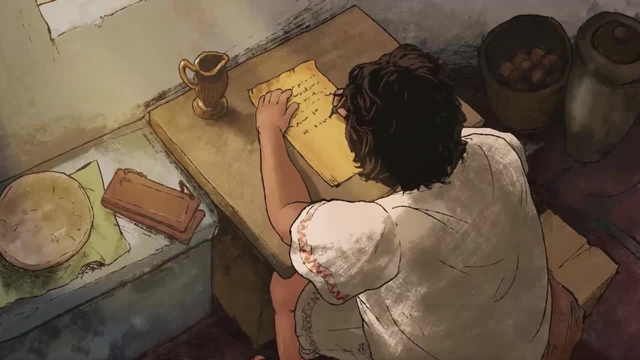 400 years later, the Greek philosopher Nicomachus published Introductio Arithmetica, the standard arithmetic text for the next thousand years. In it he stated five conjectures, statements he believed to be true but did not bother actually trying to prove. 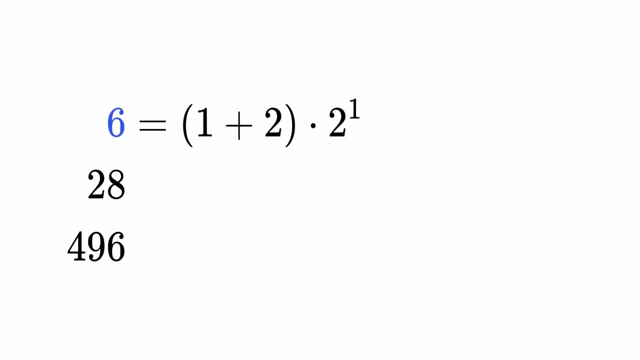 So six equals one plus two times two to the power of one, and 28 equals one plus two plus four times two. squared, and 496 equals one plus two plus four plus eight plus 16 times two to the power of four, where the first term is prime. 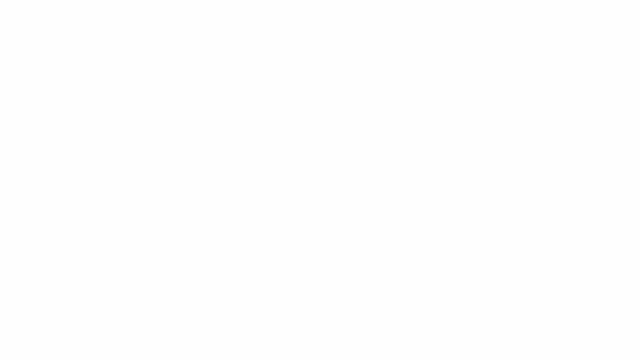 But there's a more convenient way to write this still, Take any sum of consecutive powers of two, So two to the power of zero, which is one plus two to the one plus two to the two, all the way up to two to the n minus one. 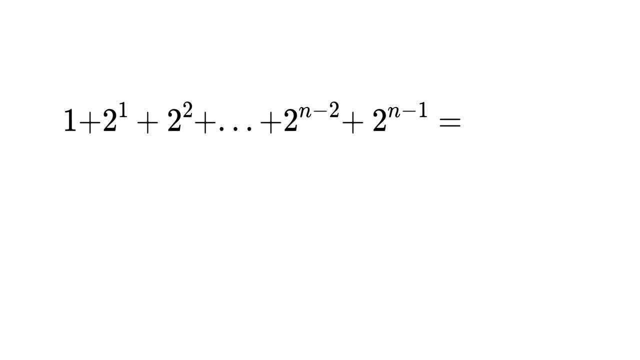 And now, because you don't know n, you don't know what that is equal to, but it will be equal to something, so let's call that t. Now multiply this whole equation by two, So you get two to the one plus two to the two. 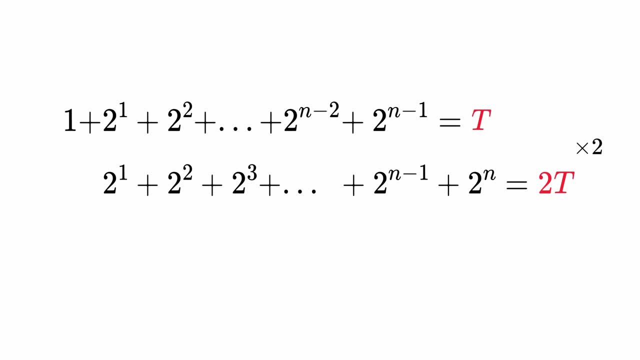 all the way up to two to the n, and this is equal to two t. If you now subtract the first equation from the second, almost all the terms will cancel out and you're left with: t equals two to the n minus one. 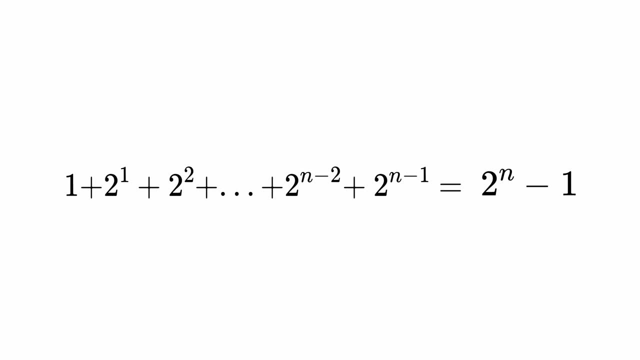 So you can replace this whole series with one less than the next power of two. So six becomes two squared minus one times two to the one. 28 becomes two cubed minus one minus one times two squared, and 496 becomes two to the five minus one. 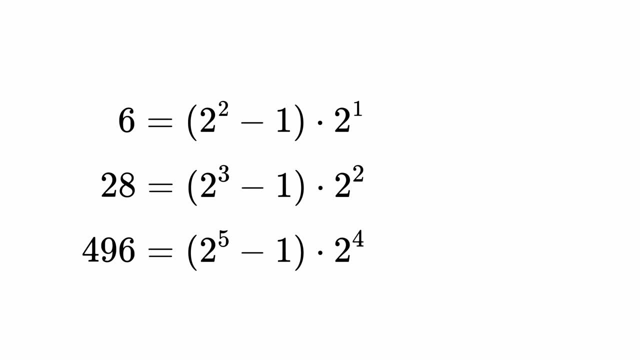 times two to the four. Do you see the pattern? This number is always one more than this. So if we call this p, then Euclid's formula that gives the perfect number is two to the p minus one times two to the p minus one. 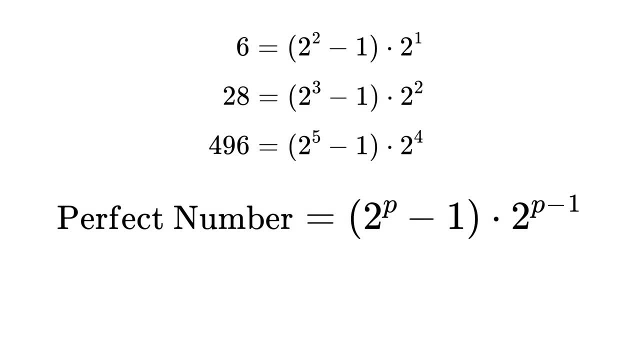 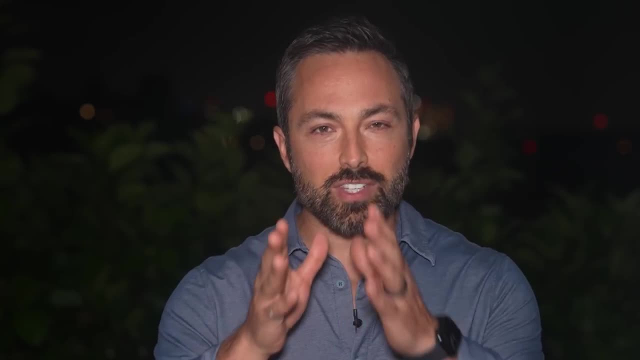 whenever this is prime Now, because you're multiplying it by two to the p minus one, which is even, this will always give an even number. Euclid had found a way to generate even perfect numbers, but he didn't prove that this was the only way. 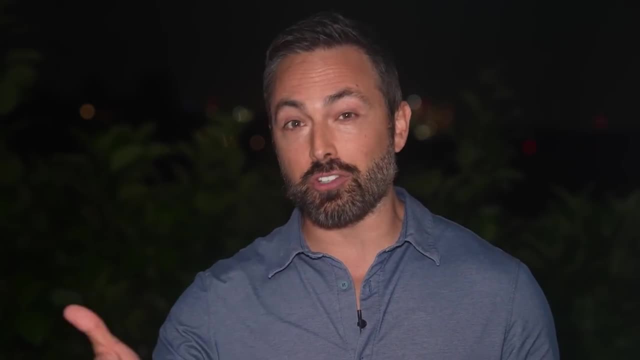 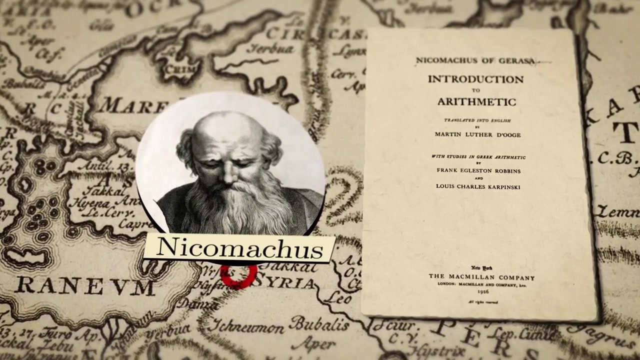 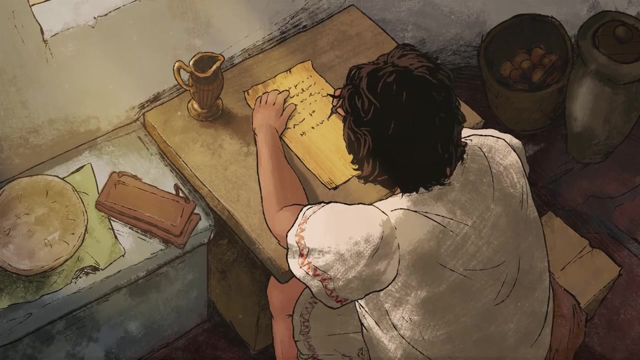 So there could be other ways to get perfect numbers, including potentially ones that are odd. 400 years later, the Greek philosopher Nicomachus published Introductio Arithmetica, the standard arithmetic text for the next thousand years. In it he stated five conjectures. 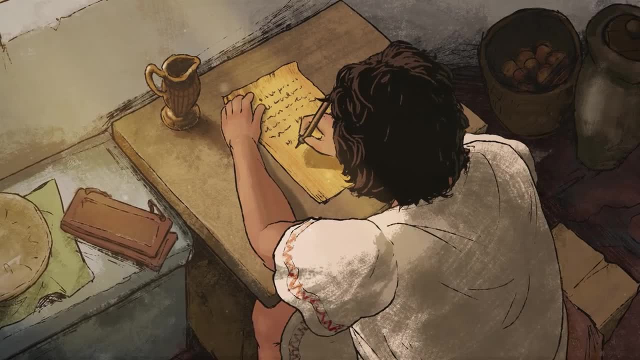 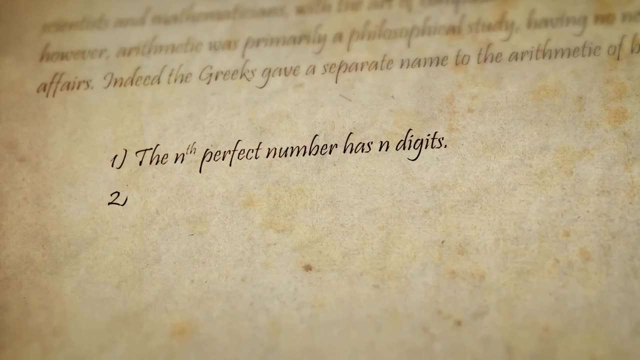 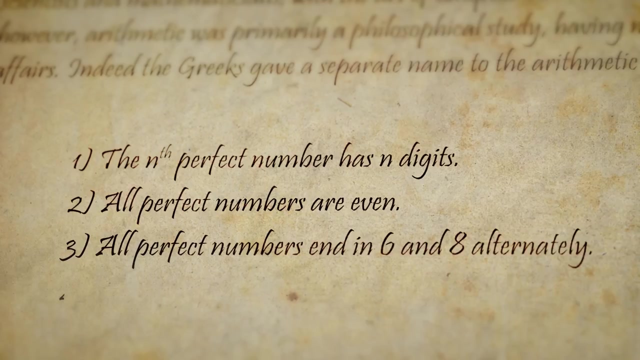 statements he believed to be true but did not bother actually trying to prove. His conjectures were: one: the nth perfect number has n digits. Two: all perfect numbers are even. Three: all perfect numbers end in six and eight alternately. 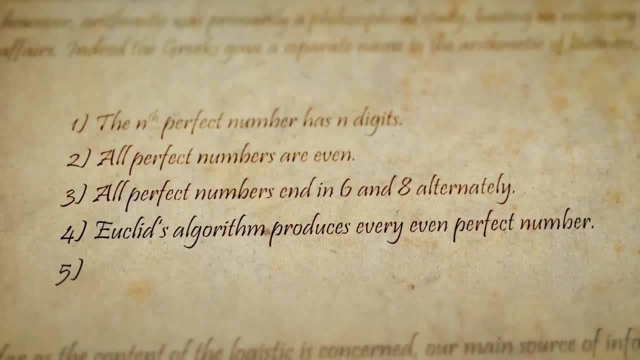 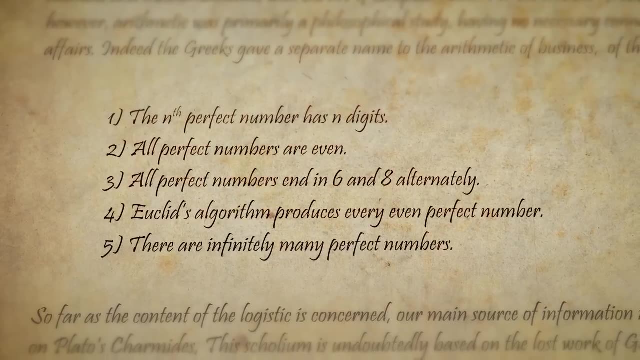 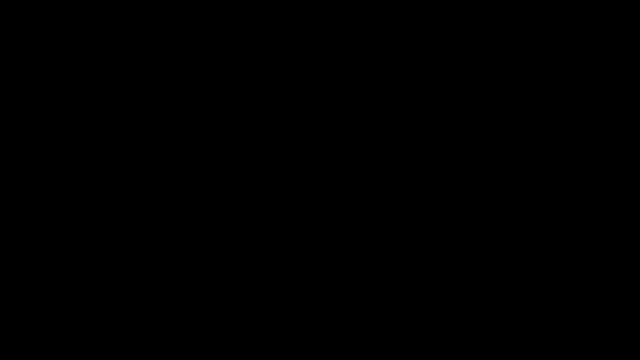 Four: Euclid's algorithm produces every even perfect number. And five: there are infinitely many perfect numbers For the next thousand years. no one could prove or disprove any of these conjectures And they were considered facts, But in the 13th century. 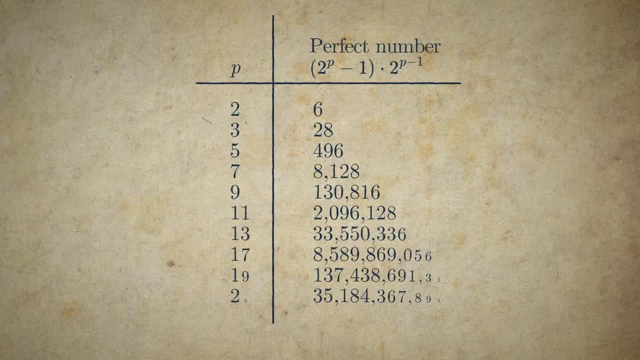 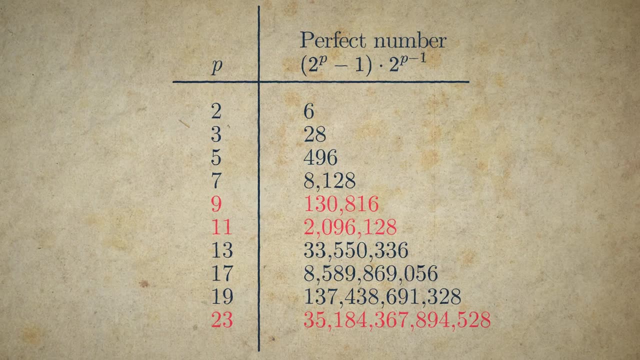 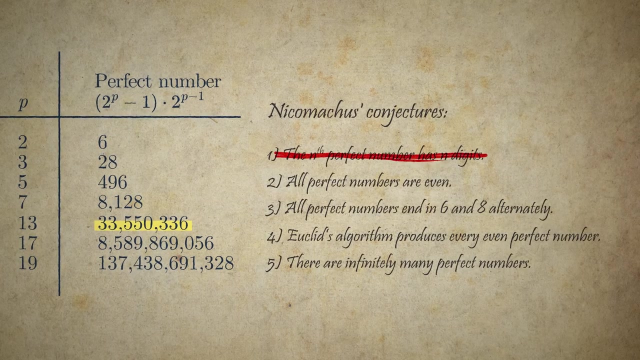 Egyptian mathematician Ibn Falas published a list with 10 perfect numbers and their values of p. Three of these perfect numbers turned out not to be perfect at all, but the remaining ones are. The fifth perfect number is eight digits long, which disproves Nicomachus' first conjecture. 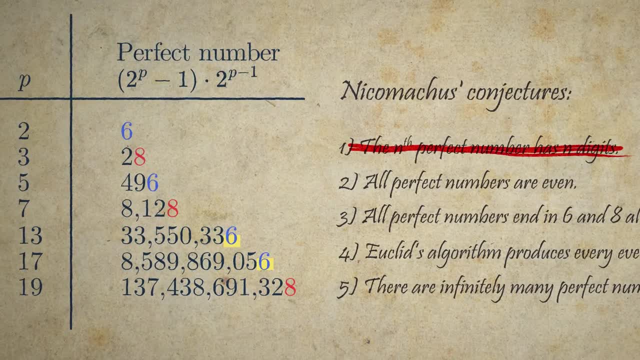 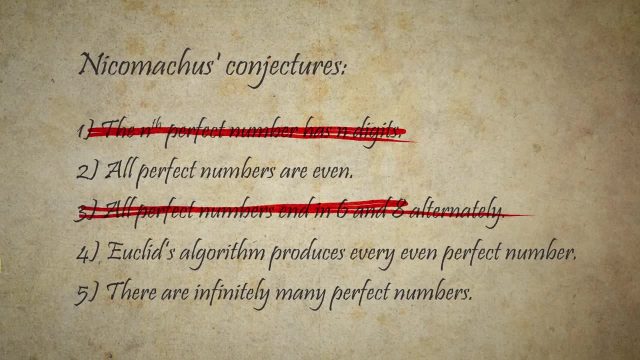 And the next thing to notice is that both the fifth and sixth perfect number end in a six. So that disproves Nicomachus' third conjecture: that all perfect numbers end in a 6 or 8 alternately. Two conjectures were proven false, but what about the other three? 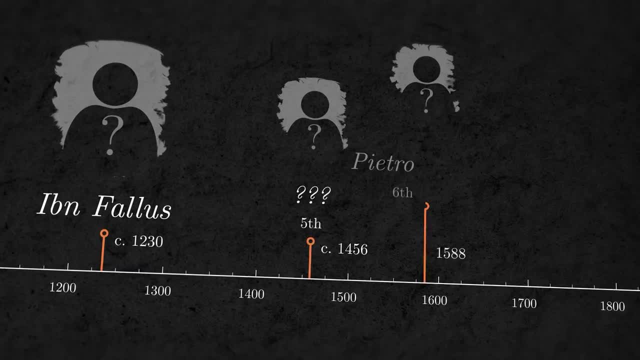 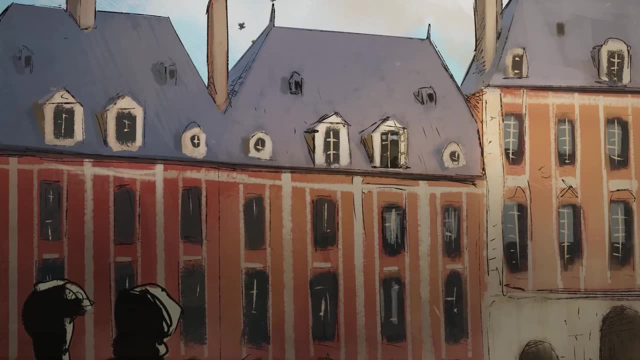 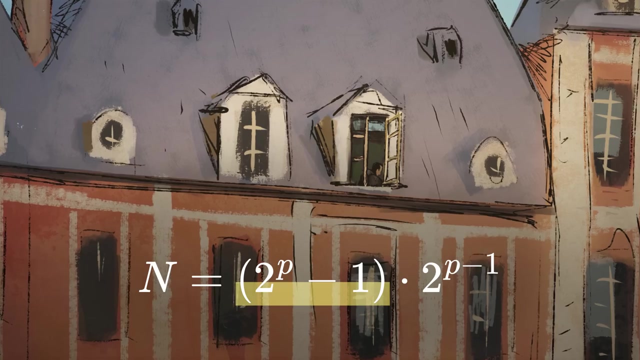 Two centuries later, the problem reached Renaissance Europe, where they rediscovered the 5th, 6th and 7th perfect numbers. So far, every perfect number had Euclid's form, And the best way to find new ones was by finding the values of p that make 2 to the p minus 1 prime. 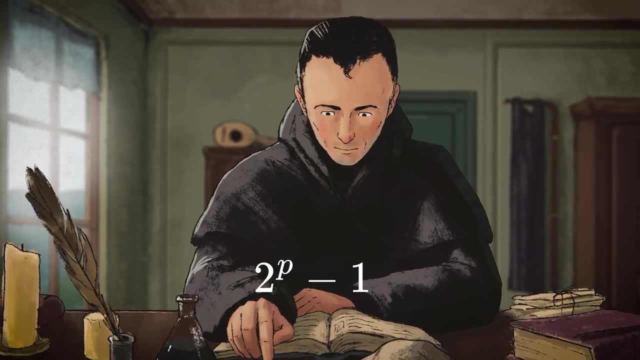 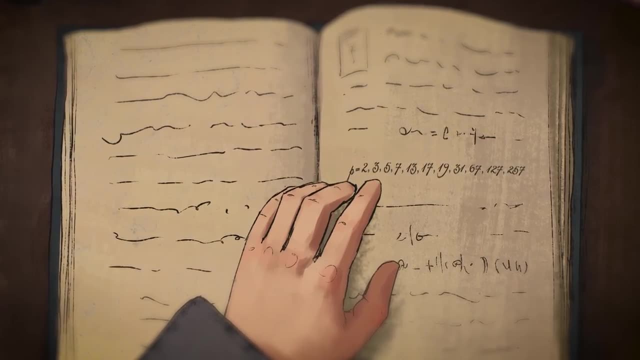 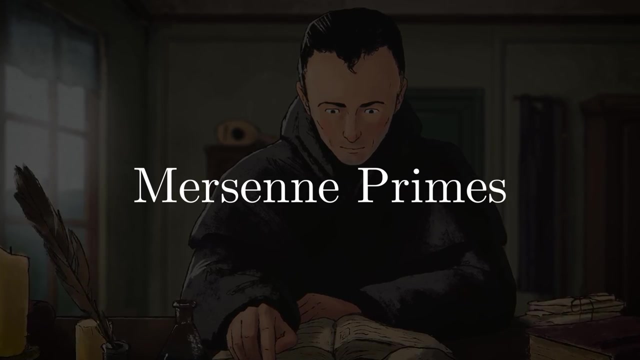 So French polymath Marin Mersenne extensively studied numbers of this form. In 1644, he published his results in a book including a list of 11 values of p for which he claimed they corresponded to primes. Numbers for which this is true are now called Mersenne primes. Of his list, the first 7 exponents of p do result in primes and they correspond to the first 7 perfect numbers. But for some of the larger numbers, like 2 to the 67 minus 1, Mersenne's first 7 exponents of p correspond to the first 7 perfect numbers. 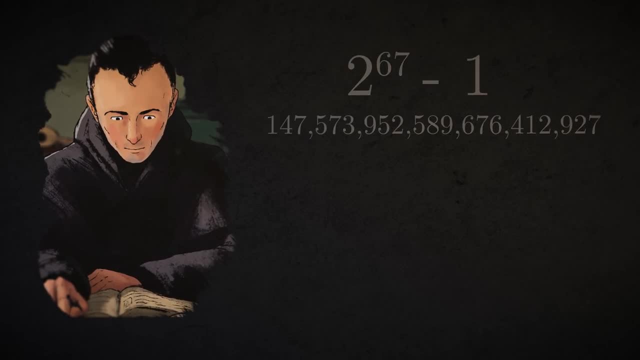 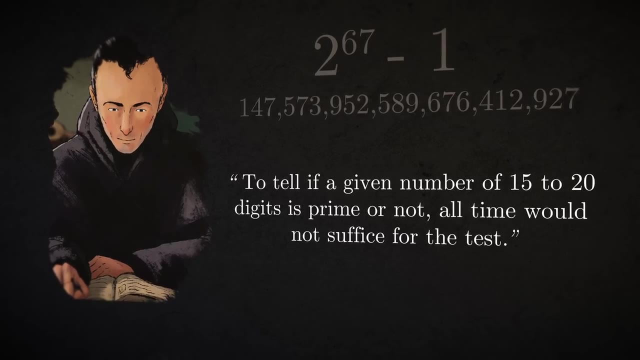 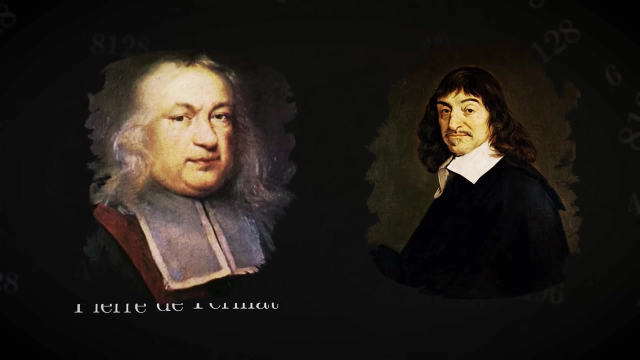 Mersenne admitted to not even checking whether they were prime. To tell if a given number of 15 to 20 digits is prime or not, all time would not suffice for the test. Mersenne discussed the problem of perfect numbers with other luminaries of the time, including Pierre de Fermat and René Descartes. 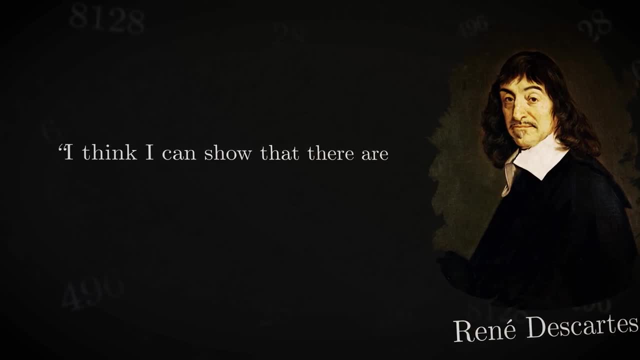 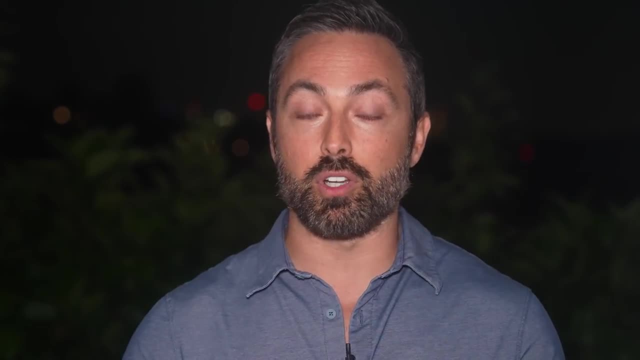 In 1638, Descartes wrote to Mersenne. I think I can show that there are no even perfect numbers except those of Euclid. He also believed that if an odd perfect number was prime, it would be prime. If an odd perfect number does exist, it must have a special form. 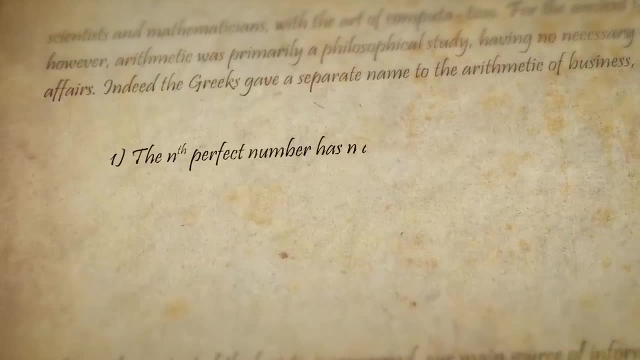 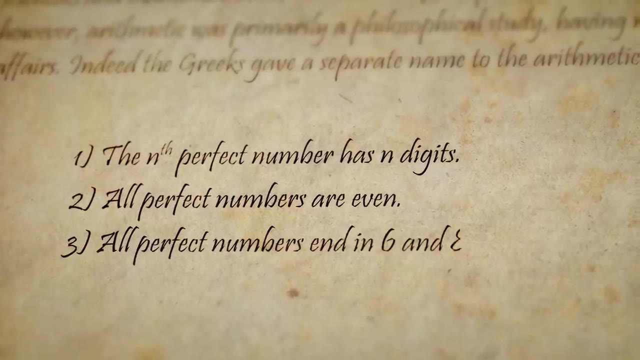 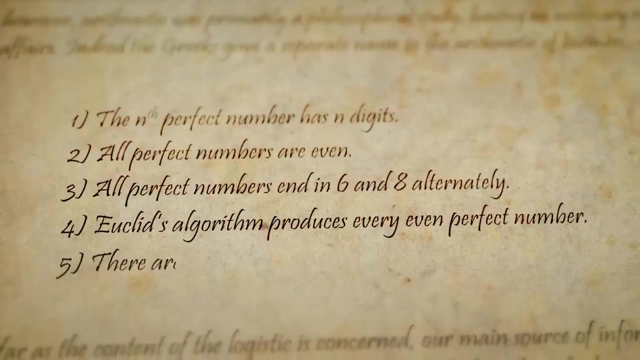 His conjectures were: one: the nth perfect number has n digits. Two: all perfect numbers are even. Three: all perfect numbers end in six and eight alternately. Four: Euclid's algorithm produces every even perfect number And five: there are infinitely many perfect numbers. 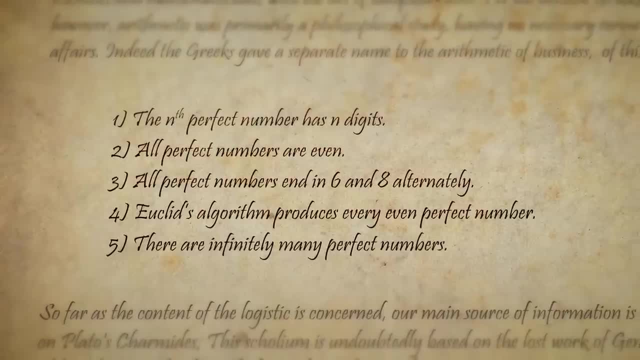 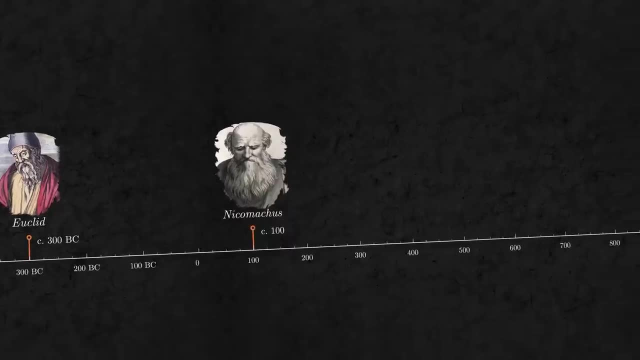 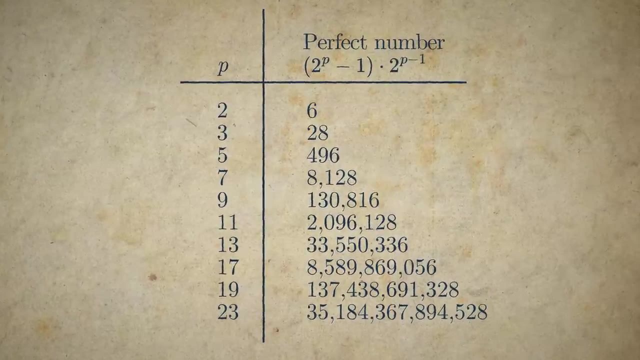 For the next thousand years. no one could prove or disprove any of these conjectures, and they were considered facts. But in the 13th century Egyptian mathematician Ibn Falis published a list with 10 perfect numbers and their values of p. 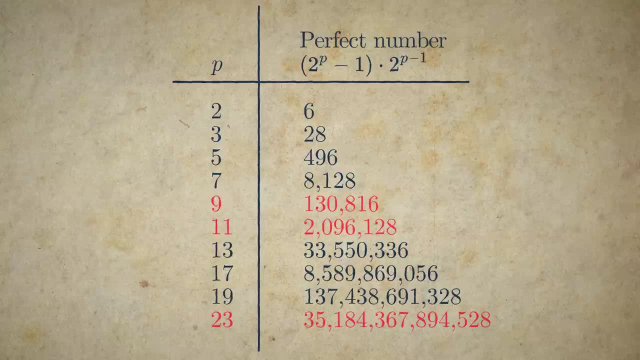 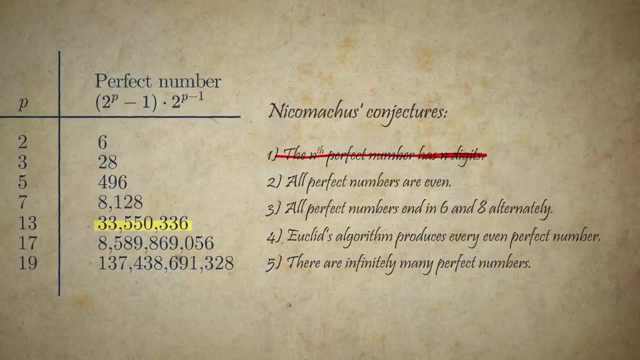 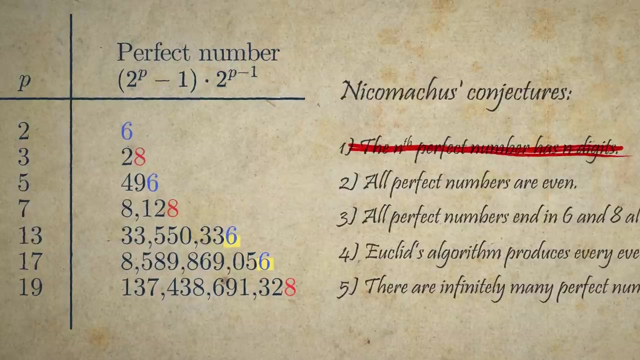 Three of these perfect numbers turned out not to be perfect at all, but the remaining ones are: The fifth perfect number is eight digits long, which disproves Nicomachus' first conjecture, And the next thing to notice is that both the fifth and sixth perfect number end in a six. 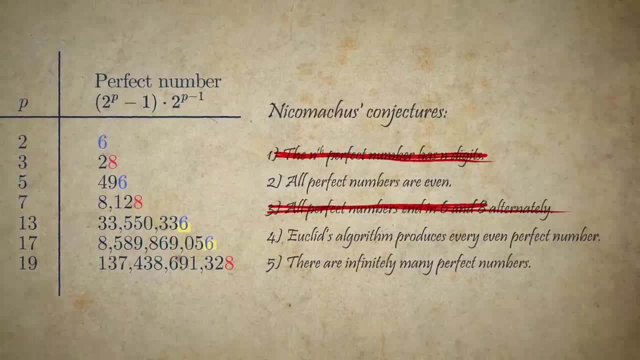 so that disproves Nicomachus' third conjecture: that all perfect numbers end in a six And that all perfect numbers end in a six or eight alternately. Two conjectures were proven false, but what about the other three? 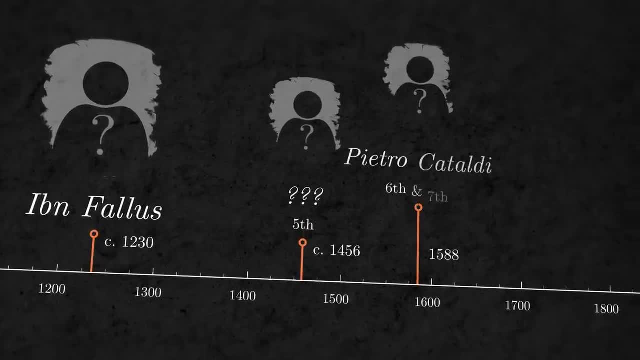 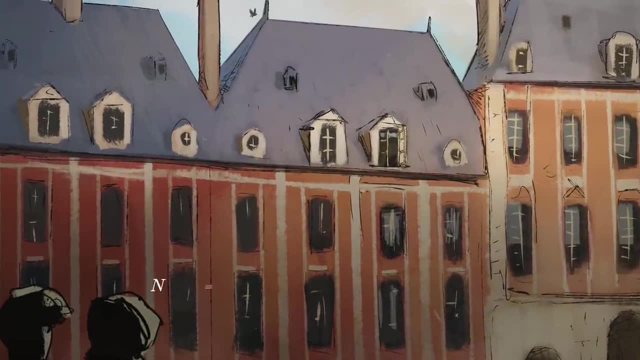 Two centuries later, the problem reached Renaissance Europe, where they rediscovered the fifth, sixth and seventh perfect numbers. So far, every perfect number had Euclid's form, And the best way to find new ones was by finding the values of p. 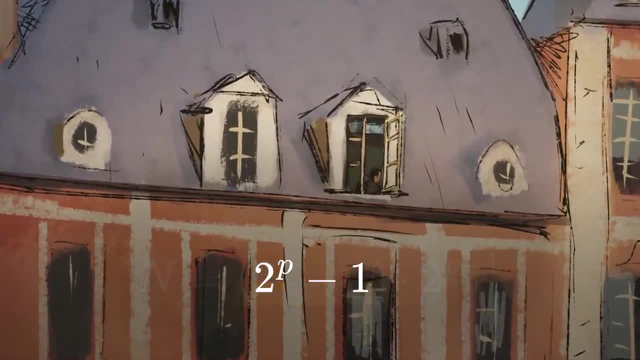 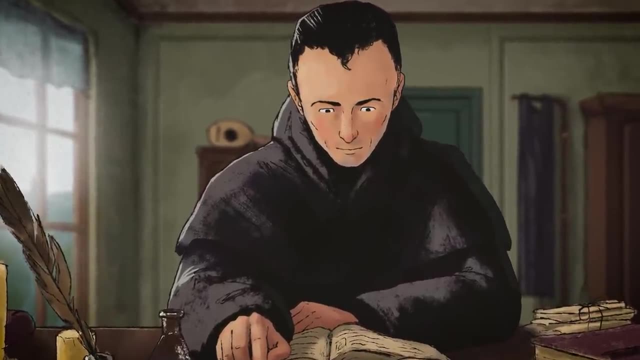 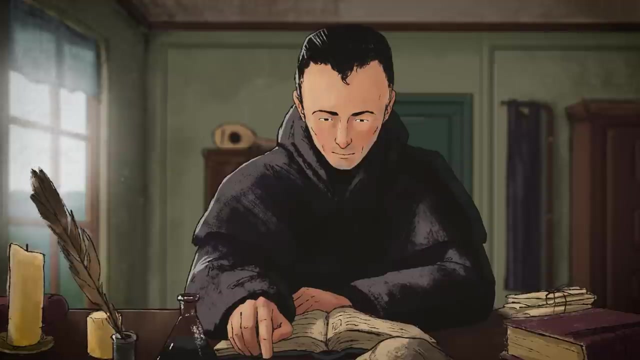 that make two to the p minus one prime. So French polymath Marin Mersenne extensively studied numbers of this form In 1644, he published his results in a book including a list of 11 values of p for which he claimed they corresponded to primes. 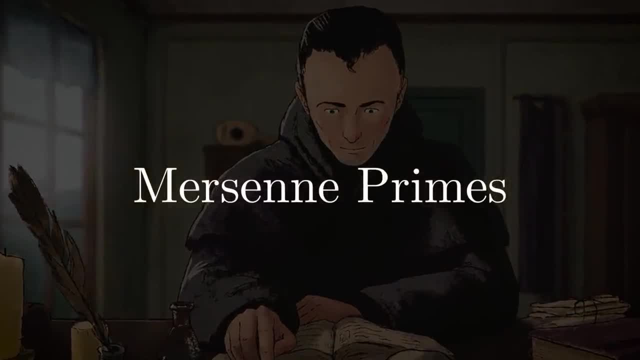 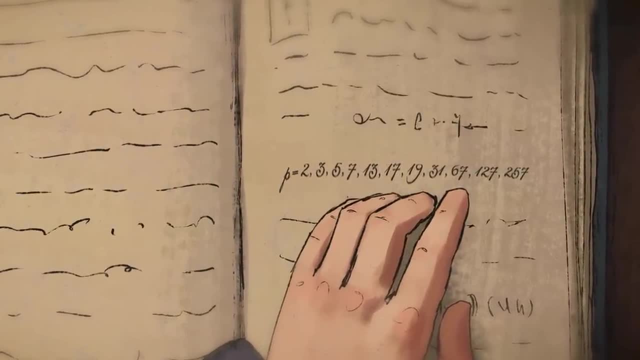 Numbers for which this is true are now called Mersenne primes Of his list. the first seven exponents of p do result in primes and they correspond to the first seven perfect numbers, But for some of the larger numbers, like two to the 67 minus one, 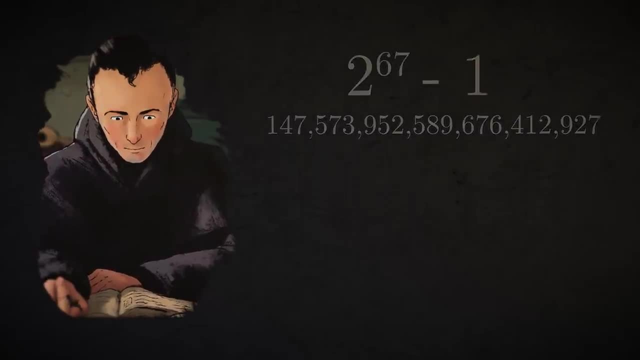 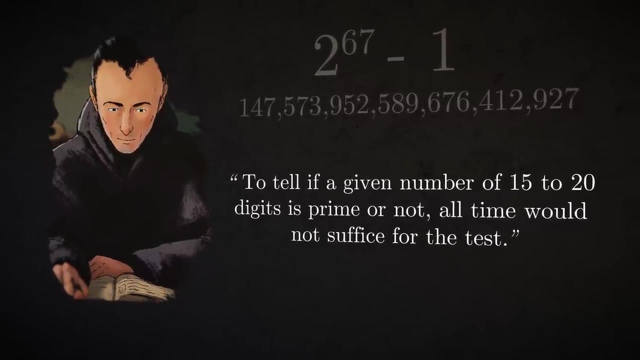 Mersenne admitted to not even checking whether they were prime. To tell if a given number of 15 to 20 digits is prime or not, all time would not suffice for the test. Mersenne discussed the problem of perfect numbers with other luminaries of the time. 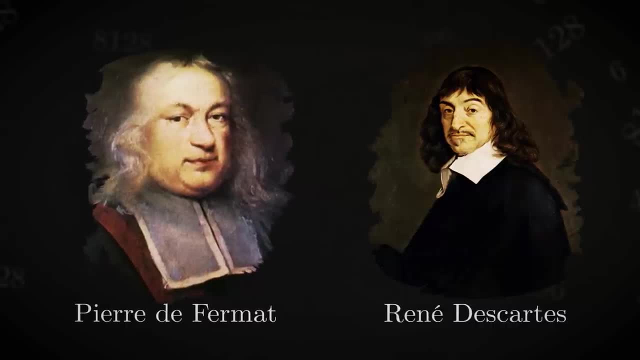 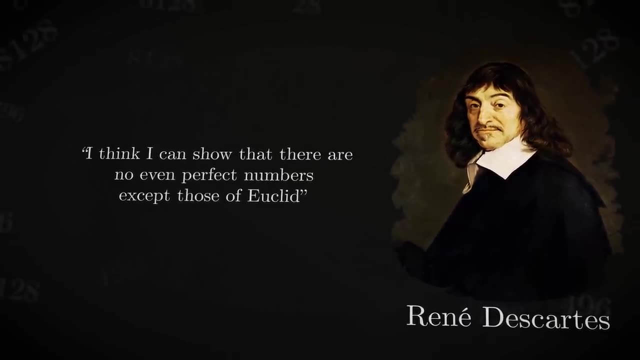 including Pierre de Fermat and René Descartes. In 1638, Descartes wrote to Mersenne. I think I can show that there are no even perfect numbers except those of Euclid. He also believed that if an odd perfect number does exist, 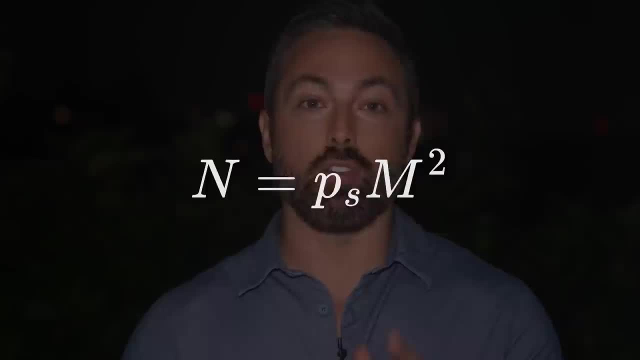 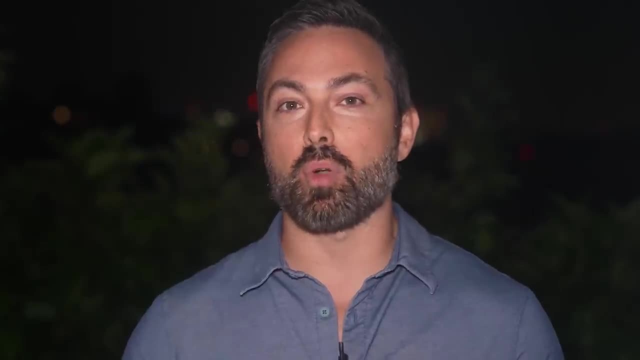 it must have a special form. It must be the product of a prime and the square of a different number. If he was right, these would easily have been the biggest breakthroughs on the problem since Euclid 2,000 years earlier. But Descartes couldn't prove either of those statements. 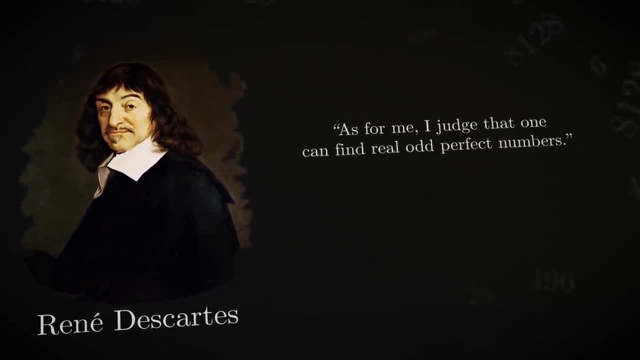 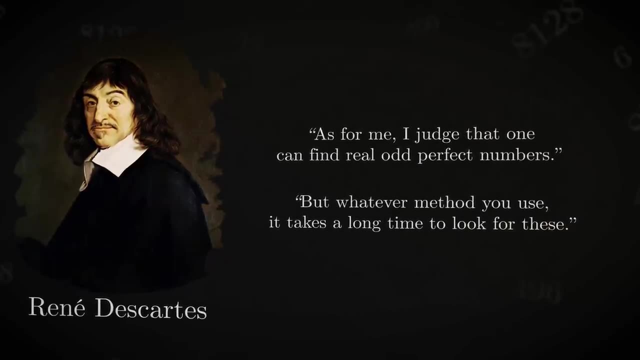 Instead he wrote: as for me, I judge that one can find real, odd, perfect numbers, but whatever method you use, it takes a long time to look for these Around. a hundred years later, at the St Petersburg Academy, the Prussian mathematician Christian Goldbach, 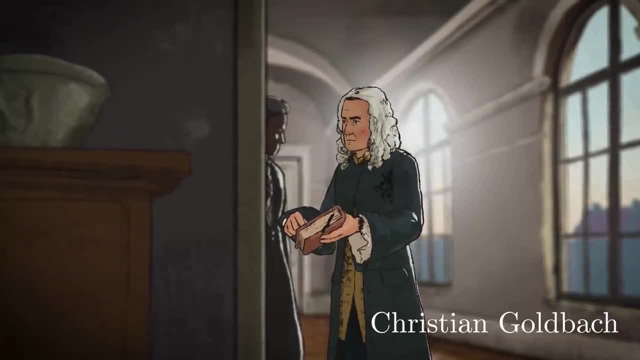 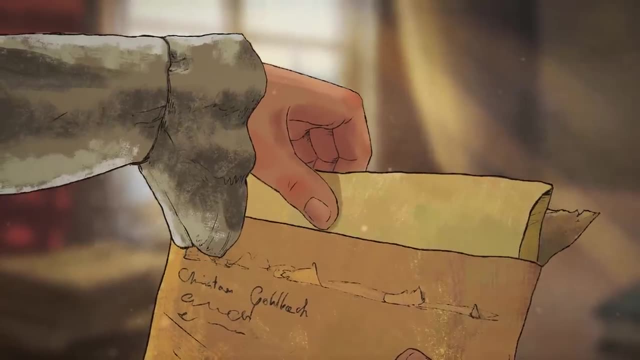 met a 20-year-old math prodigy. The two stayed in touch, corresponding by mail, And in 1729, Goldbach introduced this young man to the work of Fermat. At first he seemed indifferent, but after a little more prodding by Goldbach, he became passionate about number theory, and he spent the next 40 years working on different problems in the field. Among them was the problem of perfect numbers. This prodigy's name was Leonard Euler. Euler picked up where Descartes had left off. 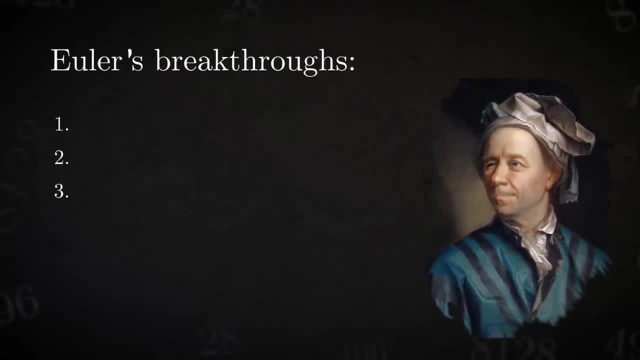 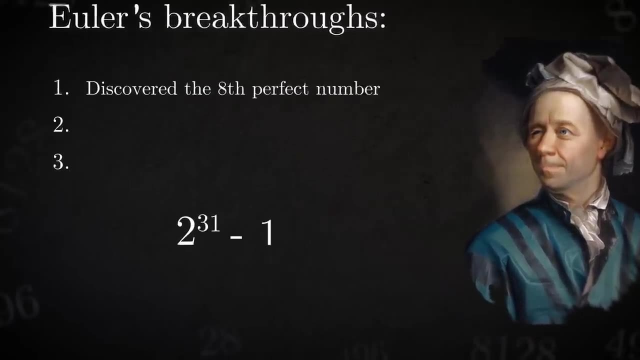 but with more success In doing so. he made three breakthroughs on this problem. First, in 1732, he discovered the eighth perfect number, which he had done by verifying that two to the 31 minus one is prime, just as Mersenne had predicted. 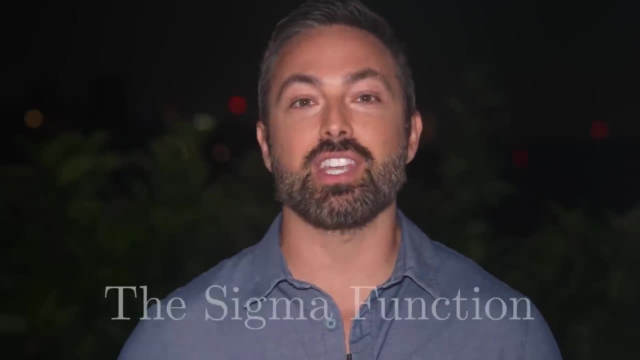 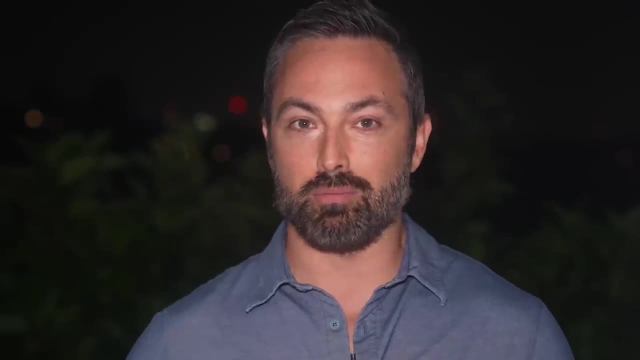 For his other two breakthroughs, he invented a new weapon, the sigma function. All this function does is it takes all the divisors of a number, including the number itself, and puts it in the middle, Including the number itself, and adds them up. 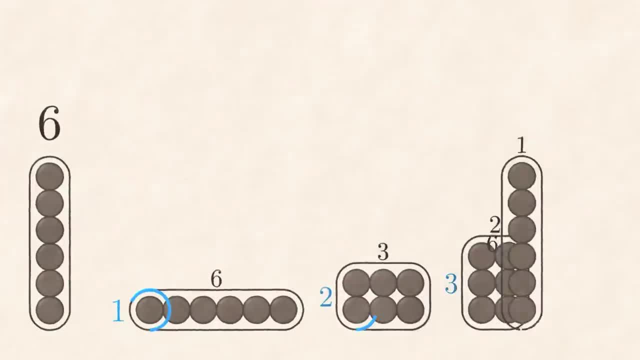 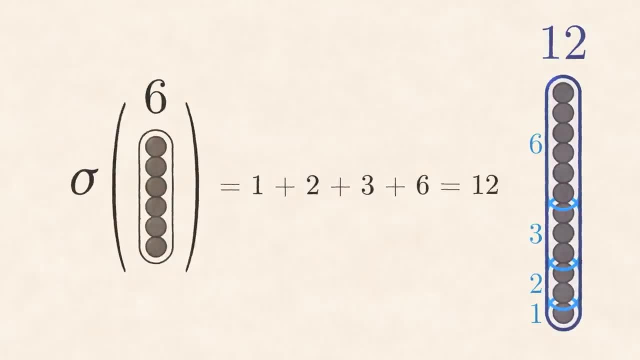 So take any number, say six, sum up all its divisors and you get 12, which is twice the number we started with. And this will be true for all perfect numbers. The sigma function of a perfect number will always give twice the number itself. 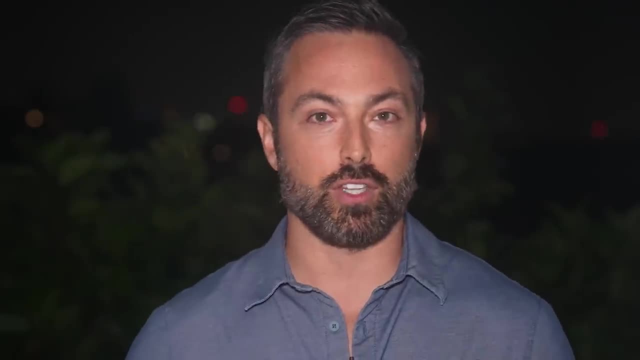 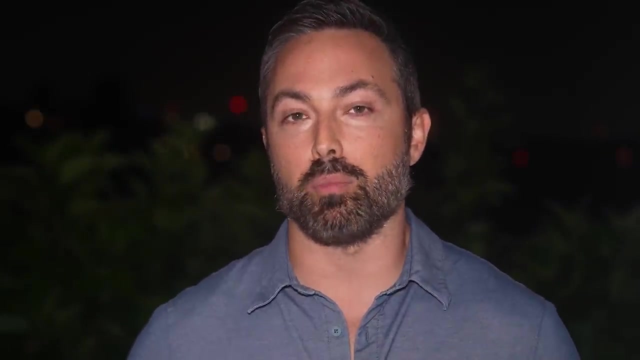 because the sigma function includes the number as one of its divisors. Now this may seem like a small change, but it ends up being extremely powerful. So let's look at a few examples. Take a prime number like seven Now, because it's prime. 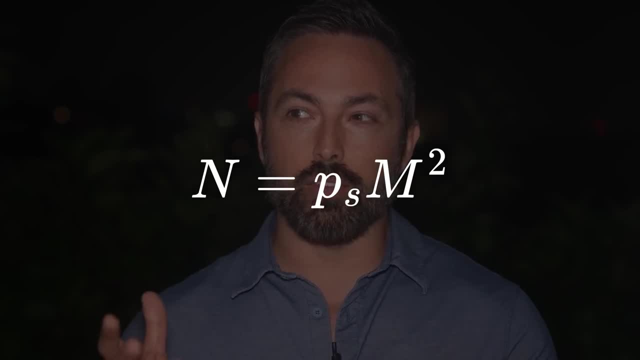 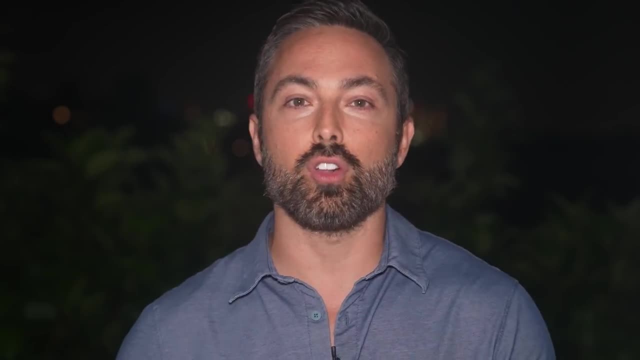 It must be the product of a prime and the square of a different number. If he was right, these would easily have been the biggest breakthroughs on the problem since Euclid 2,000 years earlier. But Descartes couldn't prove either of those statements. Instead he wrote. As for me, I judge that one can find real odd, perfect numbers, But whatever method you use, it takes a long time to look for these. Around 100 years later, at the St Petersburg Academy, the Prussian mathematician Christian Goldbach met a 20-year-old math prodigy. 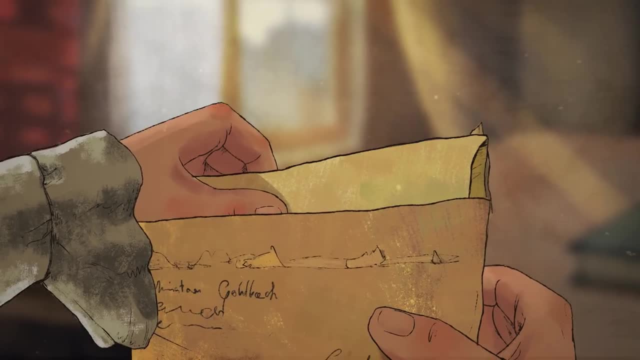 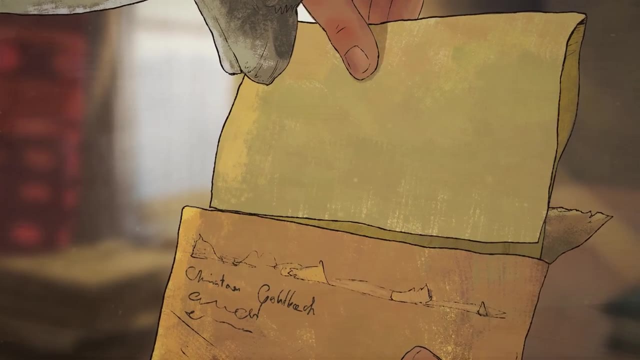 The two stayed in touch, corresponding by mail, And in 1729, Goldbach introduced this young man to the work of Fermat. At first he seemed indifferent, But after a little more prodding by Goldbach he became passionate about number theory. 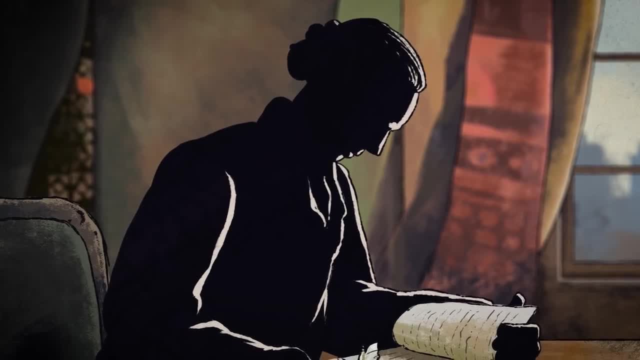 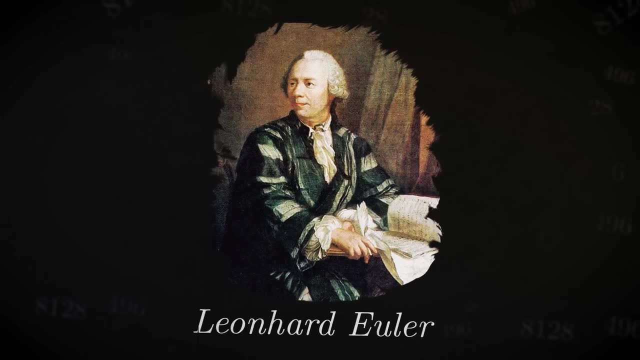 and he spent the next 40 years working on different problems in the field. Among them was the problem of perfect numbers. This prodigy's name, His name was Leonard Euler. Euler picked up where Descartes had left off, but with more success. 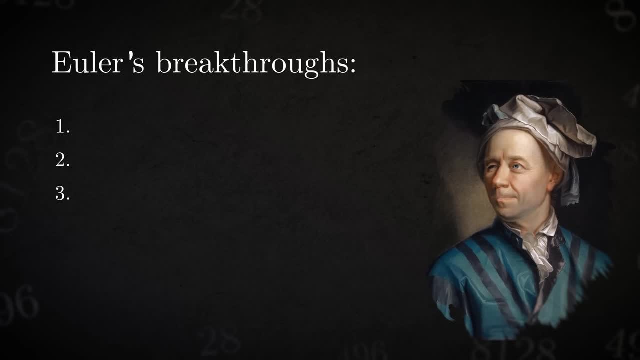 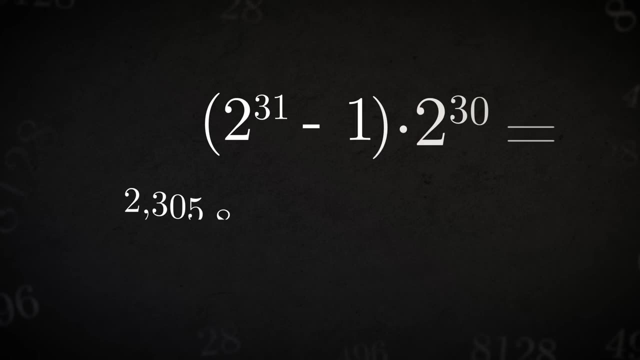 In doing so, he made three breakthroughs on this problem. First, in 1732, he discovered the eighth perfect number, which he had done by verifying that 2 to the 31 minus 1 is prime, just as Mersenne had predicted. 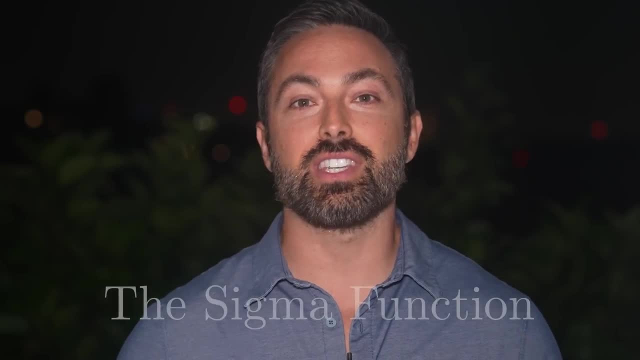 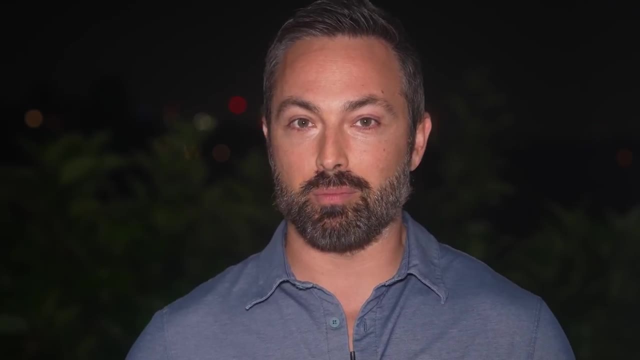 For his other two breakthroughs, he invented a new weapon, the sigma function. All this function does is it takes all the divisors of a number, including the number itself, and adds them up. So take any number, say 6, sum up all its divisors and you get 12,. 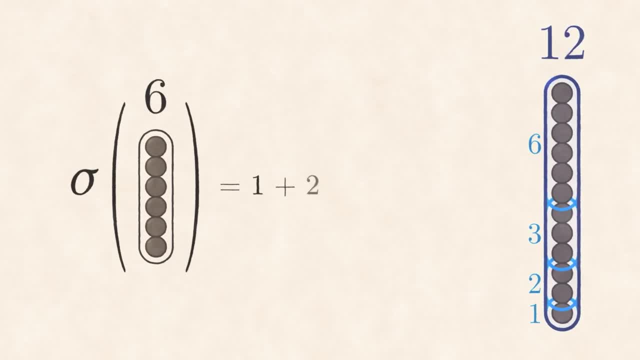 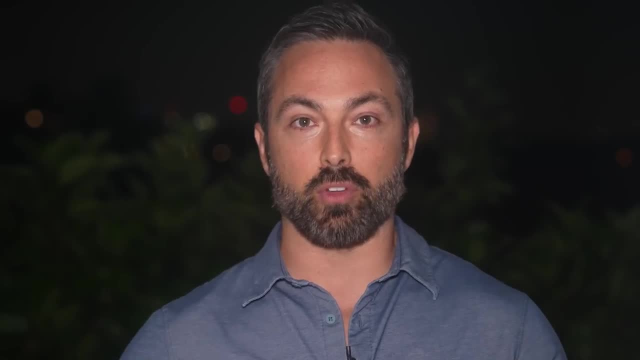 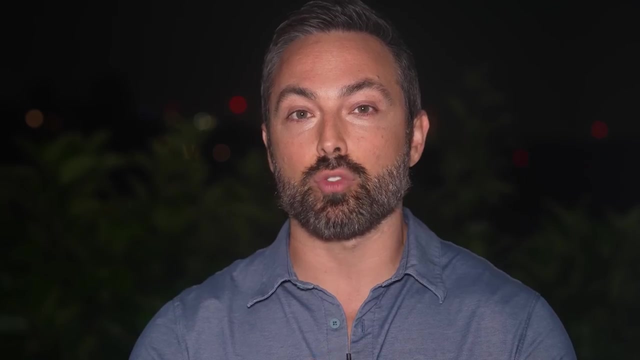 which is twice the number we started with, And this will be true for all perfect numbers. The sigma function of a perfect number will always give twice the number itself, because the sigma function includes the number as one of its divisors. Now this may seem like a small change, but it ends up being extremely powerful. 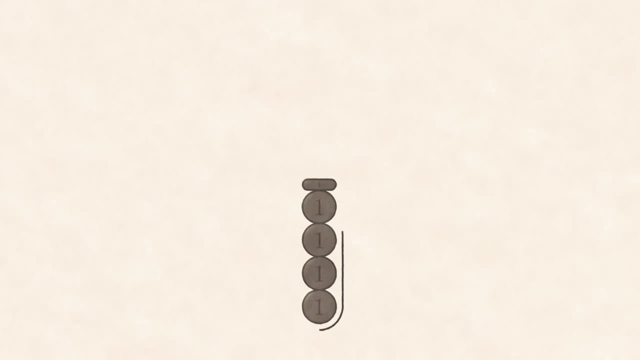 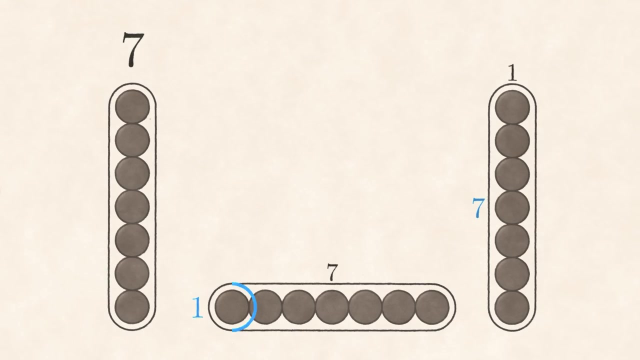 So let's look at a few examples. Take a prime number like 7.. Now, because it's prime, you can't rearrange it into a rectangle. Therefore, the only divisors are 1 and the prime itself. So sigma 7 is 1 plus 7, which is equal to 8.. 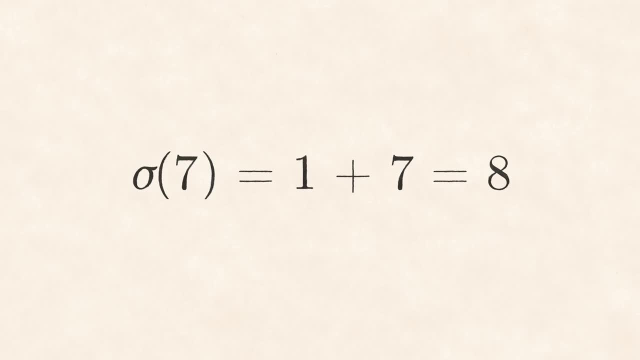 Now, to keep things easier to follow, we'll just stick to the numbers. But what if, instead of 7, you had 7 cubed? Well, again, the sum of the divisors is really simple. It's just 1 plus 7 plus 7 squared plus 7 cubed. 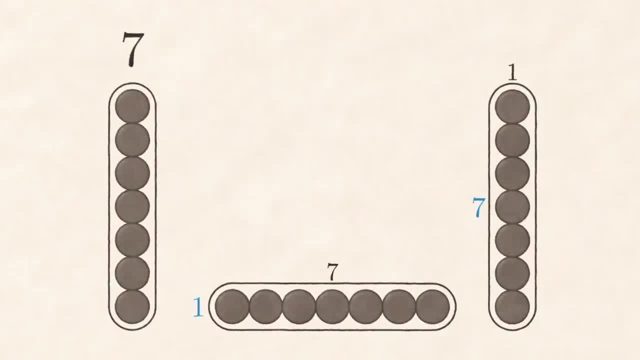 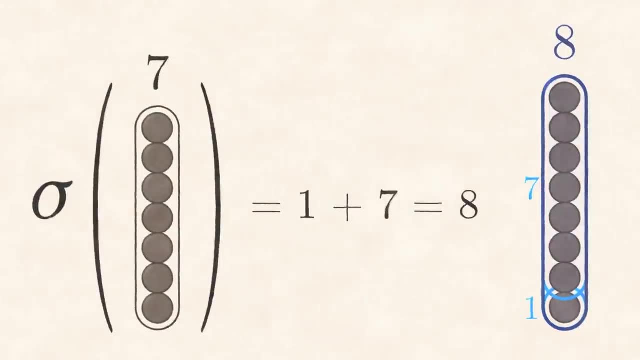 you can't rearrange it into a rectangle. Therefore, the only divisors are one and the prime itself. So sigma seven is one plus seven, which is equal to eight. Now, to keep things easier to follow, we'll just stick to the numbers. 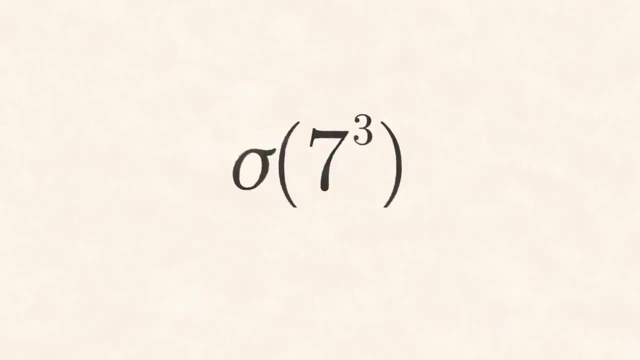 But what if, instead of seven, you had seven cubed? Well again, the sum of the divisors is really simple. It's just one plus seven, plus seven squared, plus seven cubed. Now let's use it on a different number. 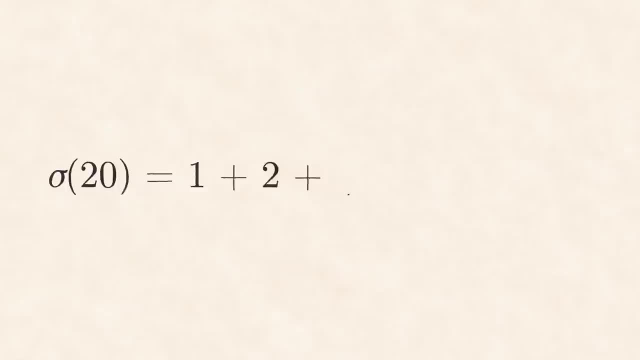 Say 20.. The sum of its divisors is one plus two plus four plus five plus 10 plus 20,, which equals 42. But you can also write this as one plus two plus four times one plus five, And this is what really makes the sigma function so powerful. 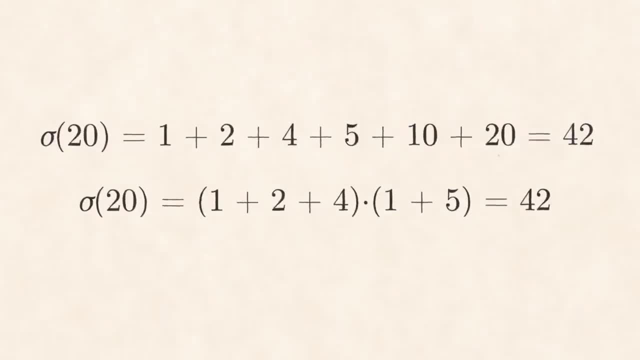 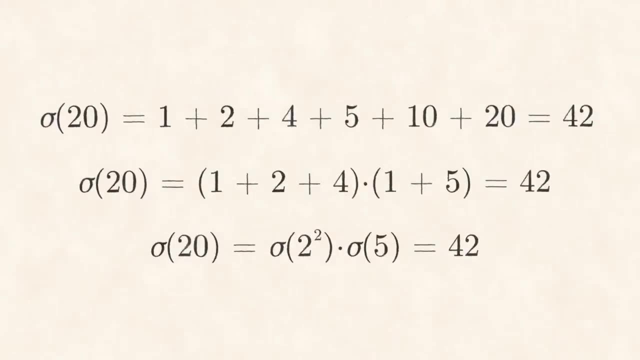 If you have a number that is made up of other numbers that don't share factors with each other, then you can split up the sigma function into the sigma functions of the prime powers that make it up. So sigma of two squared times sigma five is equal. 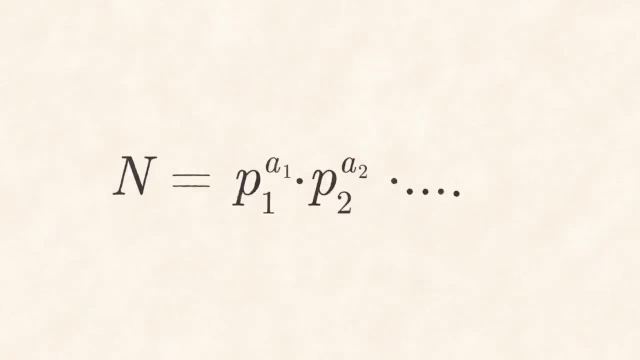 to sigma 20.. And since any number can be written as the product of prime powers, you can split up the sigma function of any composite number into the sigma functions of its prime powers. With his new function in hand, Euler achieved his second breakthrough. 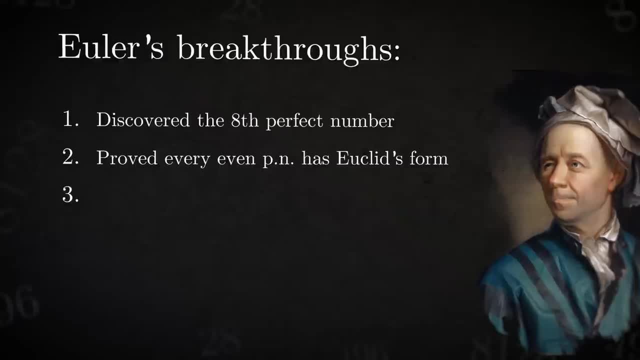 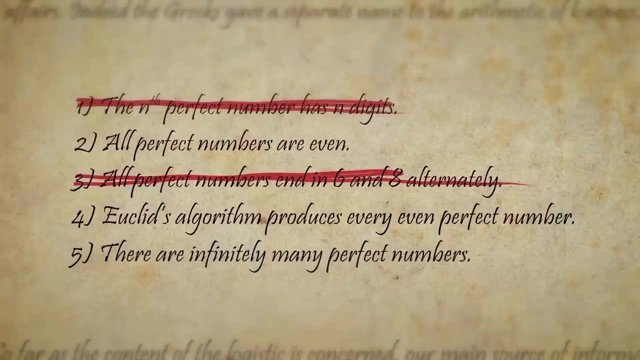 and did what Descartes couldn't: He proved that every, even perfect number has Euclid's form. This Euclid-Euler theorem solved a 1600-year-old problem and proved Nicomachus' fourth conjecture. Math historian William Dunham called it. 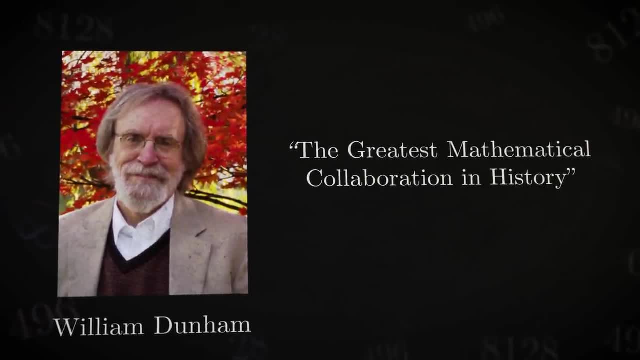 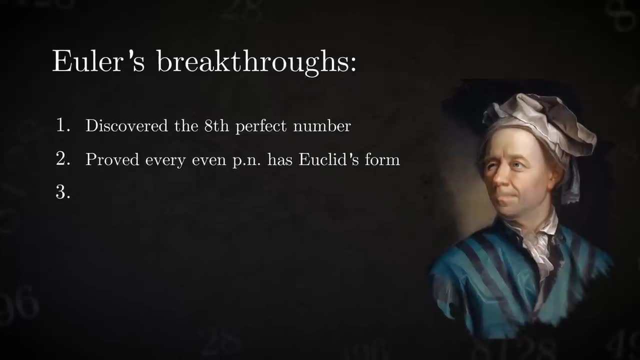 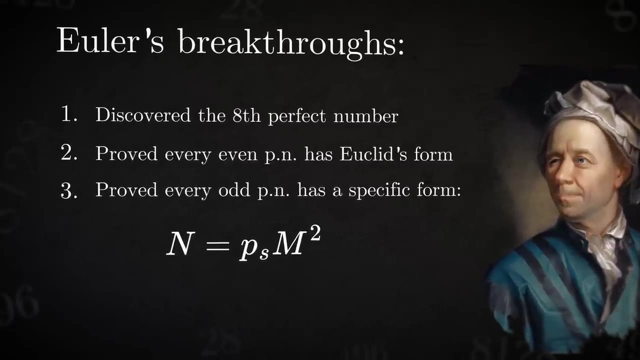 the greatest mathematical collaboration in history. But Euler wasn't finished yet. He also wanted to solve the problem of odd perfect numbers. So for his third breakthrough he set out to prove Descartes' other statement that every odd perfect number must have a specific form. 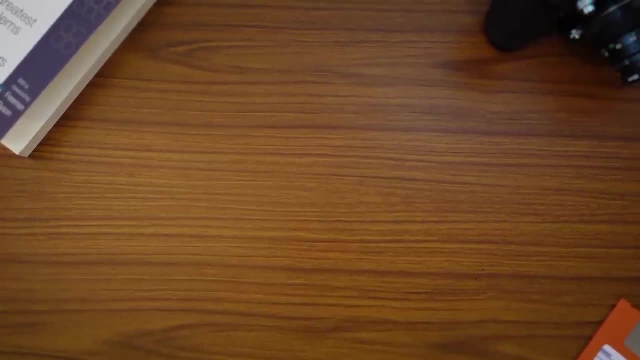 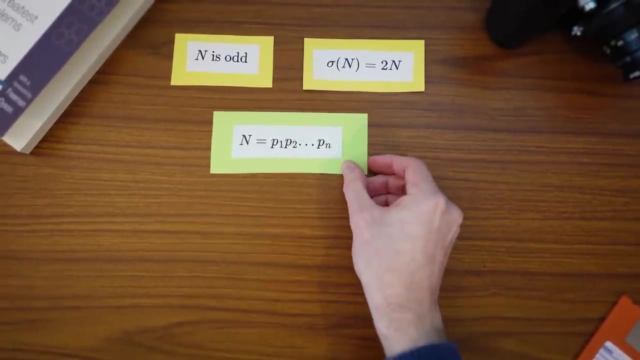 Because if an odd, perfect number does exist, you know two things: First, n is odd And second, sigma of n equals two n. Now, any number, n, you can write as a product of different prime numbers, and each prime can be to some power. 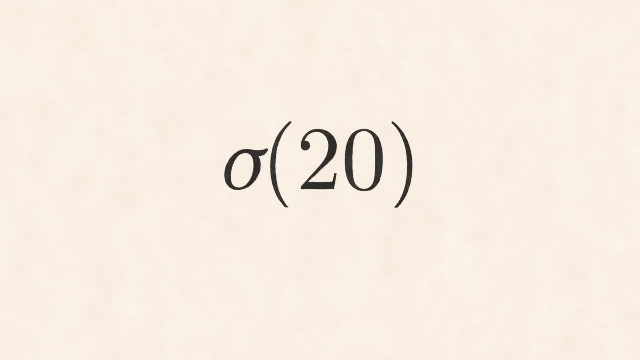 cubed. Now let's use it on a different number, say 20.. The sum of its divisors is 1 plus 2 plus 4 plus 5 plus 10 plus 20, which equals 42. But you can also write this as 1 plus 2 plus 4 times 1. 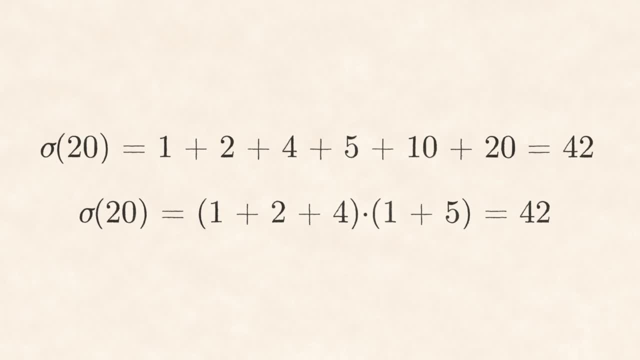 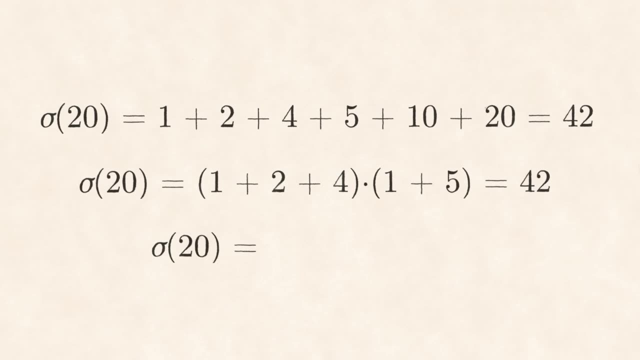 plus 5.. And this is what really makes the sigma function so powerful. If you have a number that is made up of other numbers that don't share factors with each other, then you can split up the sigma function into the sigma functions of the prime powers that make it up. So, sigma of 2: 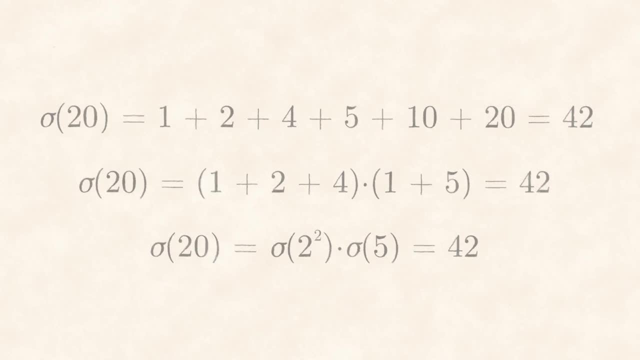 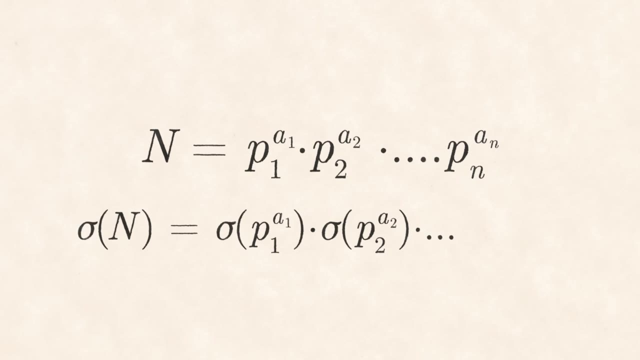 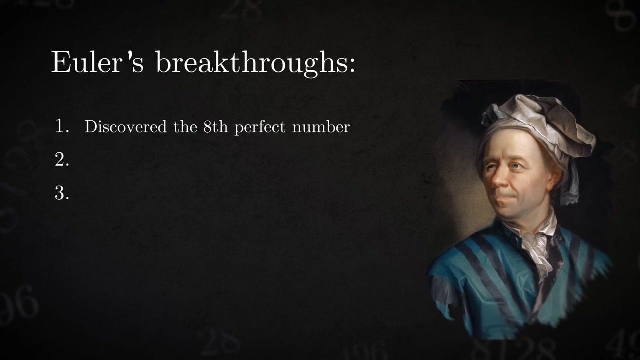 squared times, sigma 5 is equal to sigma 20.. And since any number can be written as the product of prime powers, you can split up the sigma function of any composite number into the sigma functions of its prime powers. With his new function in hand, Euler achieved his second. 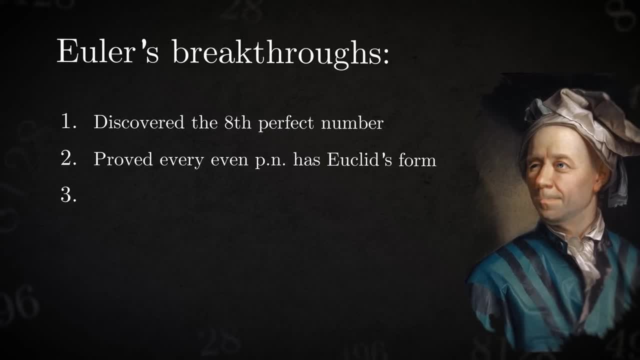 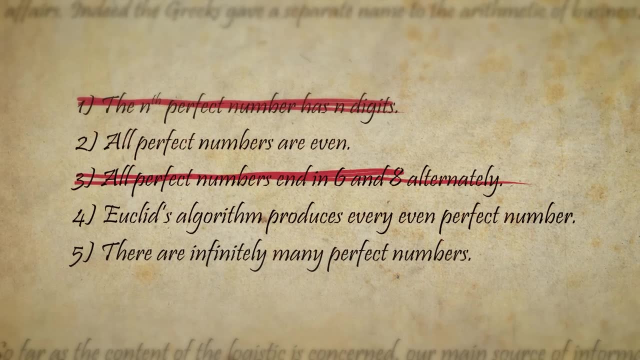 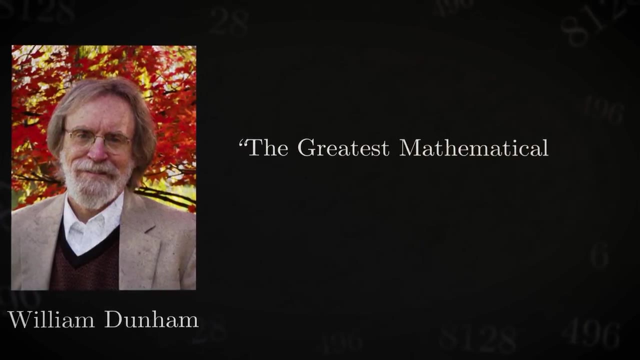 breakthrough and did what Descartes couldn't: He proved that every even perfect number has Euclid's form. This Euclid-Euler theorem solved a 1600-year-old problem and proved Nicomachus' fourth conjecture. Math historian William Dunham called it the greatest mathematical collaboration in history. 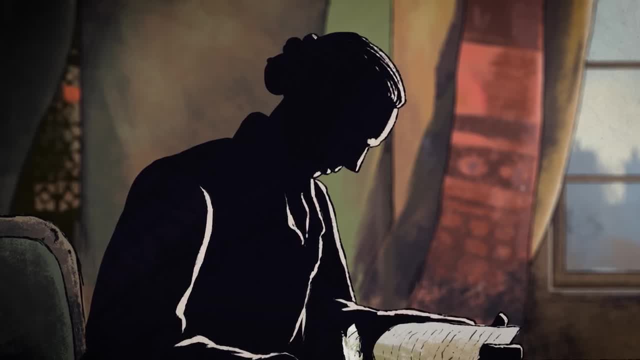 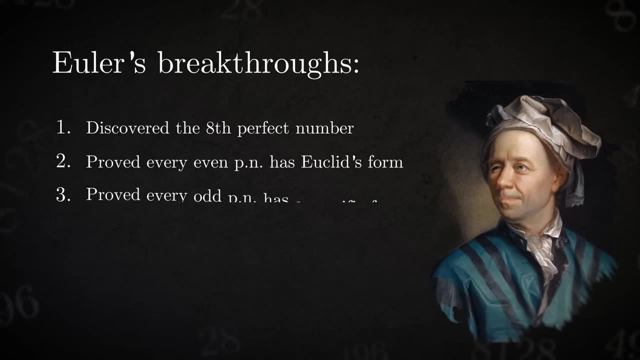 But Euler wasn't finished yet. He also wanted to solve the problem of odd perfect numbers. So for his third breakthrough he set out to prove Descartes' other statement that every odd perfect number must have a specific form, Because if an 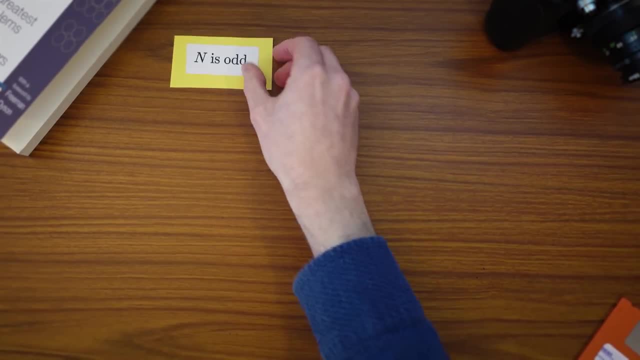 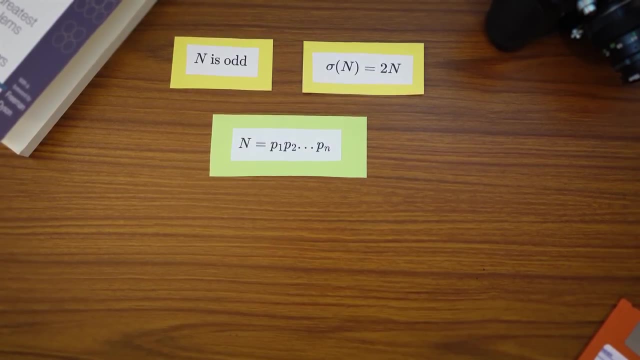 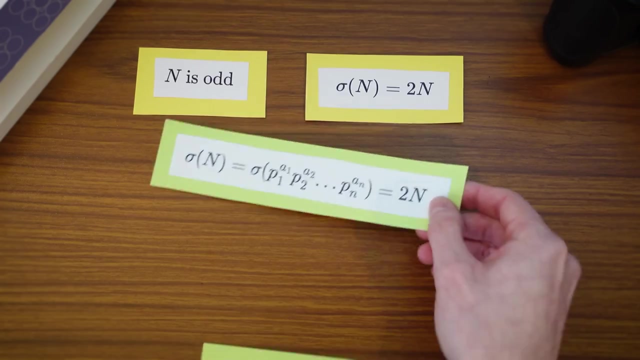 odd, perfect number does exist. you know two things: First, n is odd, And second, sigma of n equals 2n. Now, any number n you can write as a product of different prime numbers, And each prime can be to some power. So let's take that and put it into Euler's sigma function, So you get sigma of. 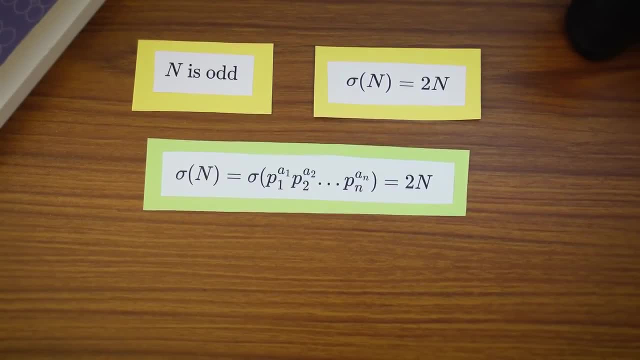 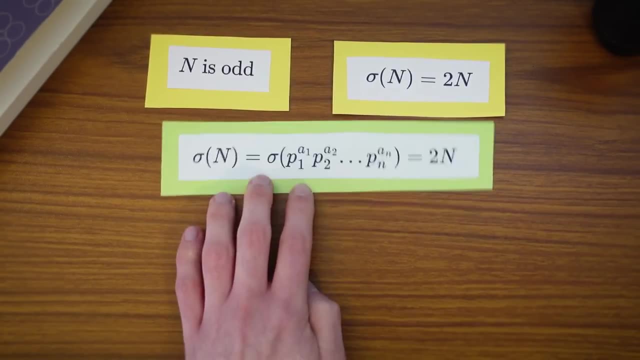 n equals sigma of all of those primes to their powers, which equals 2n. But since all of these factors are primes, you can actually split up the sigma function into two, So you get sigma of n equals sigma of all of those prime powers. So what you can then do is knowing those primes. 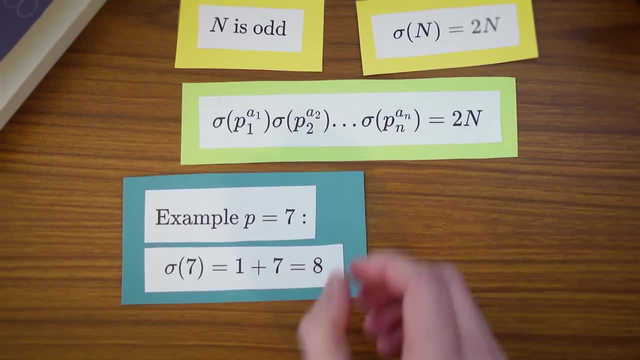 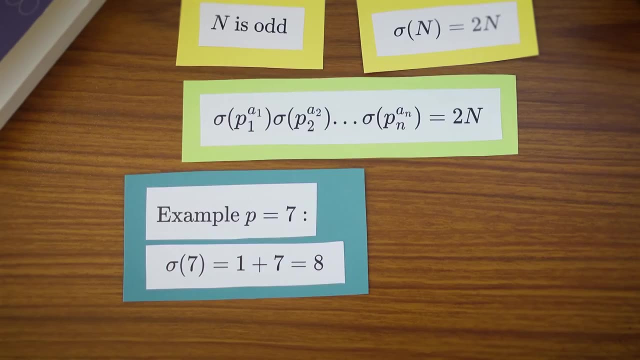 Now, one thing to notice is that if you have a prime number raised to an odd power- for example 7 to the power of 1, then the sigma function will be even. when reading the sigma function which equals 1. You'll always get an even number because odd means odd. 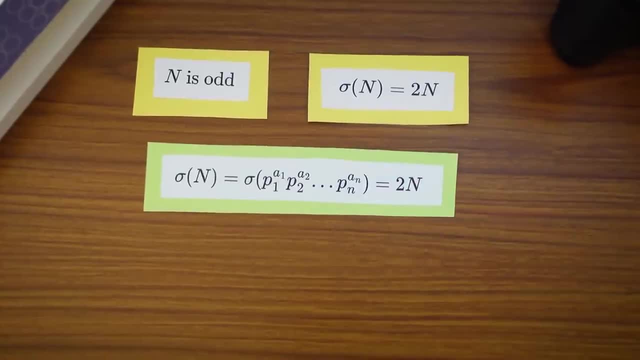 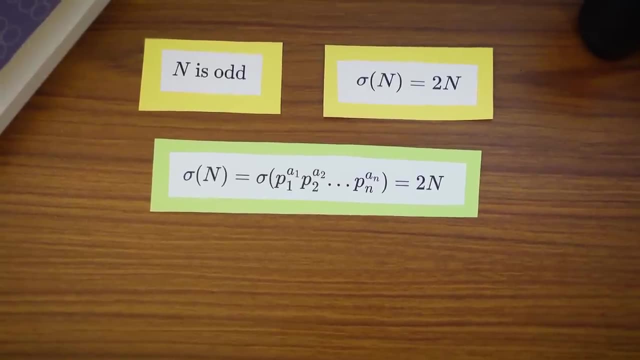 So let's take that and put it into Euler's sigma function. So you get sigma of n equals sigma of all of those primes to their powers, which equals two n. But since all of these factors are primes, you can actually split up the sigma function. 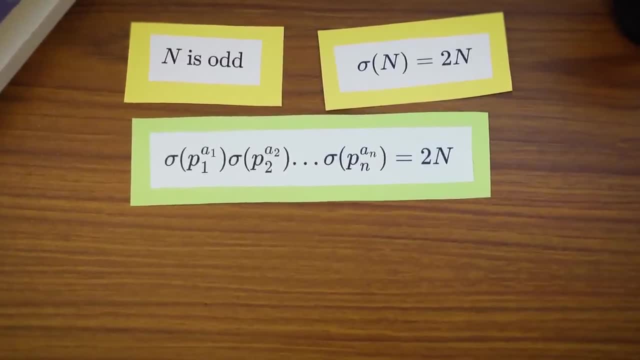 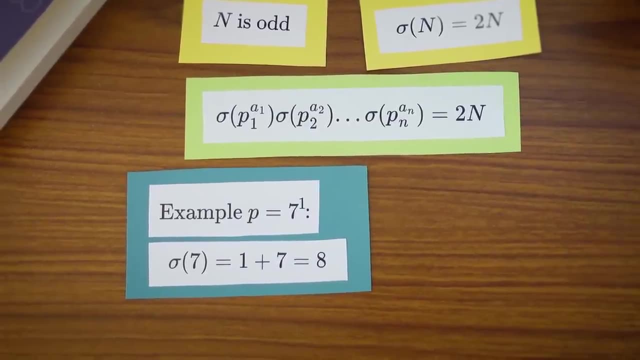 into the sigmas of the individual prime powers. Now one thing to notice is that if you have a prime number raised to an odd power, for example seven to the power of one, then the sigma function will be even, because one plus seven equals eight. 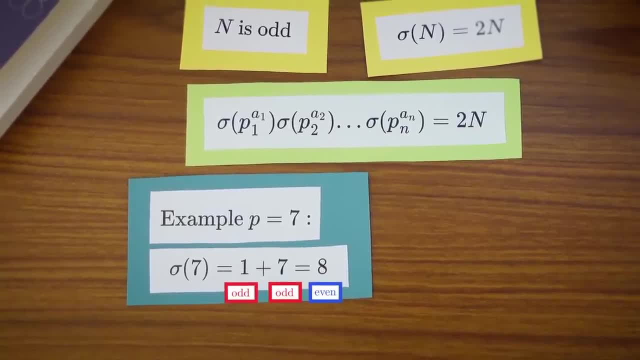 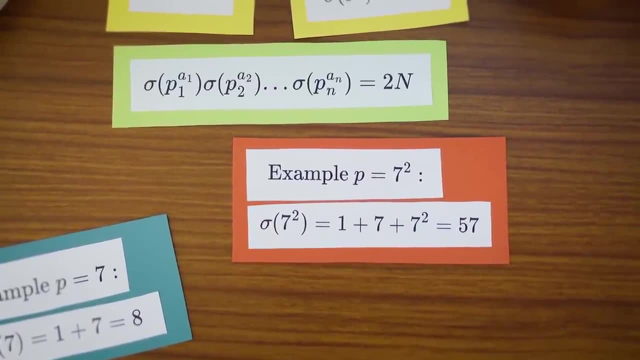 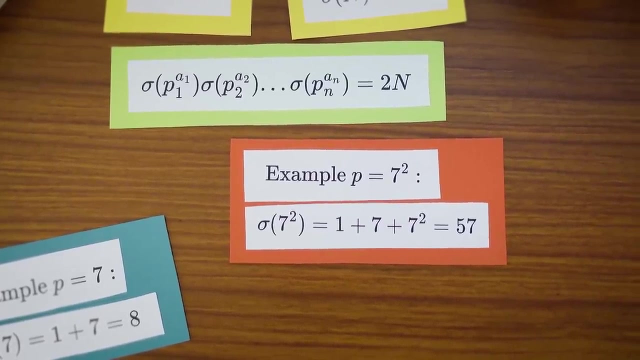 You'll always get an even number, because odd plus odd is even. If the prime number is instead raised to an even power, like seven squared, then the sigma function returns an odd number. Sigma of seven squared equals one plus seven plus seven squared, which equals 57.. 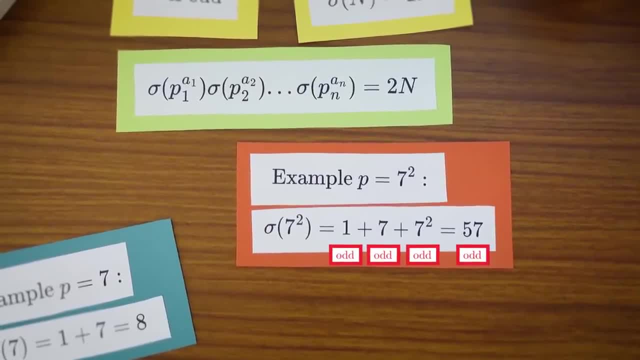 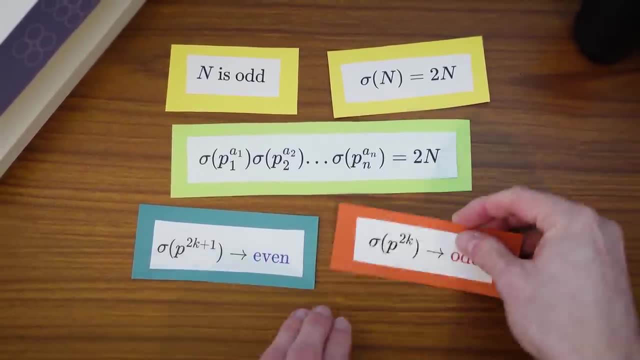 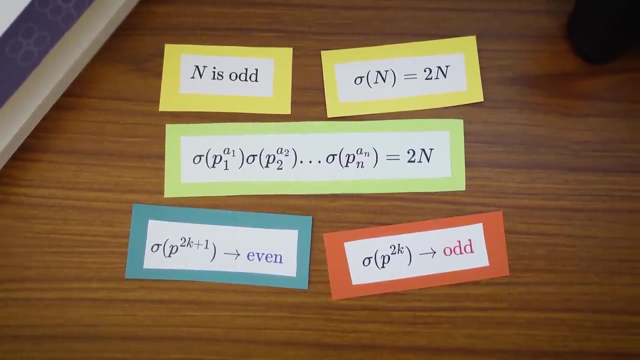 Because odd plus odd plus odd equals odd. So if you have the sigma function of an odd prime raised to an odd power, it will give an even number. If instead it's raised to an even power, you get an odd number. And this is where Euler's genius insight comes in. 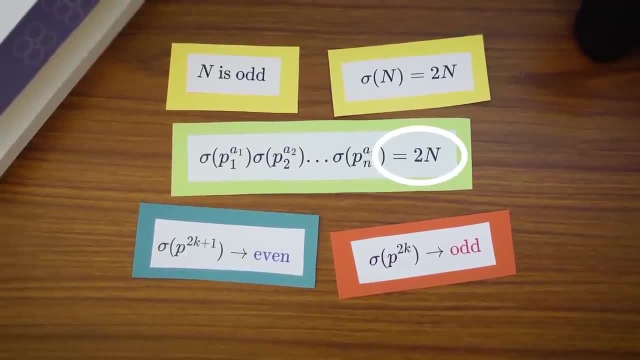 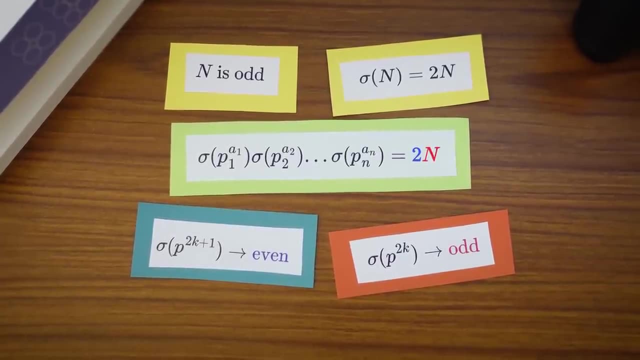 Because here on the right side you've got two times n, where n is an odd perfect number and two is even. Well, what that means is that on the left side there must only be one even number, Because if there were two even numbers, 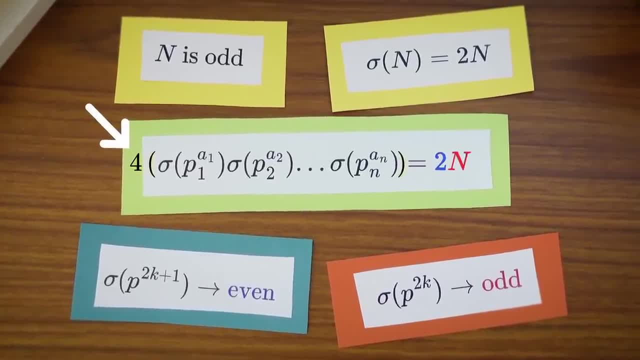 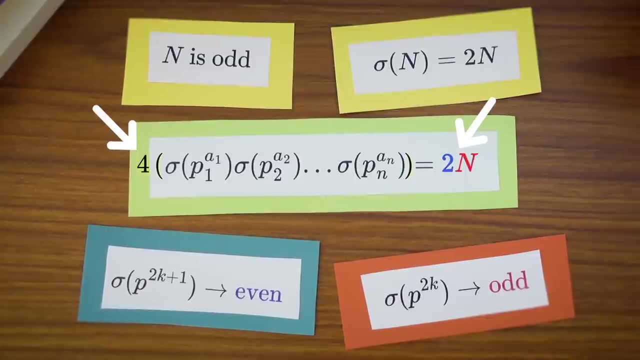 you could factor out four, But that means you should also be able to factor out four on the right side, which you can't, because n is odd and there's only a single two here. So only one of these sigmas here can give an even number. 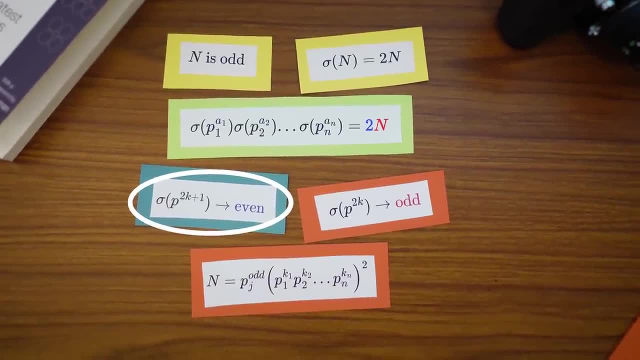 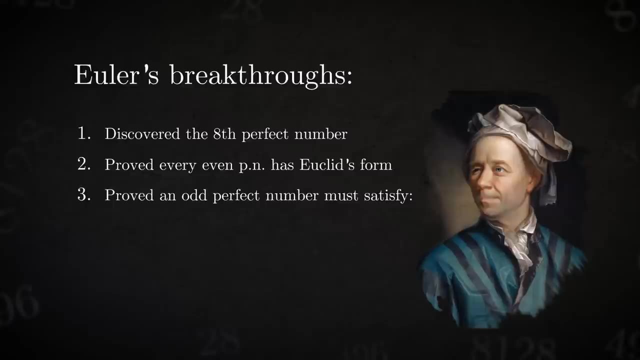 which means that there is exactly one prime, that is to an odd power, and all the others must be to an even power, just as Descartes had predicted. Now Euler refined the form a bit more and showed that an odd perfect number must satisfy this. 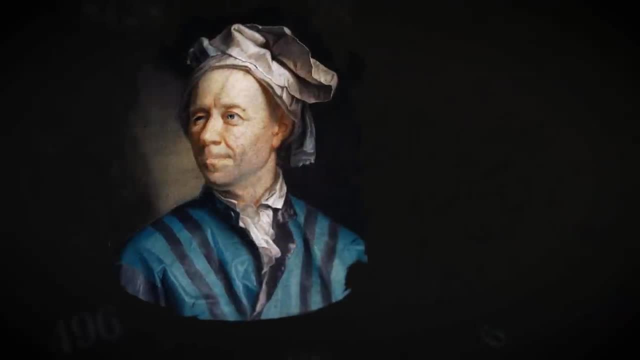 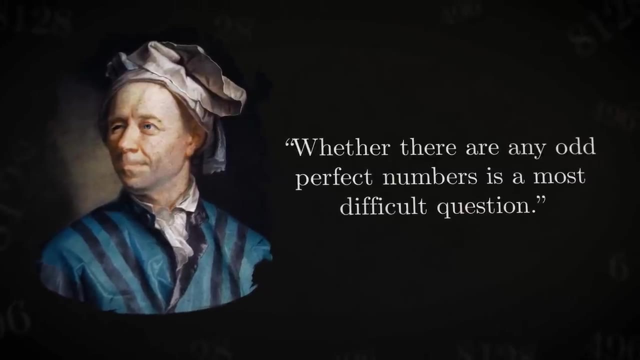 and that's exactly what we're going to do. But even Euler couldn't prove whether they existed or not. He wrote: whether there are any odd perfect numbers is a most difficult question For the next 150 years. very little progress was made. 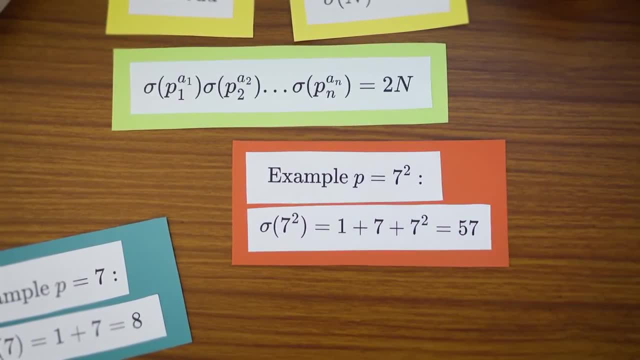 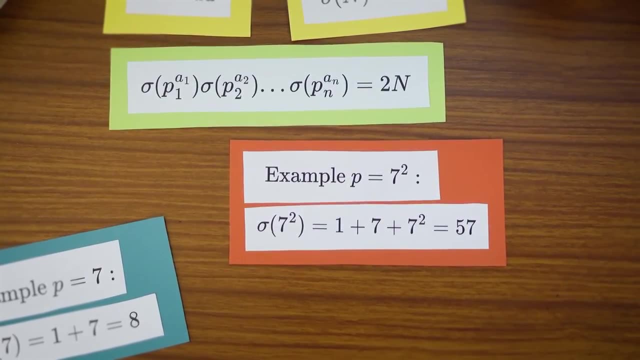 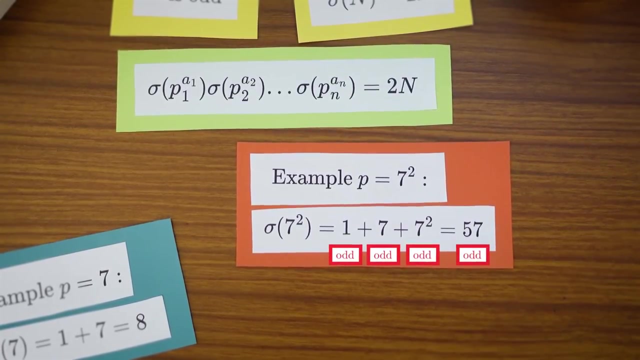 What if the prime number is instead raised to an even power, like 7 squared? then the sigma function returns an odd number. sigma of 7 squared equals 1 plus odd, 7 plus 7 squared, which equals 57.. Because odd plus odd plus odd equals odd. So if you have the 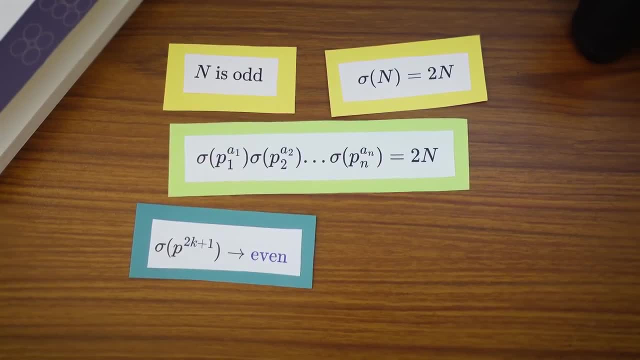 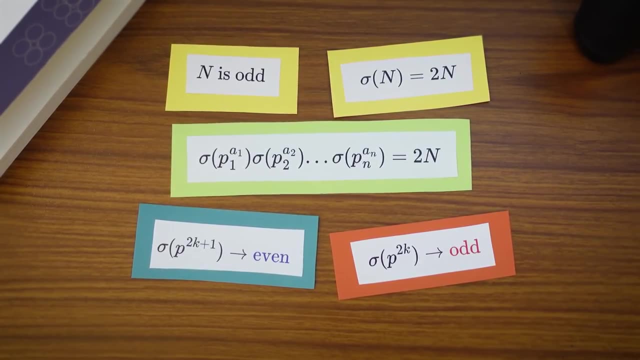 sigma function of an odd prime. raised to an odd power, it will give an even number. If, instead, it's raised to an even power, you get an odd number. And this is where Euler's genius insight comes in, Because here on the right side you've got 2 times n, where n is an odd, perfect number. 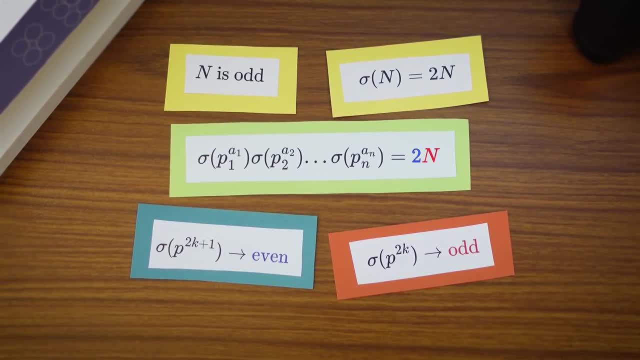 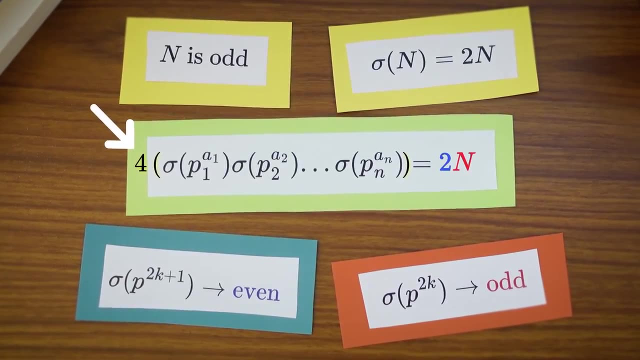 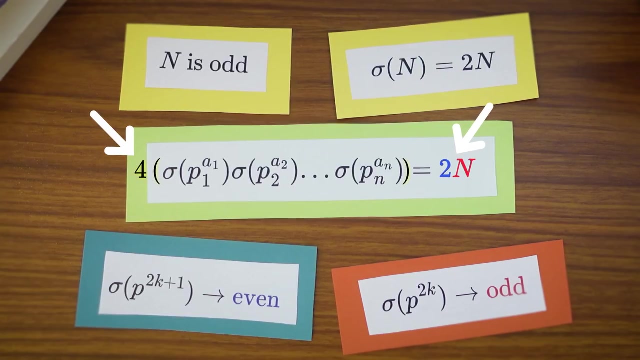 and 2 is even. Well, what that means is that on the left side there must only be one even number, Because if there were two even numbers, you could factor out 4.. But that means you should also be able to factor out 4 on the right side, which you can't because n is odd and there's only a single. 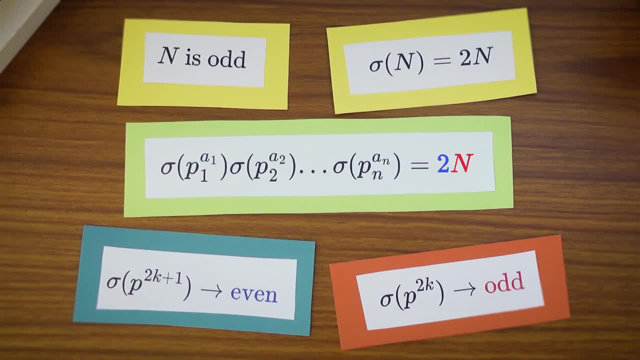 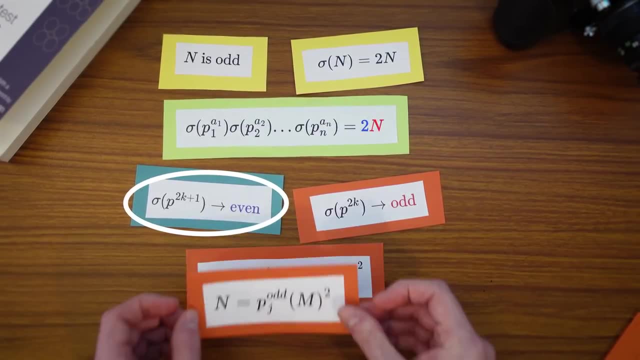 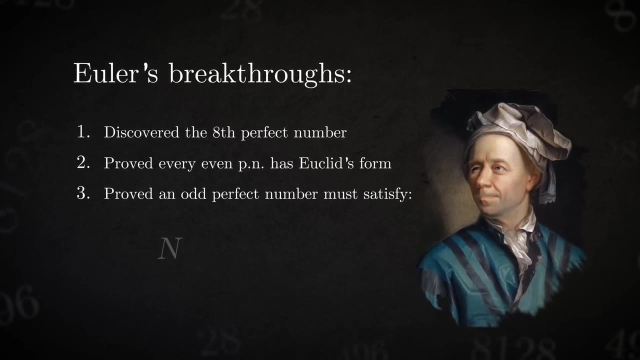 2 here. So only one of these sigmas here can give an even number, which means that there is exactly one prime that is to an odd power, and all the others must be to an even power, just as Descartes had predicted. Now Euler refined the form a bit more and 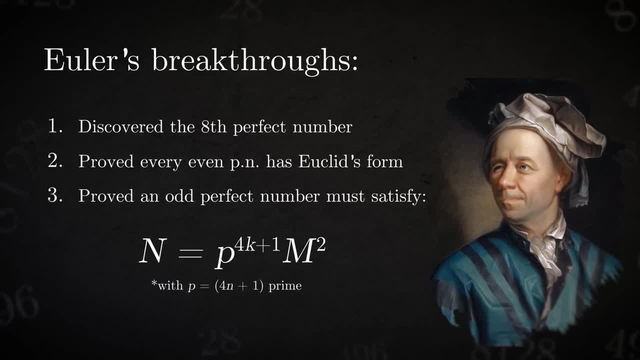 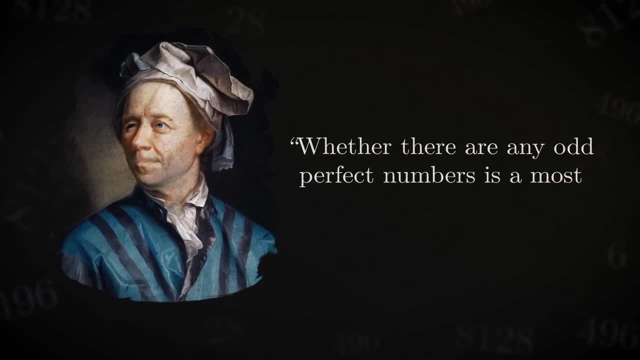 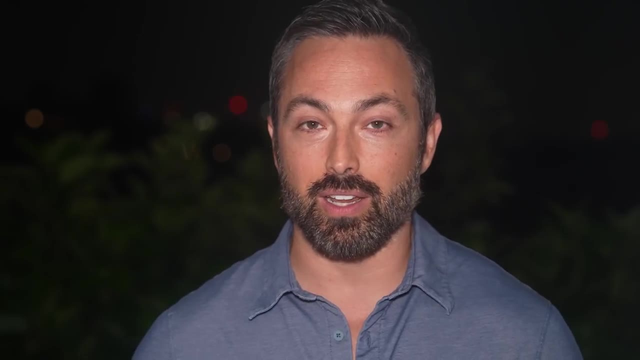 showed that an odd perfect number must satisfy this condition. But even Euler couldn't prove whether they existed or not. He wrote: whether there are any odd perfect numbers is a most difficult question For the next 150 years. very little progress was made and no new perfect. 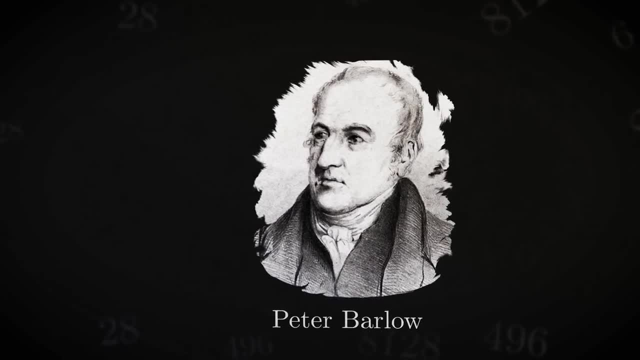 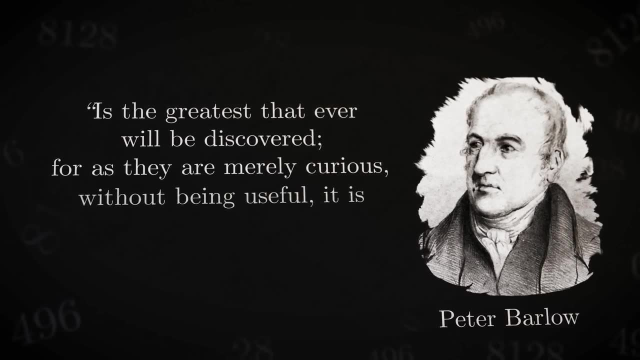 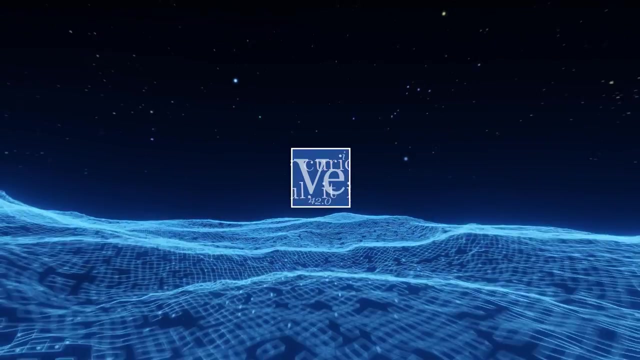 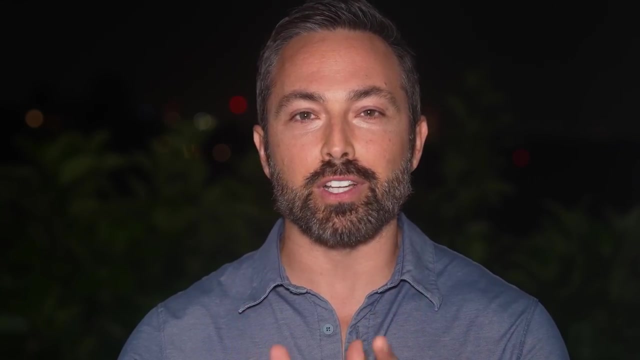 numbers were discovered. English mathematician Peter Barlow wrote that Euler's eighth perfect number is the greatest that ever will be discovered, For as they are merely curious without being useful, it is not likely that any person will ever attempt to find one beyond it. But Barlow was wrong. Mathematicians kept pursuing these elusive perfect numbers. 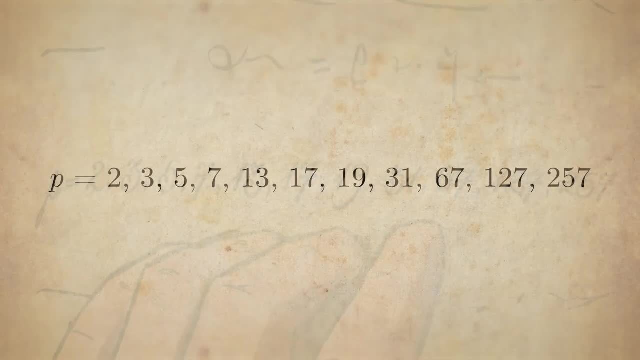 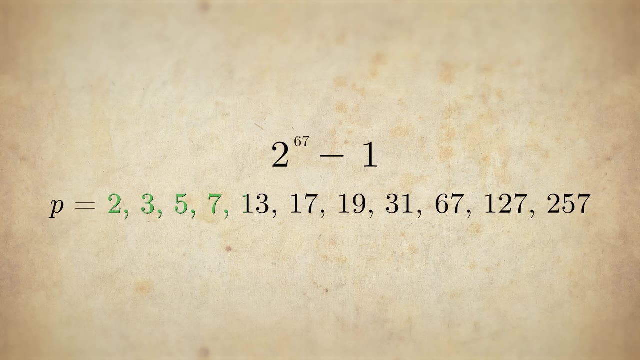 and most started with Mersenne's list of proposed primes. The next on his list was 2 to the 67 minus 1.. So far, Mersenne's list of proposed primes has been the most popular and the most popular. Mersenne had done an excellent job. He had included Euler's eighth perfect number, while 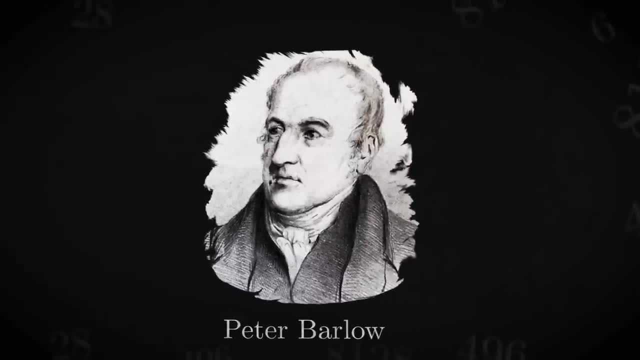 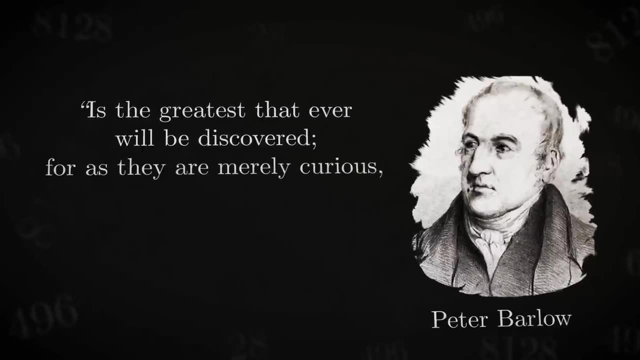 and no new perfect numbers were discovered. English mathematician Peter Barlow wrote that Euler's eighth perfect number is the greatest that ever will be discovered, for as they are merely curious without being useful, it is not likely that any person will ever attempt to find one beyond it. 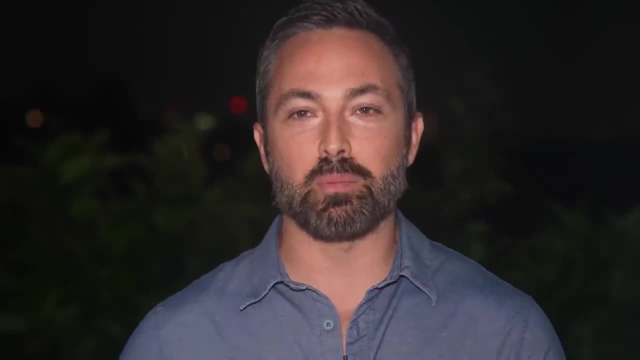 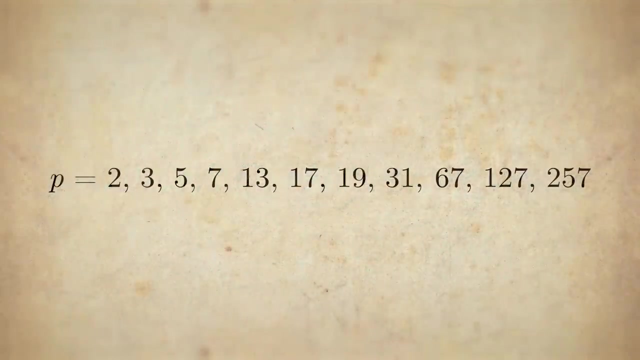 But Barlow was wrong. Mathematicians kept pursuing these elusive perfect numbers, and most started with Mersenne's list of proposed primes. The next on his list was two to the 67 minus one. So far, Mersenne had done an excellent job. 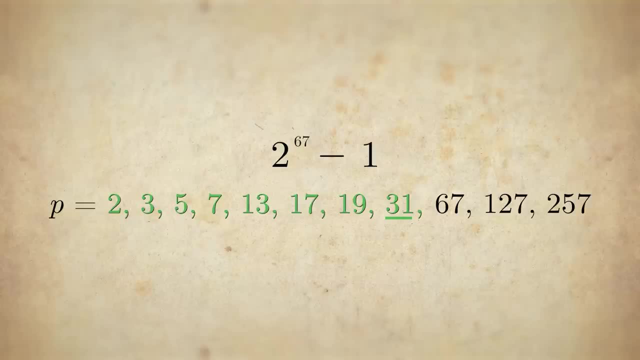 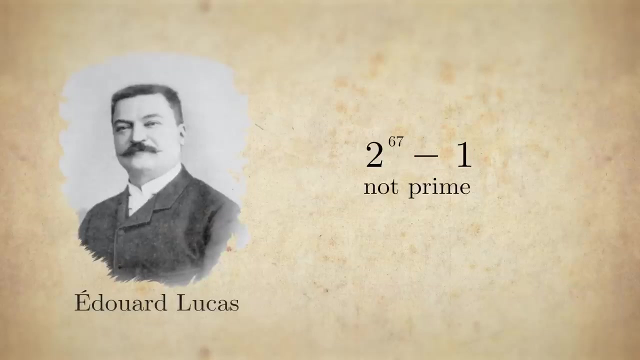 He had included Euler's eighth perfect number while avoiding others like 29. that turned out not to lead to a perfect number, But 230 years after Mersenne published his list, Eduard Luca proved that two to the 67 minus one was not prime, although he was unable to find its factors. 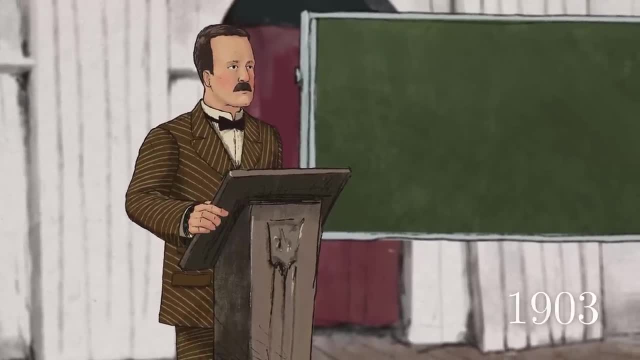 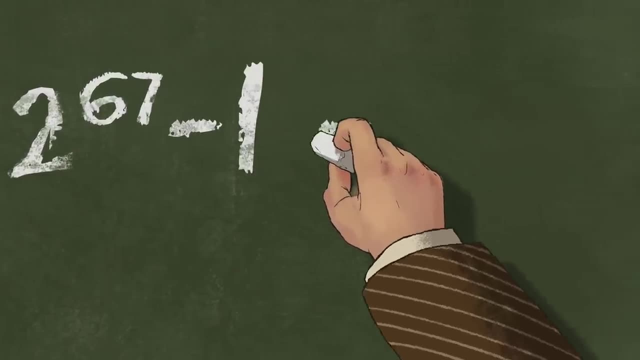 27 years later, Frank Nelson Cole gave a talk to the American Mathematical Society. Without saying a word, he walked to one side of the blackboard and wrote down: two to the 67 minus one equals 147 quintillion 573 quadrillion, 952 trillion. 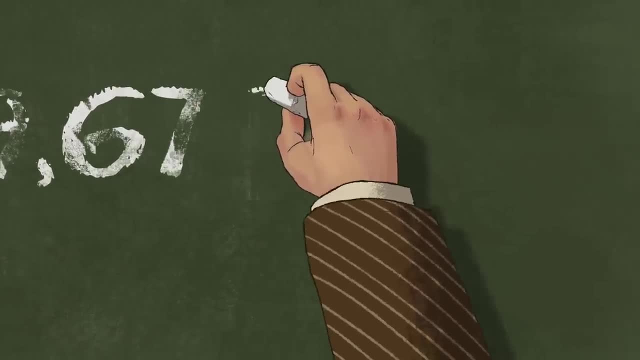 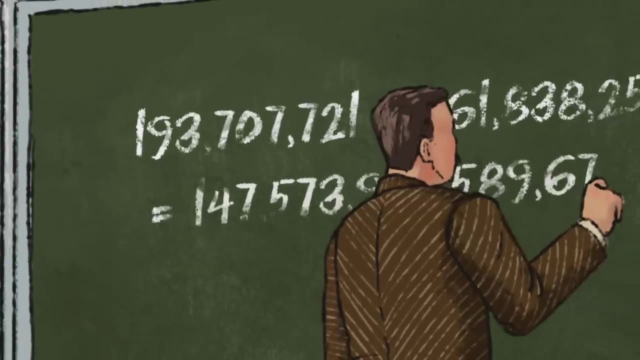 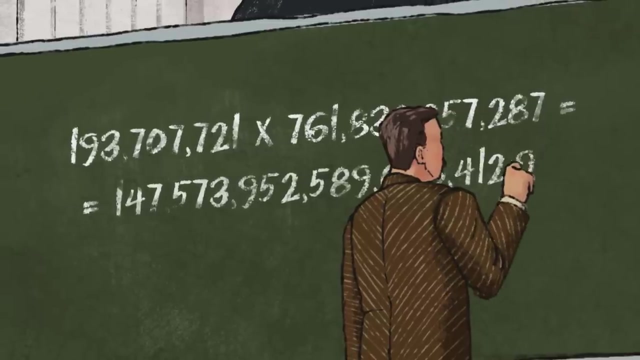 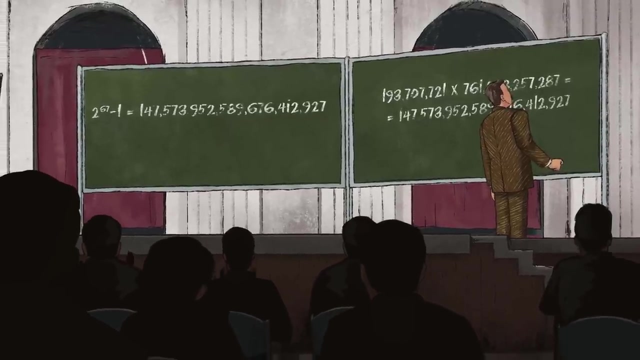 589 billion 676 million 412,927.. He then walked to the other side of the blackboard and multiplied 193 million 707,721 times 761 billion 838 million 257,287. giving the same answer, He sat down without saying a word. 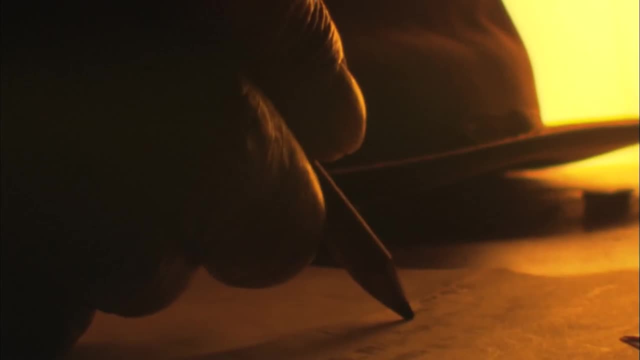 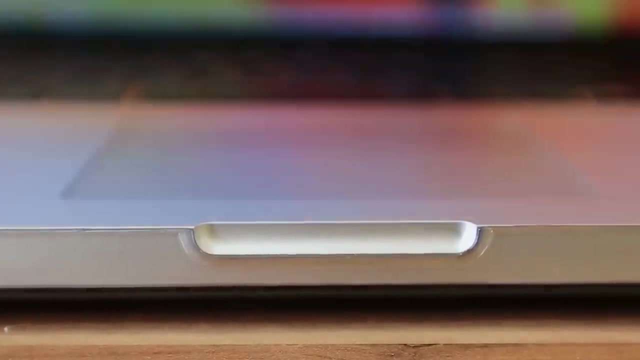 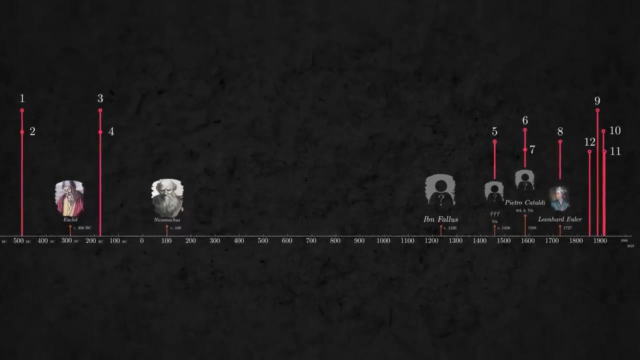 and the audience erupted in applause. He later admitted it took him three years, working on Sundays- to solve this. A modern computer could solve this in less than a second. From 500 BC until 1952, people had discovered just 12 Mersenne primes. 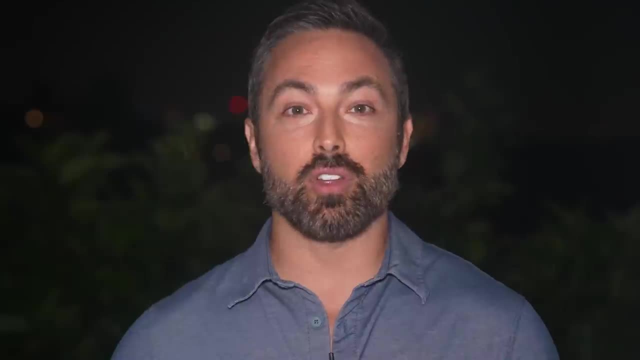 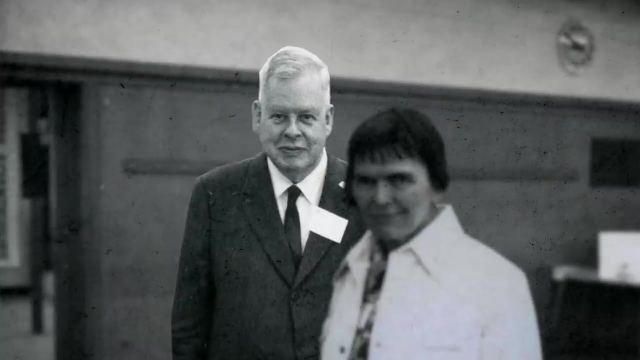 and therefore only 12 perfect numbers. The main difficulty was checking whether large Mersenne numbers were actually prime. But in 1952, American mathematician Raphael Robinson wrote a computer program to perform this task, and he ran it on the fastest computer at the time. 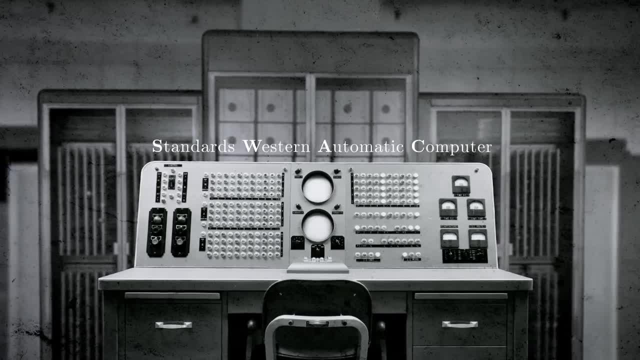 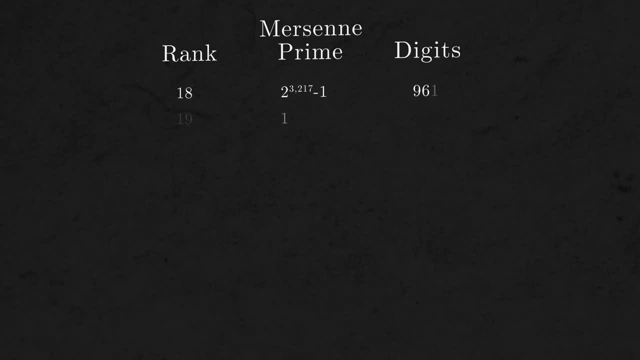 and he ran it on the fastest computer at the time, the SWAC. Within 10 months he found the next five Mersenne primes and so corresponding perfect numbers, And over the next 50 years new Mersenne primes were discovered in rapid succession. 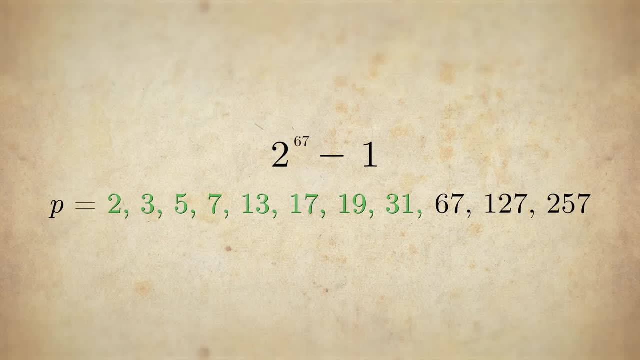 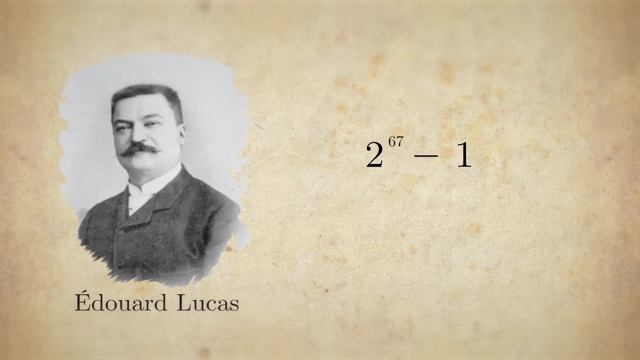 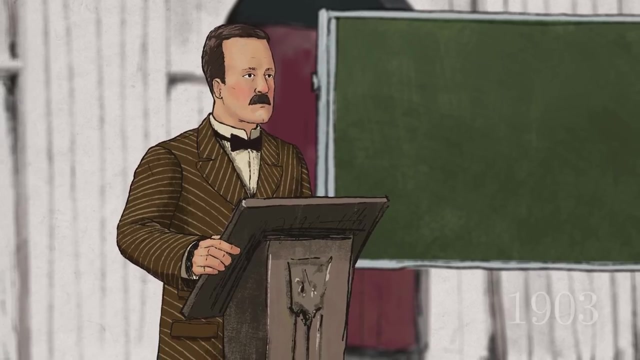 avoiding others like 29. that turned out not to lead to a perfect number. But 230 years after Mersenne published his list, Eduard Luca proved that 2 to the 67 minus 1 was not prime, although he was unable to find its factors. 27 years later, Frank Nelson Cole gave a talk to the American. 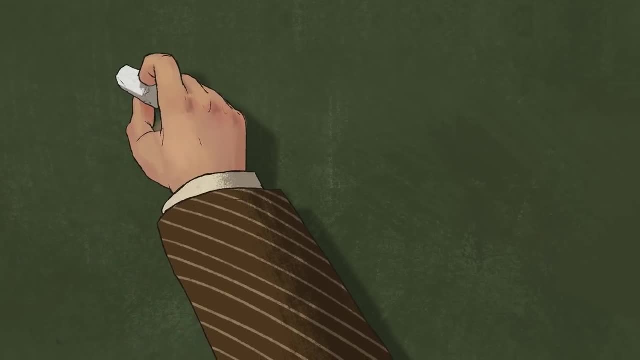 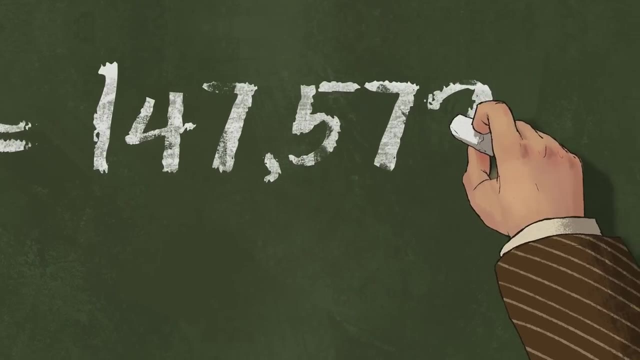 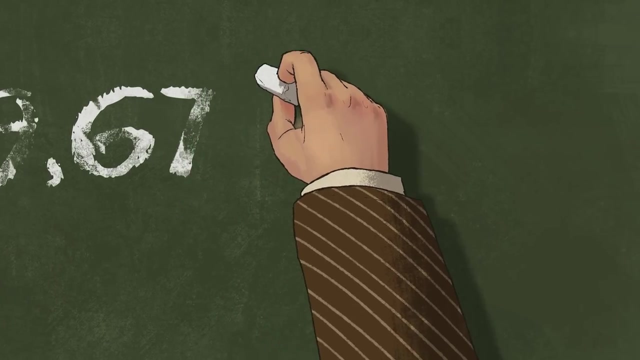 Mathematical Society. Without saying a word, he walked to one side of the blackboard and wrote down: 2 to the 67 minus 1 equals 147 quintillion 573 quadrillion 952 trillion 589 billion 676 million 412 thousand 927.. He then walked to the other side of the blackboard. 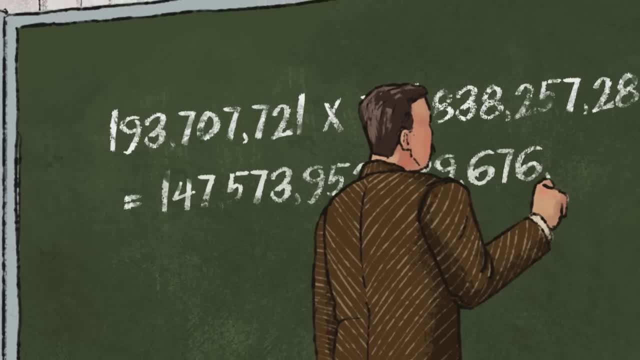 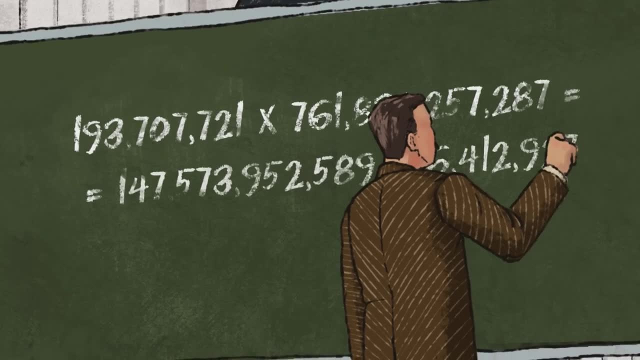 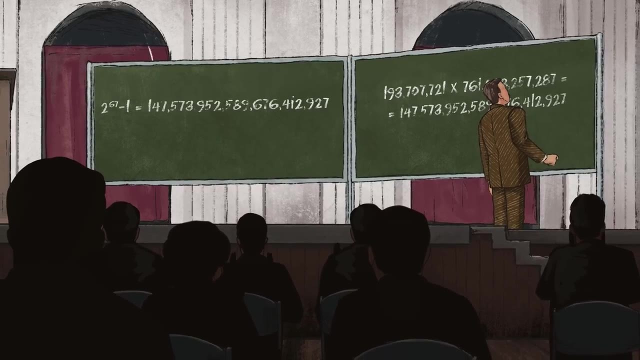 and multiplied 193 million 707 thousand 721 times 761 billion 838 million 257 thousand 287, giving the same answer, He sat down without saying a word and the audience erupted in applause. He later admitted it took him three years working on Sundays to 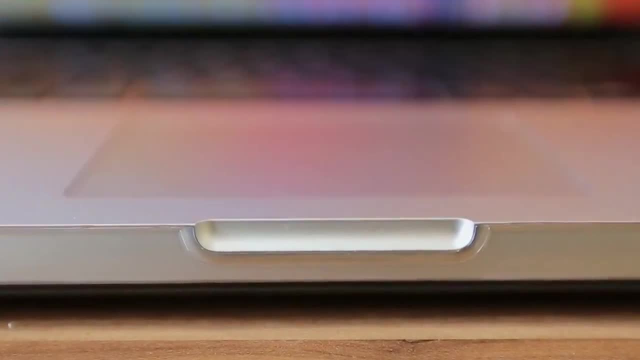 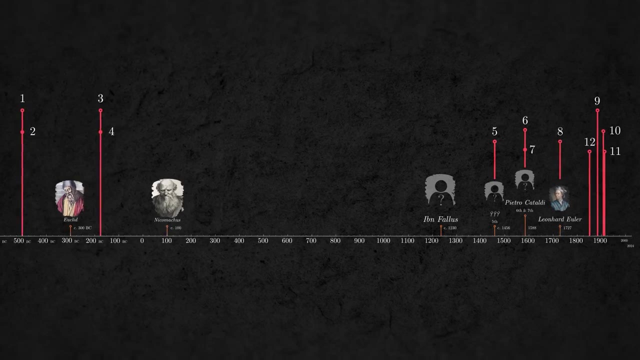 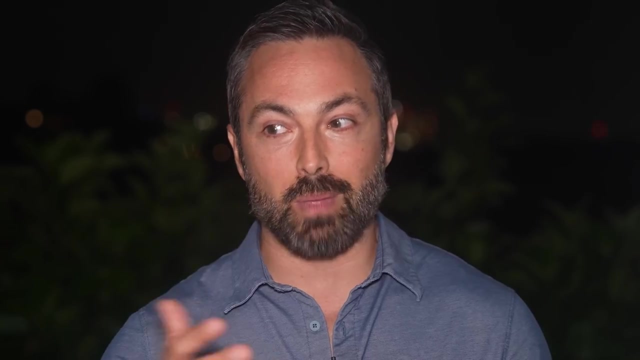 solve this. A modern computer could solve this in less than a second. From 500 BC until 1952, people had discovered just 12 Mersenne primes, and therefore only 12 perfect numbers. The main difficulty was checking whether large Mersenne numbers were. 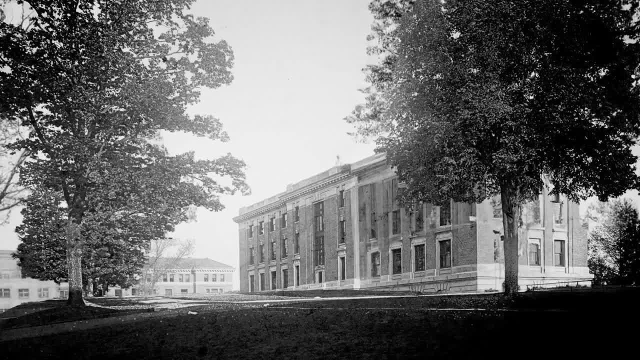 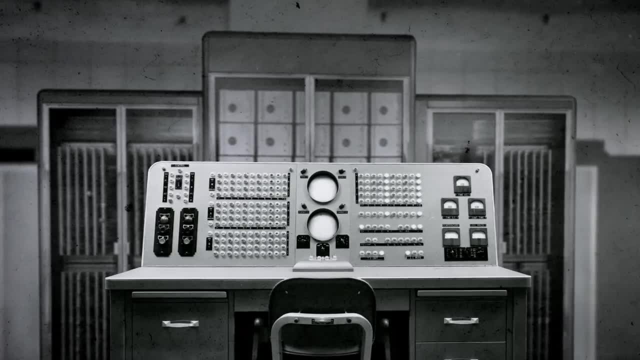 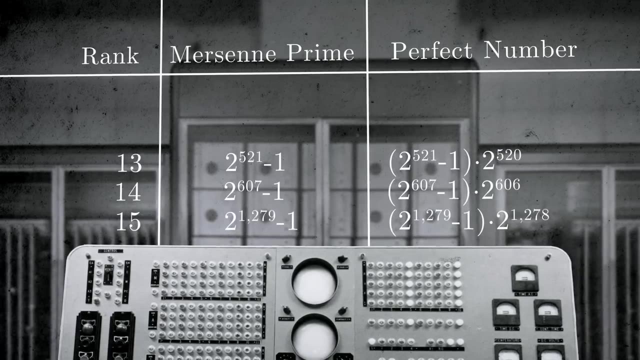 actually primes. But in 1952, American mathematician Raphael Robinson wrote a computer program to perform this task and he ran it on the fastest computer at the time, the SWAC. Within 10 months he found the next five Mersenne primes and so corresponding perfect numbers, And over the 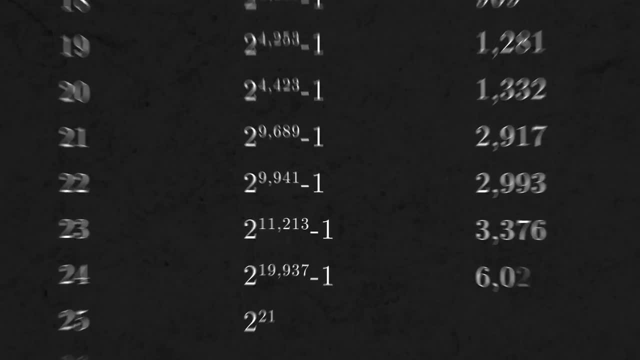 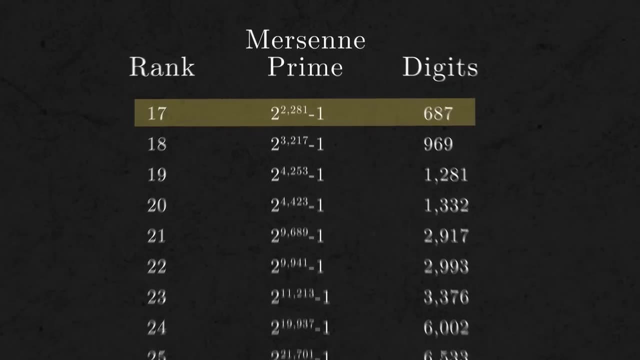 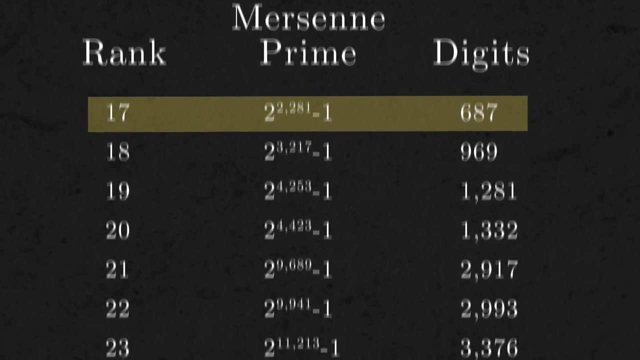 next 50 years. new Mersenne primes were discovered in rapid succession, all using computers. The largest Mersenne prime at the end of 1952 was 2 to the power of 2,000 quadrillion quadrillion, 281 minus 1, which is 687 digits long By the end of 1994, the largest Mersenne prime 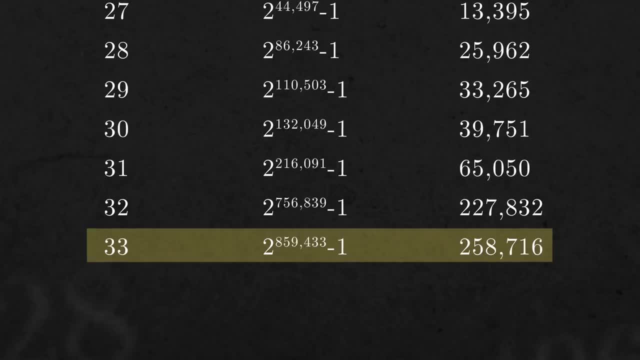 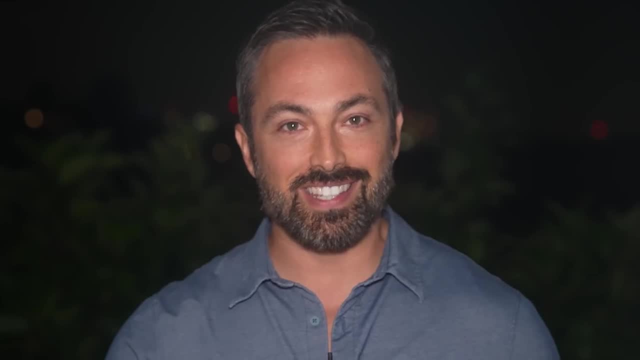 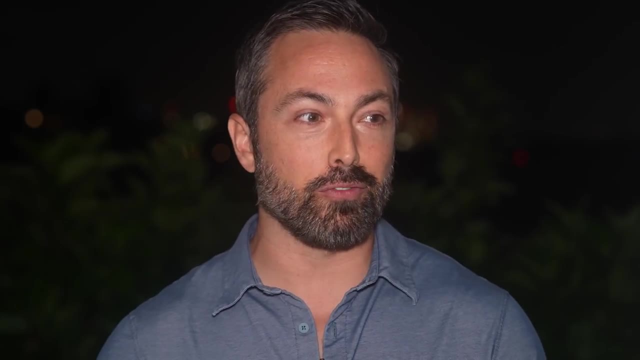 was 2 to the power of 859,433 minus 1, which is 258,716 digits long. Since these numbers were getting so astronomically large, the task of finding new Mersenne primes became more and more difficult, even for supercomputers. 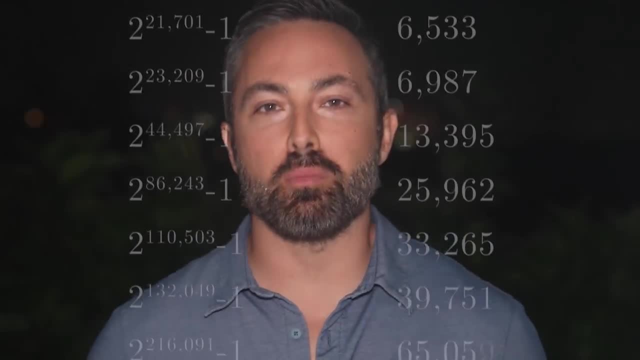 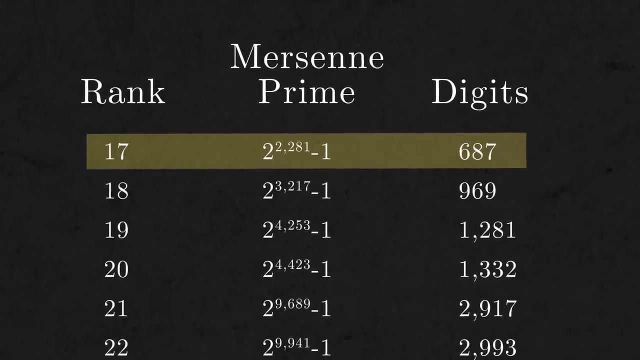 all using computers. The largest Mersenne prime at the end of 1952 was two to the power of 2,281 minus one which is 687 digits long By the end of 1994, the largest Mersenne prime. was two to the power of 859,000.. By the end of 1994, the largest Mersenne prime was two to the power of 859,000.. By the end of 1994, the largest Mersenne prime was two to the power of 859,000.. 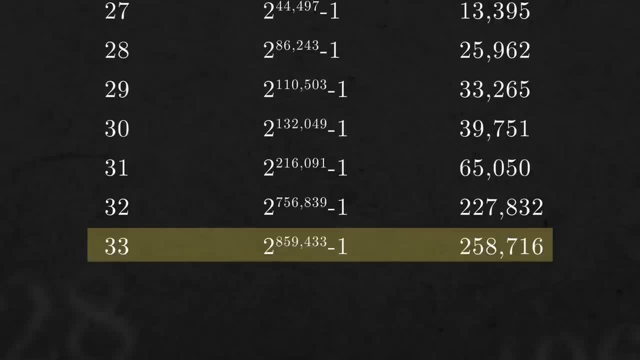 By the end of 243,. the largest Mersenne prime was two to the power of 433 minus one, which is 258,716 digits long, which is 258,716 digits long Since these numbers were getting so astronomically large. 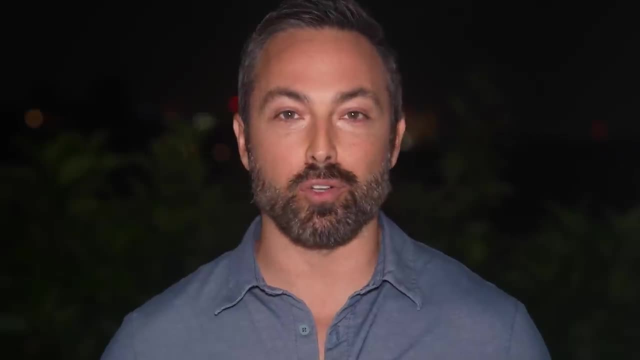 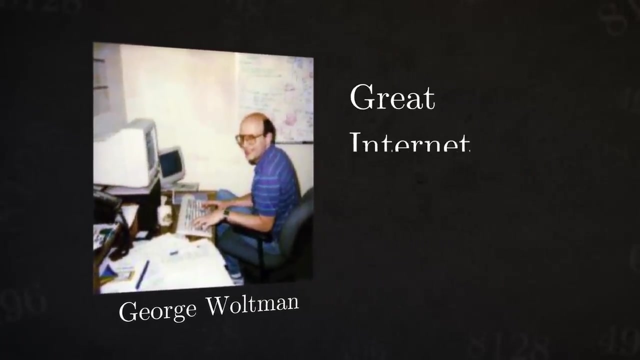 the task of finding new Mersenne primes became more and more difficult, even for supercomputers. So in 1996, computer scientist George Totman launched the great internet Mersenne prime search, or GIMPS. GIMPS distributes the work over many computers. 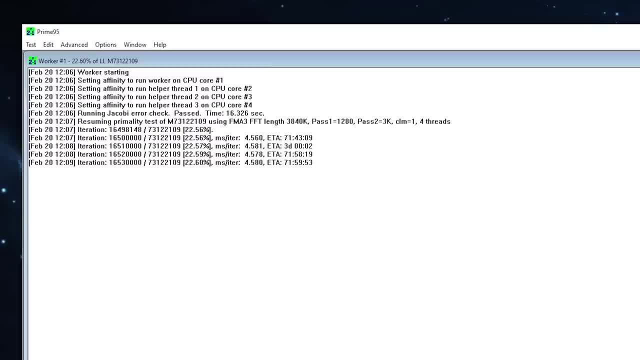 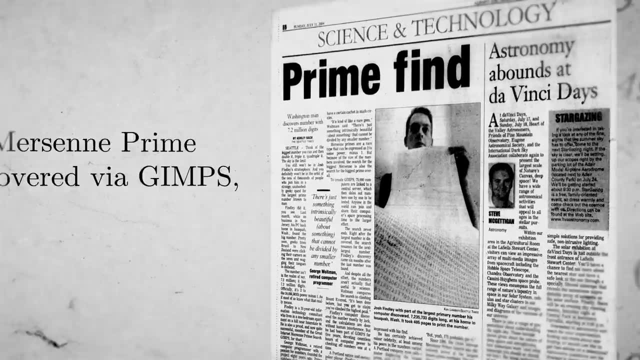 Allowing anyone to volunteer their computer power to help search for Mersenne primes. The project has been highly successful so far, having discovered 17 new Mersenne primes, 15 of which were the largest known primes at that time. And the best part. 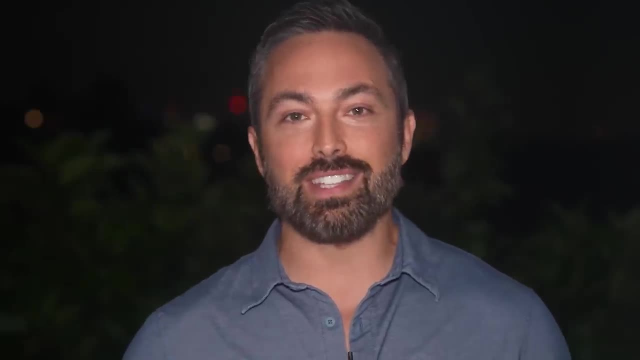 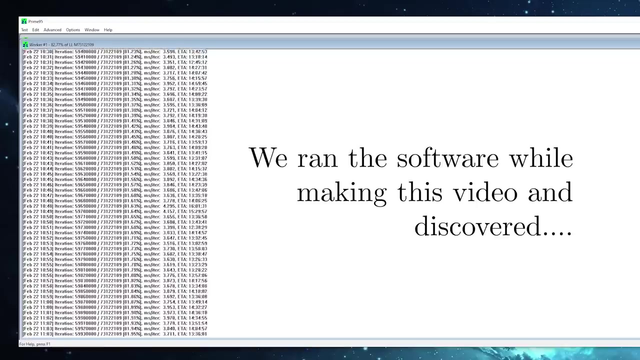 If your computer discovers a new Mersenne prime, you'll be listed as its discoverer, adding yourself to a list that includes some of the best mathematicians of all time. There's even a $250,000 prize for the first billion-digit prime. 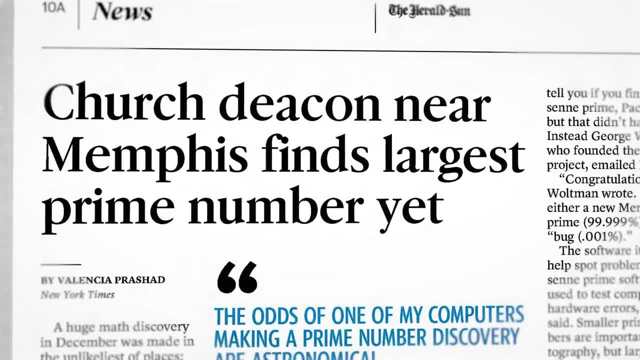 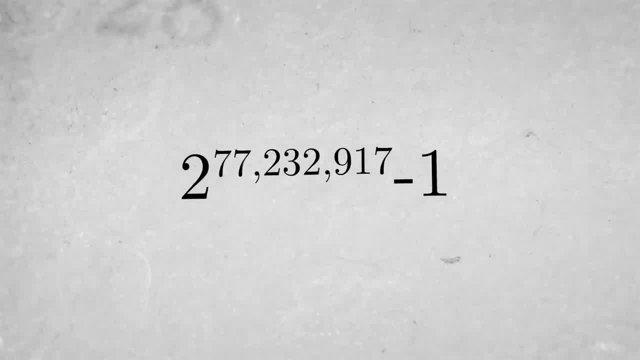 In 2017, church deacon John Pace discovered the 50th Mersenne prime by using GIMPS. The number 2 to the 77,232,917 minus 1, is more than 23 million digits long. 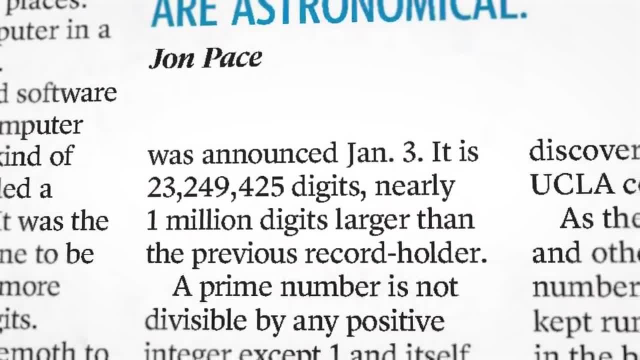 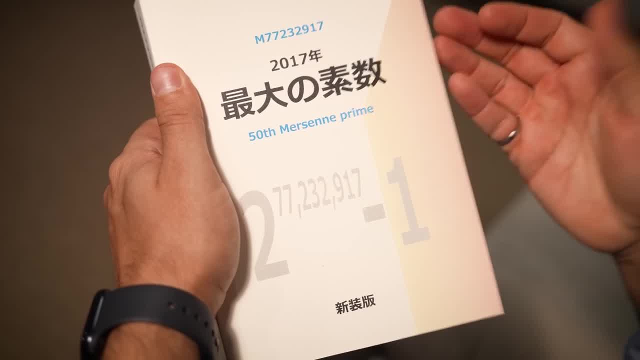 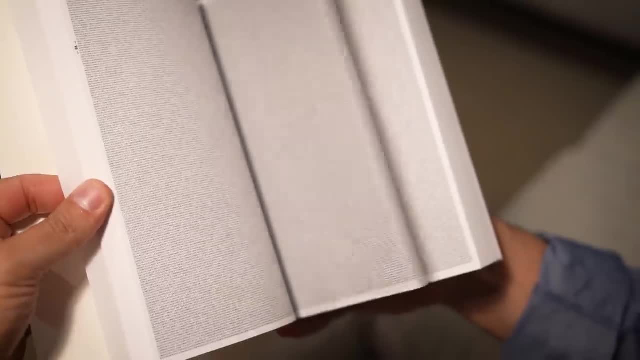 and it was also the largest known prime at the time. To celebrate this achievement, the Japanese publishing house Nanai Roshia published this book, the largest prime number of 2017.. And all it is is that That number spread over 719 glorious pages. It's wild. The size of this font is so tiny. The book quickly rose to the number one spot on Amazon and sold out in four days. A year later, the 51st Mersenne prime was discovered. It's 2 to the 82,589,933 minus 1.. 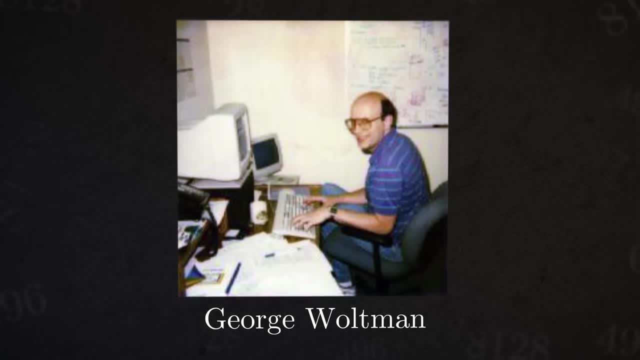 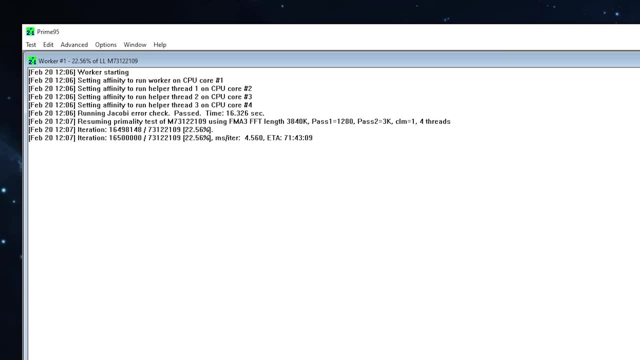 So in 1996, computer scientist George Woltman launched the Great Internet Mersenne Prime Search or GIMPS. GIMPS distributes the work over many computers, allowing anyone to volunteer their computer power to help search for Mersenne. 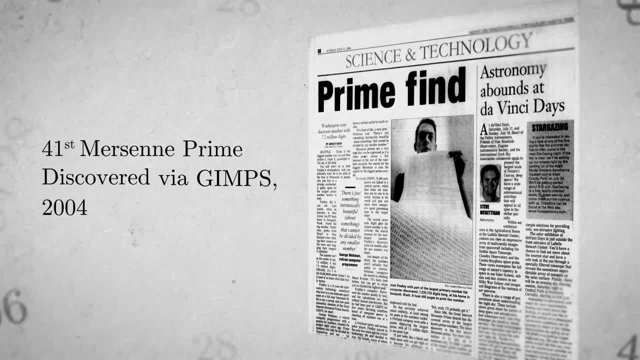 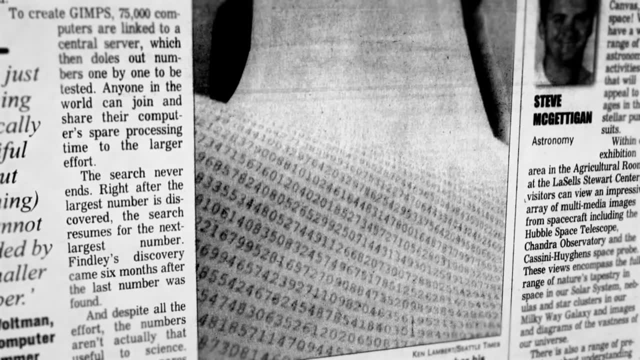 primes. The project has been highly successful so far, having discovered 17 new Mersenne primes, 15 of which were the largest known primes at that time. And the best part: If your computer discovers a new Mersenne prime, you'll be listed as. 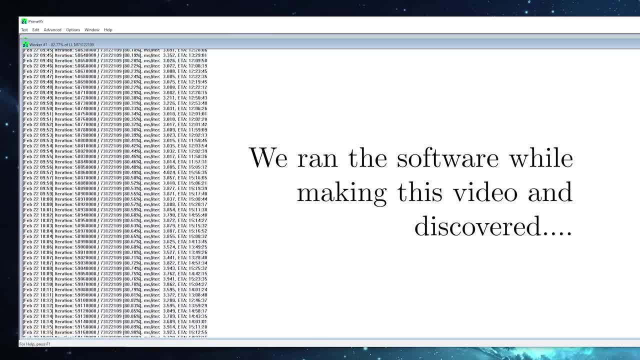 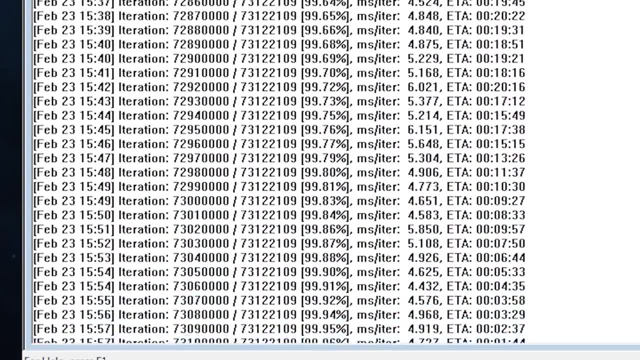 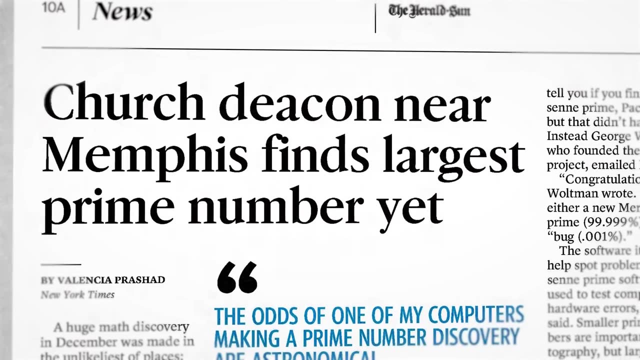 its discoverer, adding yourself to a list that includes some of the best math and computer mathematicians of all time. There's even a $250,000 prize for the first billion-digit prime. In 2017, Church deacon John Pace discovered the 50th Mersenne Prime by using GIMPS. The 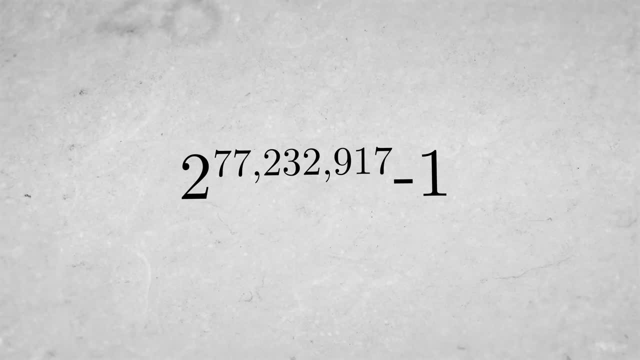 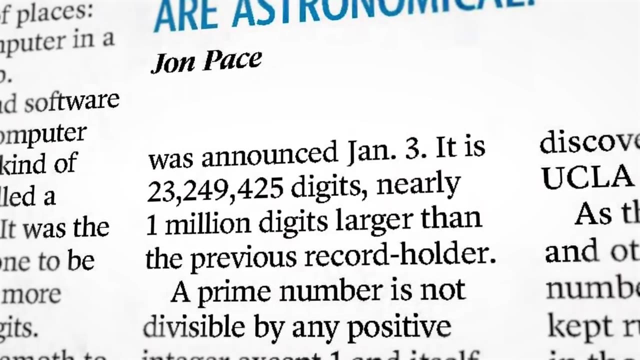 number 2 to the 77,232,917 minus 1, is more than 23 million digits long, and it was also the largest known prime at the time. The number 2 to the 77,232,917 minus 1, is more than 23 million digits long and it. 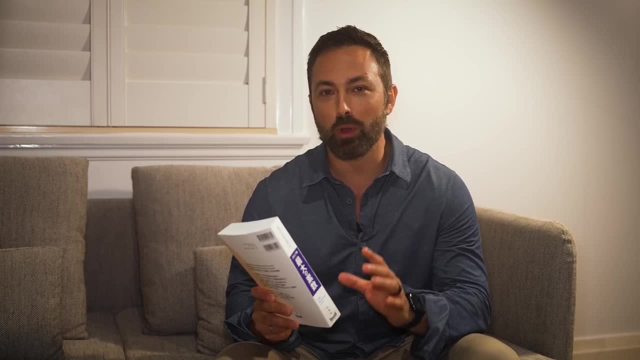 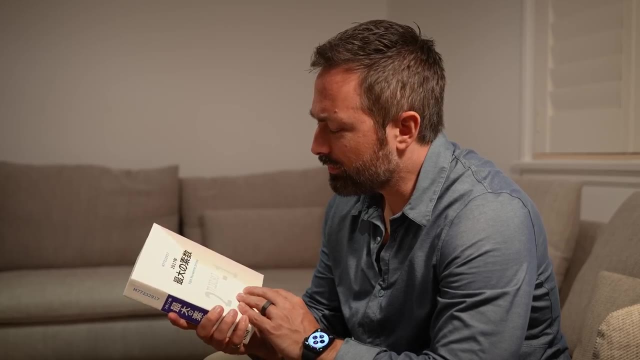 was also the largest known prime at the time achievement. the Japanese publishing house Nanai Roshia published this book: the largest prime number of 2017.. And all it is is that number spread over 719 glorious pages. It's wild. The. 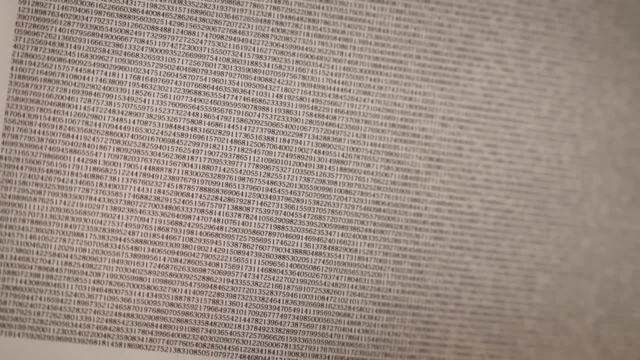 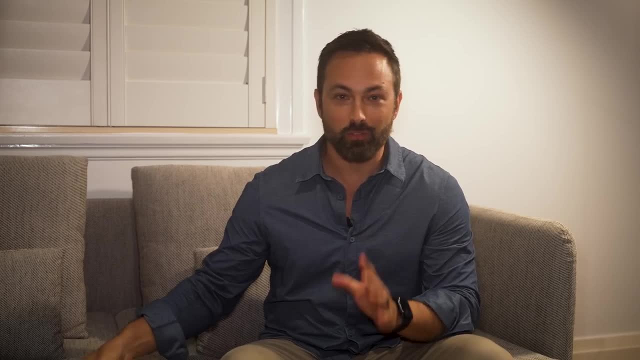 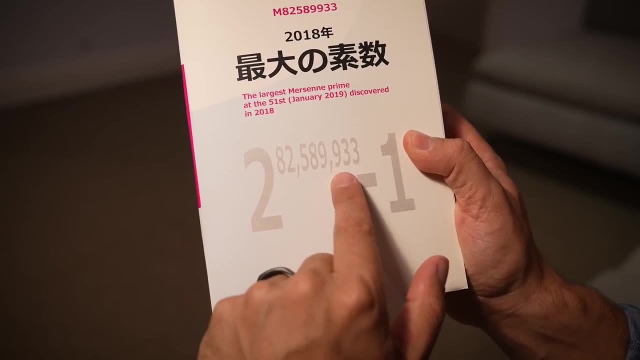 size of this font is so tiny. The book quickly rose to the number one spot on Amazon and sold out in four days. A year later, the 51st Mersenne prime was discovered. It's two to the 82,589,933. 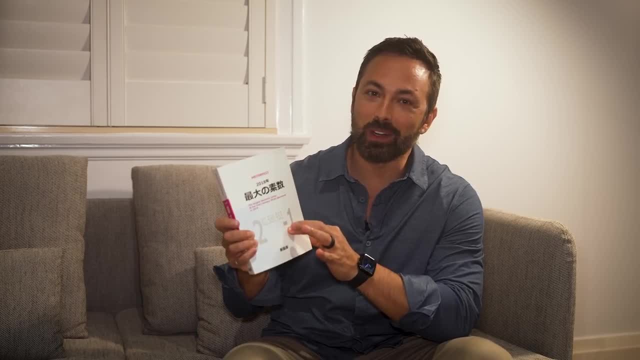 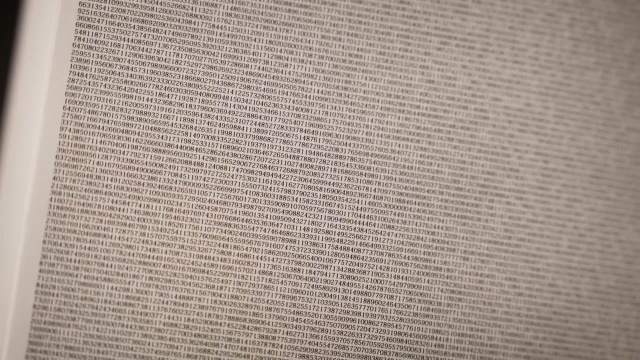 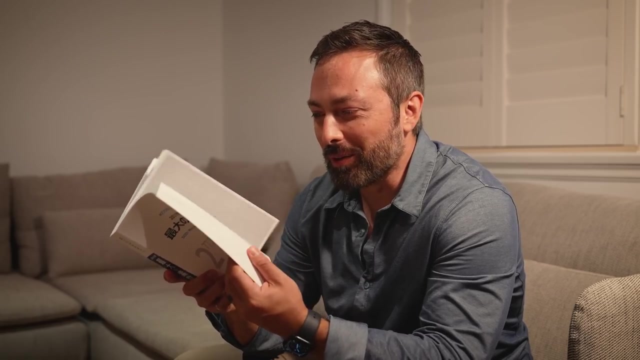 minus one, And this number has 24,862,048 digits. There's something I enjoy about the absurdity: Like there is knowledge in here, but it's not the kind of knowledge that anyone's ever going to read of a book, but in some way it's nice that there's this physical artifact that, like, has the number. 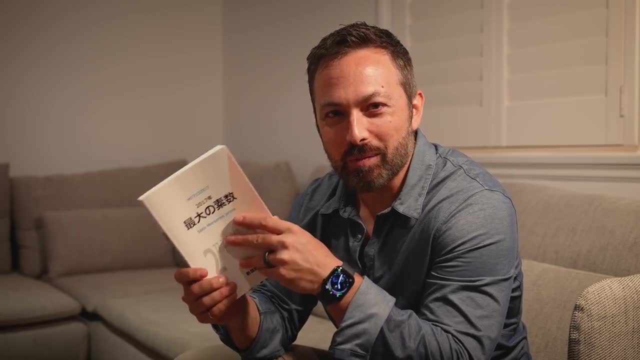 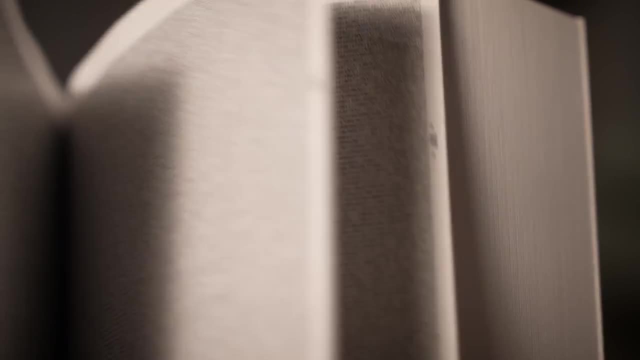 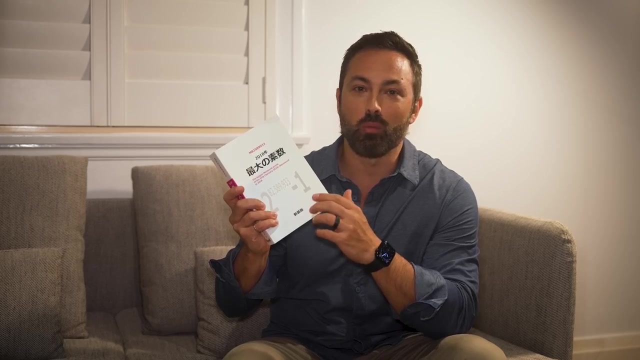 if ever we lost all the prime numbers you know, someone could find this book and be like: here's a big one. as of today, this is still the largest known prime and since numbers of this form grow so rapidly, the largest mersenne prime is almost always the largest known prime. 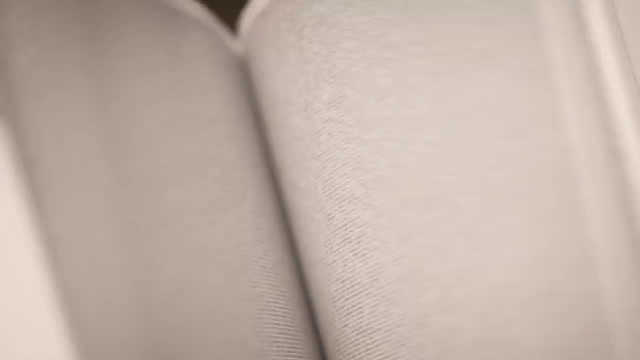 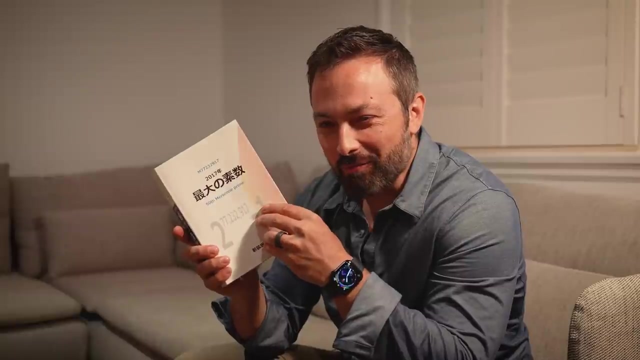 And this number has 24 million digits long, 24,862,048 digits. But there's something I enjoy about the absurdity: Like there is knowledge in here but it's not the kind of knowledge that anyone's ever going to read out of a book. 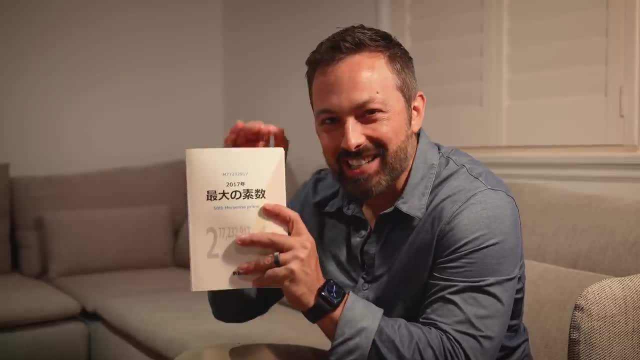 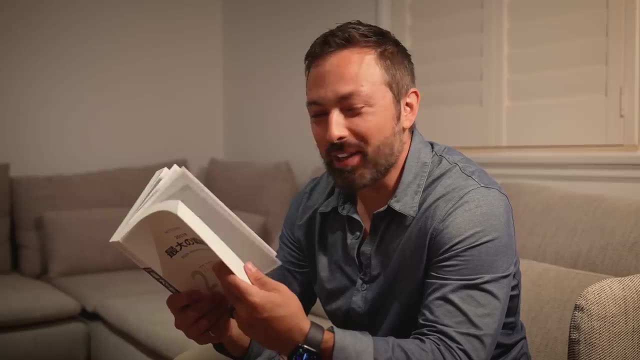 But in some way it's nice that there's this physical artifact that like has the number. If ever we lost all the prime numbers you know, someone could find this book and be like: here's a big one. As of today, this is still the largest prime number in the world. 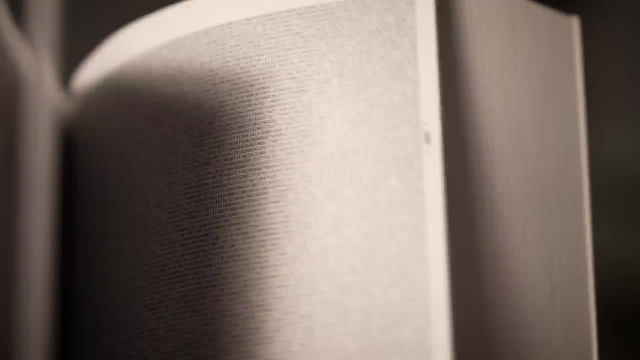 This is still the largest prime number in the world. This is still the largest prime number in the world. This is still the largest known prime And since numbers of this form grow so rapidly, the largest Mersenne prime is almost always the largest known prime. Computers have been incredibly successful at finding new Mersenne primes and their corresponding perfect numbers, But we've still only found 51 so far. So you might suspect that there are only a finite number of them, Which would mean that Nicomachus' fifth conjecture would be false. 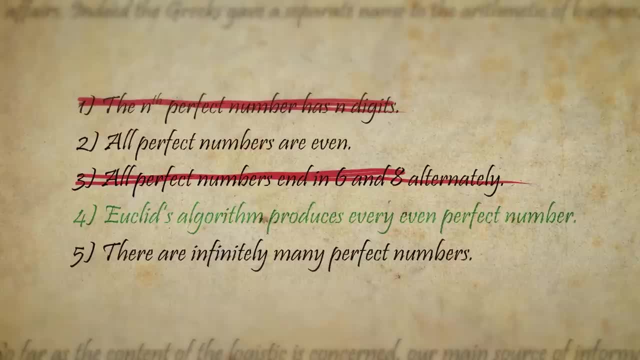 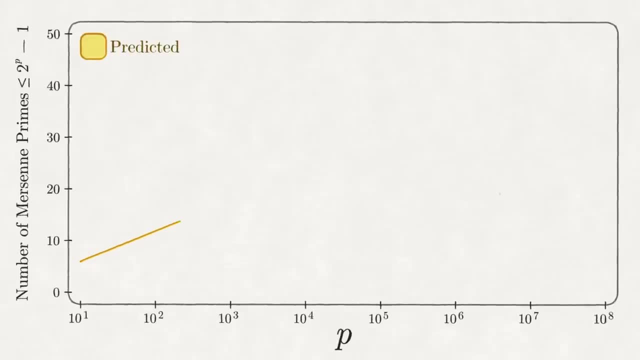 That there aren't infinitely many perfect numbers, But that might not be the case. The Leinster-Pomerantz-Wagstaff conjecture predicts how many Mersenne primes should appear, based on how large p is Now. this is the actual data. 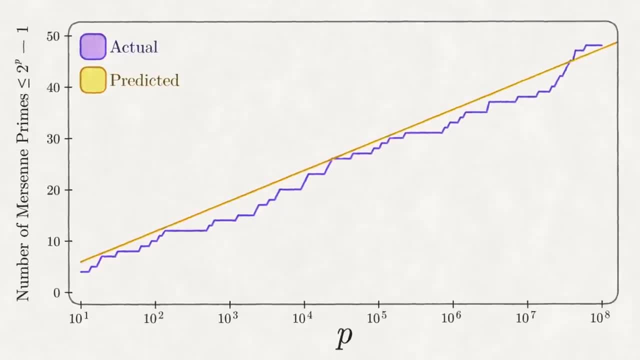 The conjecture performs remarkably well. But more importantly, it predicts that there are infinitely many Mersenne primes And so infinitely many even perfect numbers. The Mersenne primes are just so large and rare that they take a lot of time and computer. 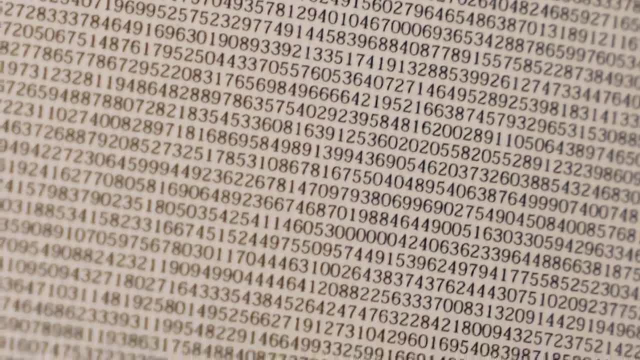 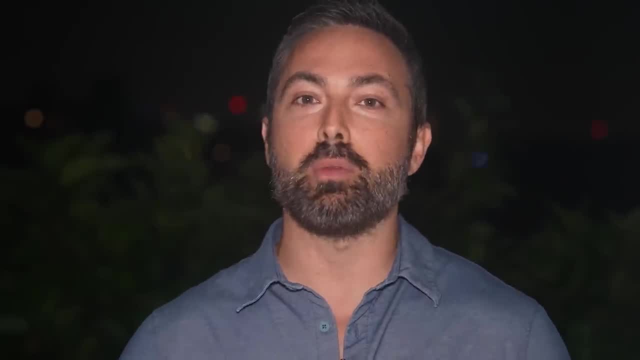 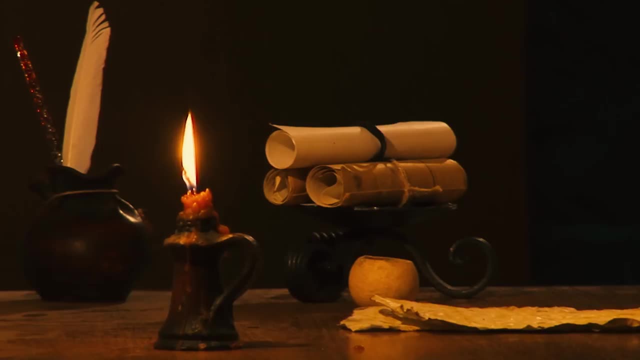 resources to find. But a conjecture is not a proof, And up until this day this problem shares the title of oldest unsolved problem in math with the other open problem: Do any odd perfect numbers exist? The easiest way to solve this problem is by finding an example. 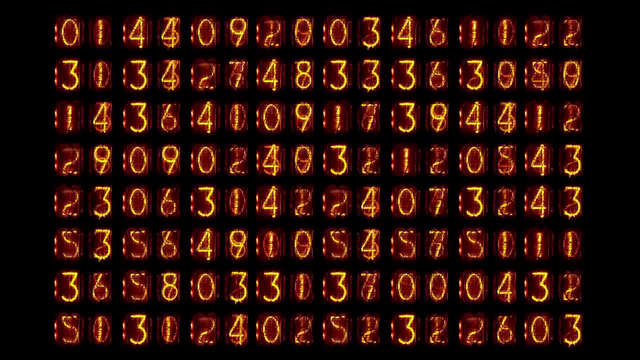 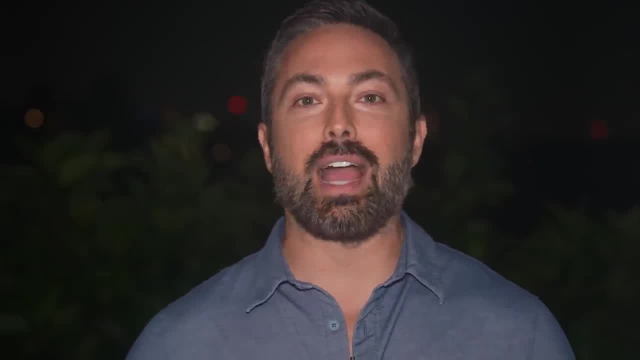 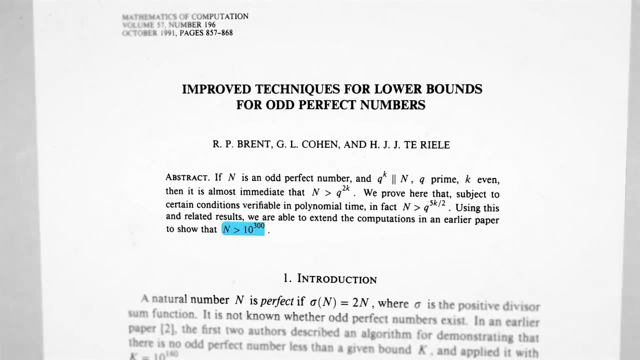 So maybe we could just check different odd numbers and see if one of them is perfect. That's exactly what researchers tried in 1991.. By using a smart algorithm called a factor chain, they were able to show that if an odd perfect number does exist, it must be larger than 10 to the power of 300. 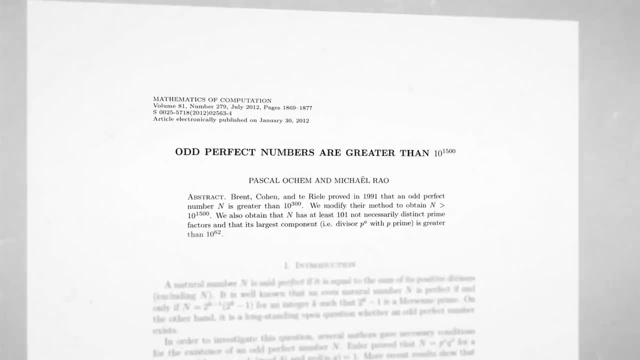 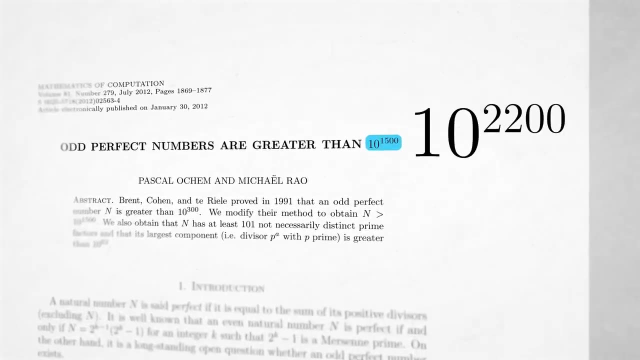 21 years later, Pascal Okum and Michael Rao raised that lower bound to 10 to the 1,500.. With recent progress pushing that number up to 10 to the 2,200.. With numbers that large it's unlikely that a computer will find one anytime soon. 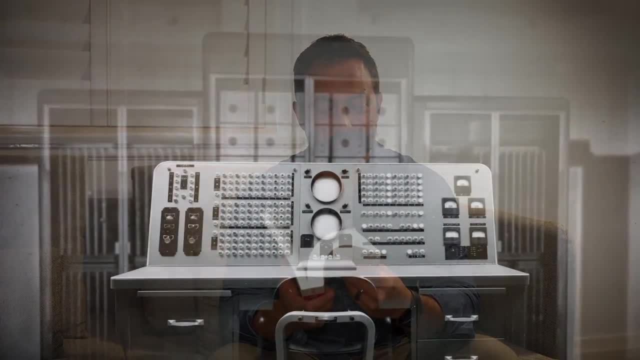 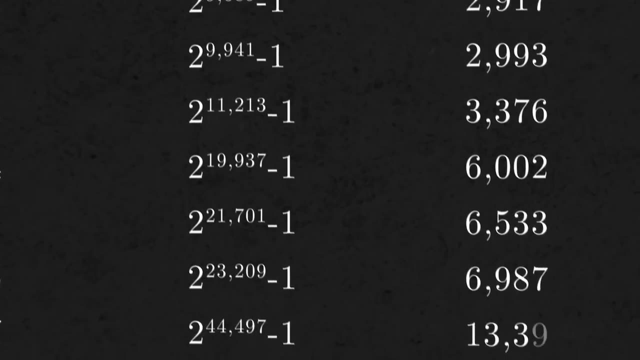 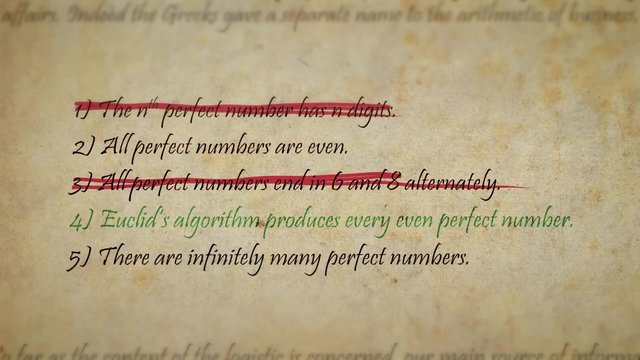 computers have been incredibly successful at finding new mersenne primes and their corresponding perfect numbers, but we've still only found 51 so far, so you might suspect that there are only a finite number of them, which would mean that nicomachus's fifth conjecture 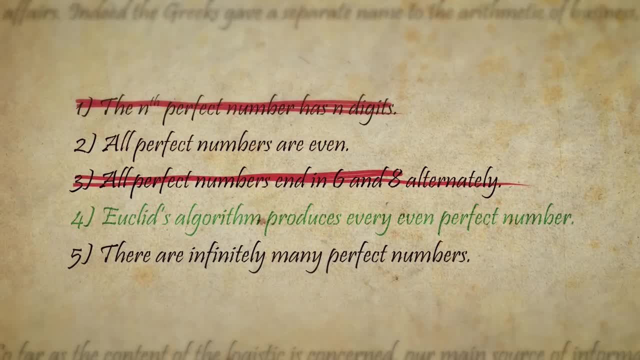 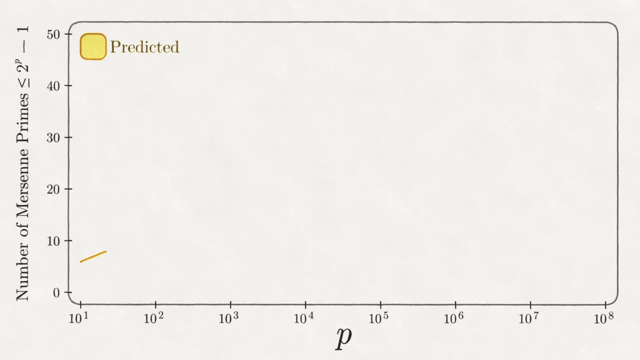 would be false that there aren't infinitely many perfect numbers, but that might not be the case. the lenstra- pomerantz- wagstaff conjecture predicts how many mersenne primes are in the world, and how many mersenne primes are in the world should appear based on how large p is now. this is the actual data. the conjecture performs remarkably. 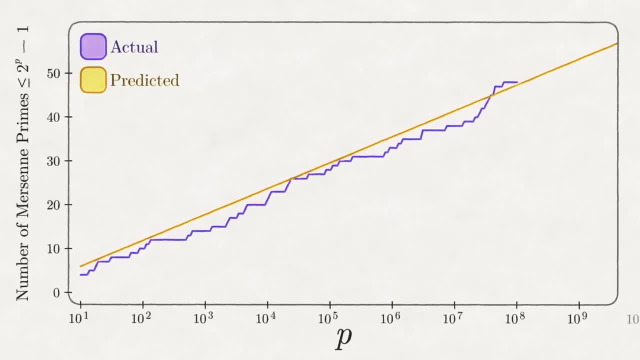 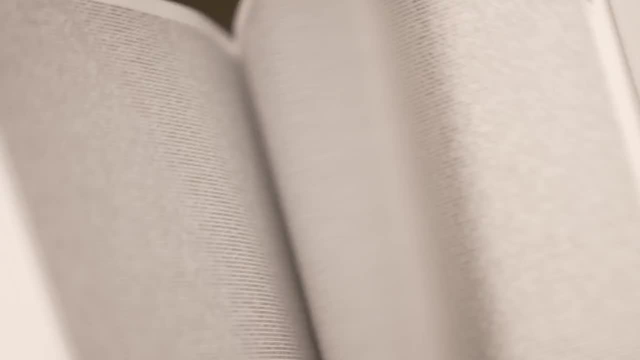 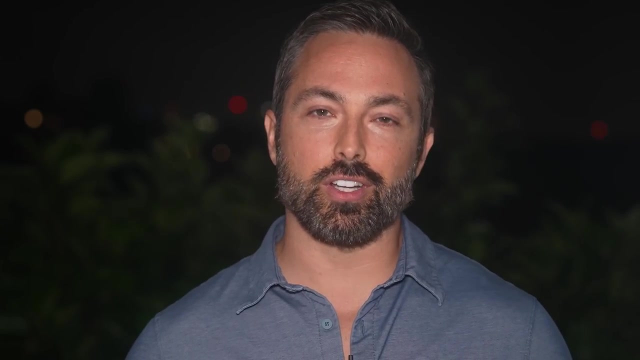 well. but more importantly, it predicts that there are infinitely many mersenne primes and so infinitely many even perfect numbers. the mersenne primes are just so large and rare that they take a lot of time and computer resources to find. but a conjecture is not a proof and up until this day this problem shares the title of. 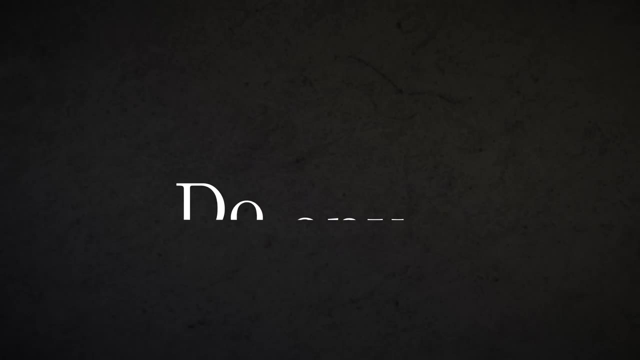 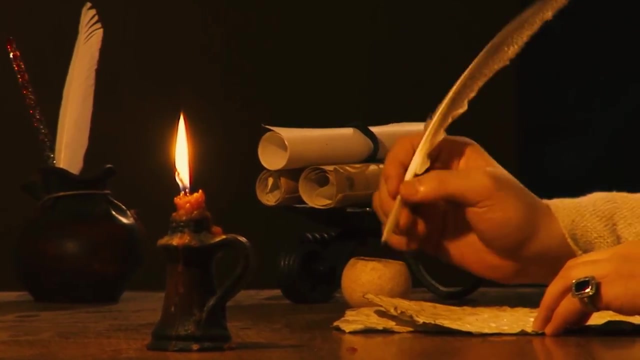 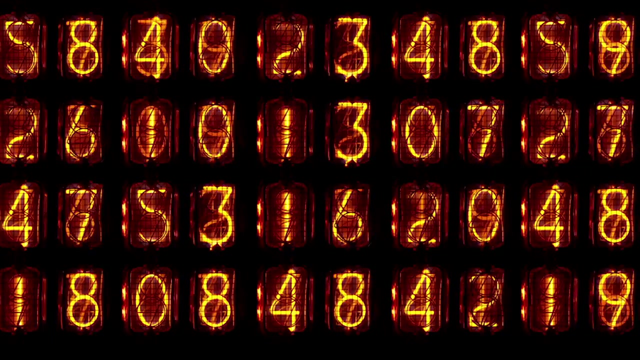 oldest unsolved problem in math with the other open problem: do any odd perfect numbers exist? the easiest way to solve this problem is by finding an example, so maybe we could just check different odd numbers and see if one of them is perfect. that's exactly what researchers tried in 1991 by using a smart algorithm called a factor chain. 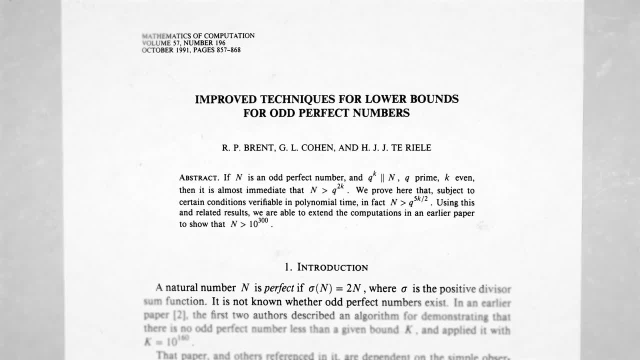 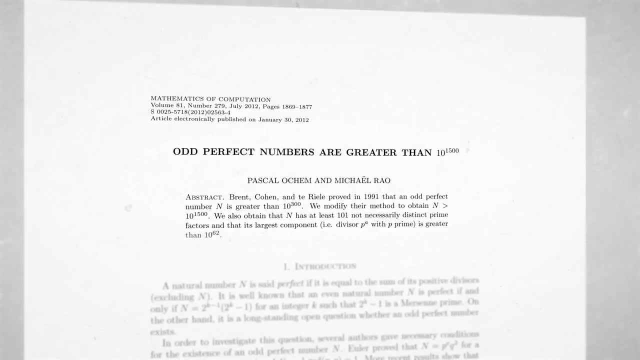 they were able to show that if an odd perfect number does exist, it must be larger than 10 to the power of 300.. 21 years later, pascal oakum and michael rao raised that lower bound to 10 to the 1500. 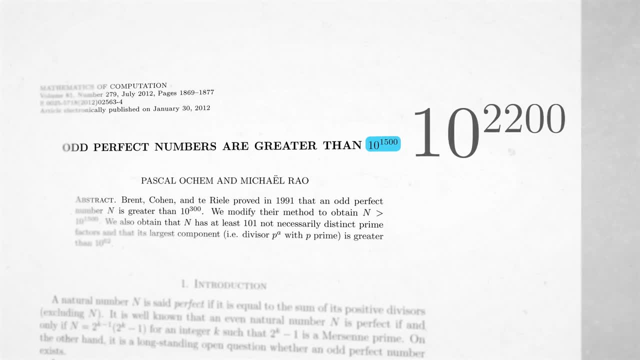 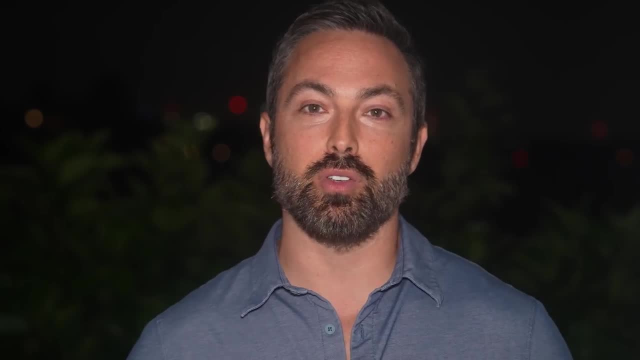 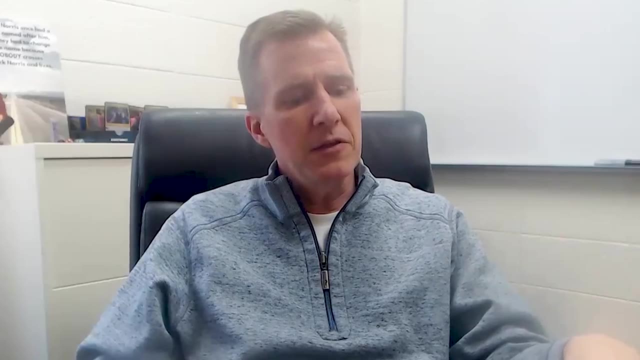 with recent progress pushing that number up to 10, to the 2200. with numbers that large, it's unlikely that a computer will find one anytime soon, so we'll need to get smart. what would a proof look? like, like, how could we actually prove this? i i think the main idea that people have been trying to approach this problem with is coming: 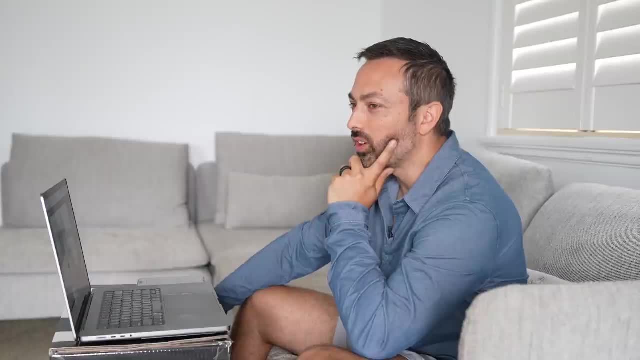 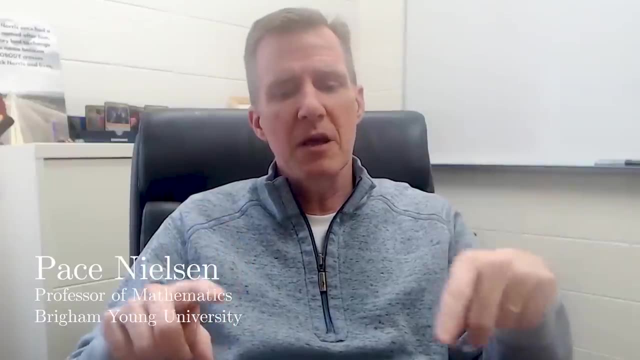 So we'll need to get smart. What would a proof be? What would a proof look like, Like, how could we actually prove this? I think the main idea that people have been trying to approach this problem with is coming up with more and more conditions. odd, perfect numbers have to satisfy. 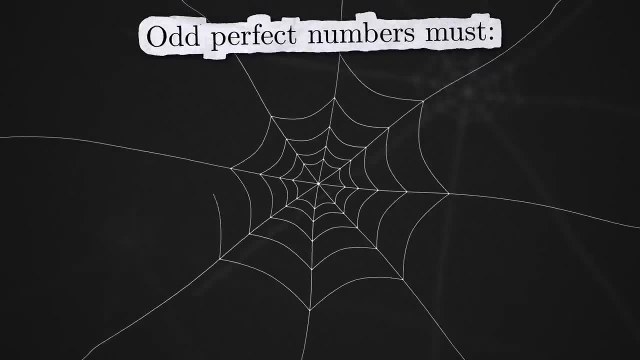 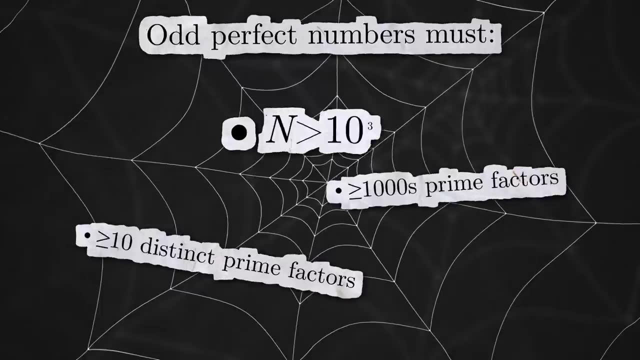 It's called this web of conditions, where it has to have 10 prime factors, now that we know, and maybe thousands of non-distinct prime factors, and it has to be bigger than 10 to the 3,000, and it has to do all these different things and we hope that eventually there's 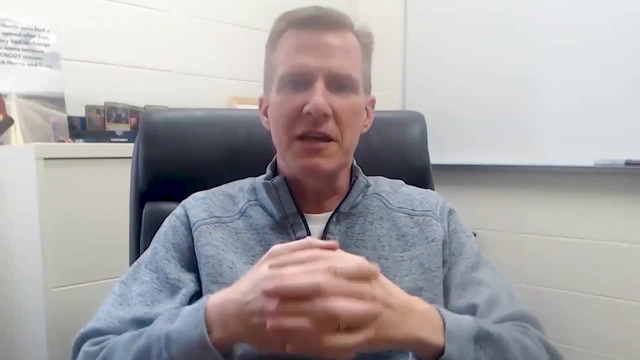 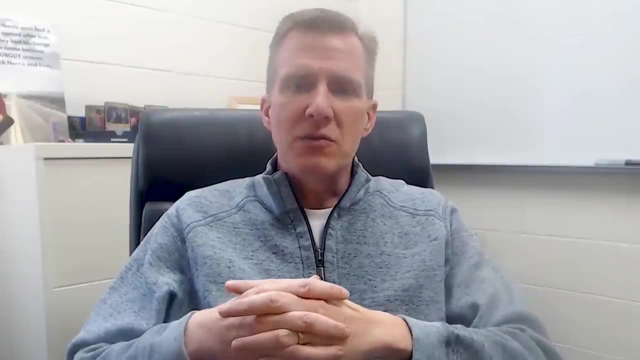 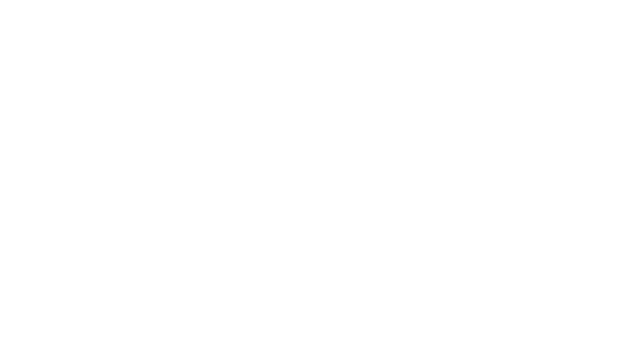 so many conditions that constrain the numbers so much that they can't exist. Since Euler, mathematicians have kept adding new conditions to this web, But so far it hasn't worked. But there might be another path. When Descartes was looking for odd perfect numbers, he came across. 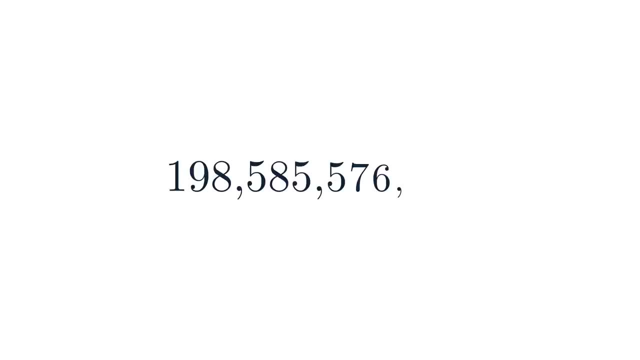 198,585,576,189, which you can factor as 3 squared times 7 squared times 11 squared times 13 squared times 22 squared, That's 22,021.. Put this into Euler's sigma function and you find it is equal to 2 times the original. 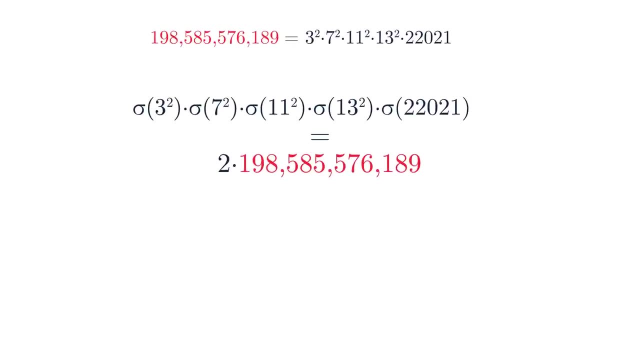 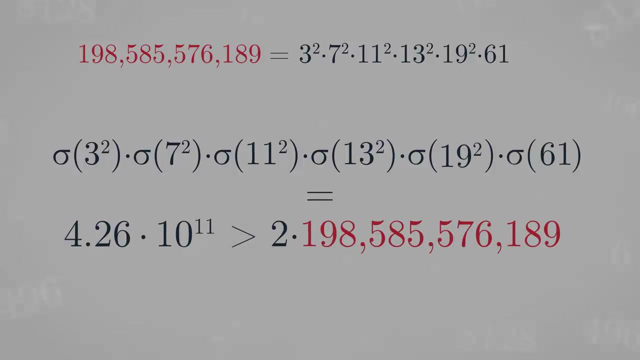 number. In other words, it is perfect. That is, if 22,021 were prime, But it's not, because it is equal to 19 squared times 61. And filling that in shows that it is not perfect. Numbers like this that are very close to being odd perfect numbers are called spoofs. 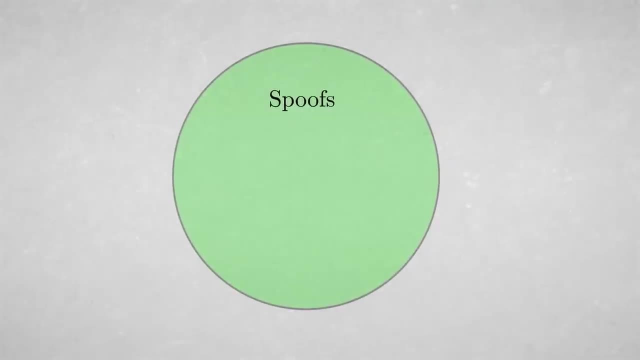 What are spoofs, Spoofs? Spoofs are a larger group of numbers, So odd, perfect numbers share all properties of spoofs and then a few extra ones, And the goal is to find properties of spoofs that ultimately prevent them from being odd. 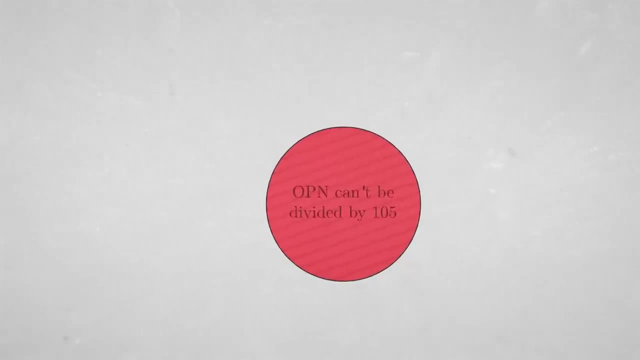 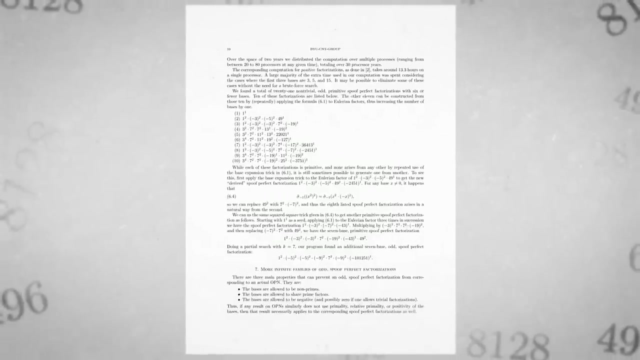 perfect numbers. For example, one condition of odd perfect numbers is that they can't be divided by 105. So if you find that spoofs must be divisible by 105, then this would prove that odd perfect numbers can't exist In 2022, Pace Nielsen and a team at BYU. 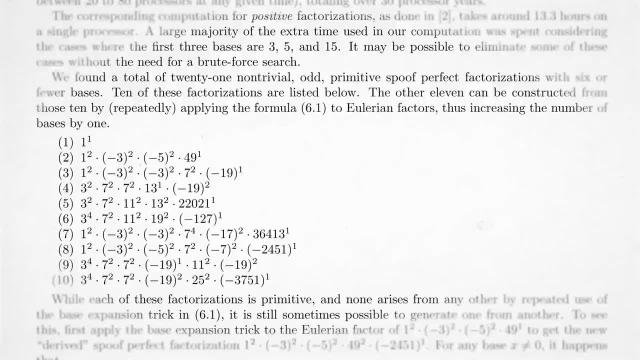 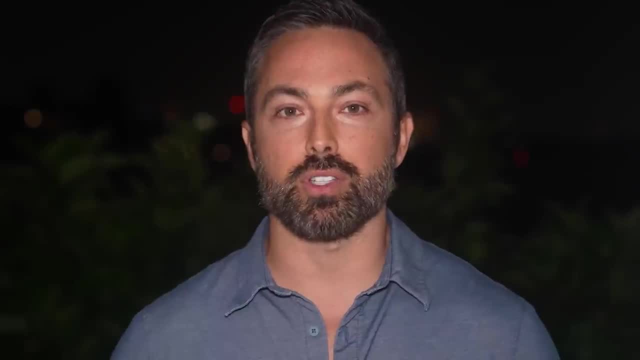 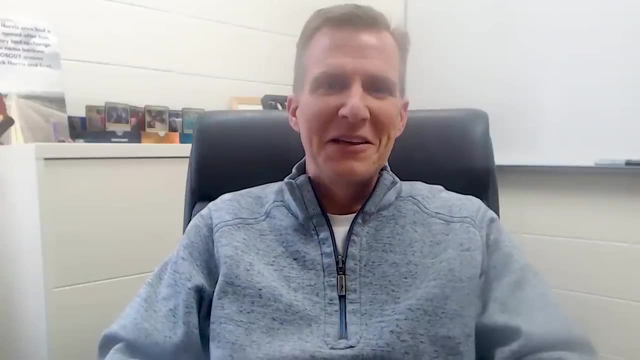 found 21 spoof numbers, including Descartes' number, And while they discovered some new properties of spoofs, they didn't find any that rule out odd perfect numbers. So how large would an odd perfect number have to be? They don't exist. 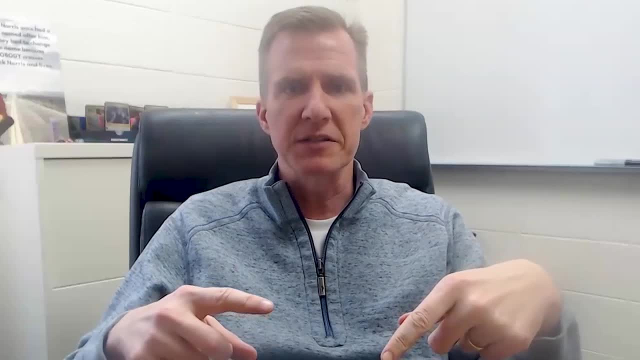 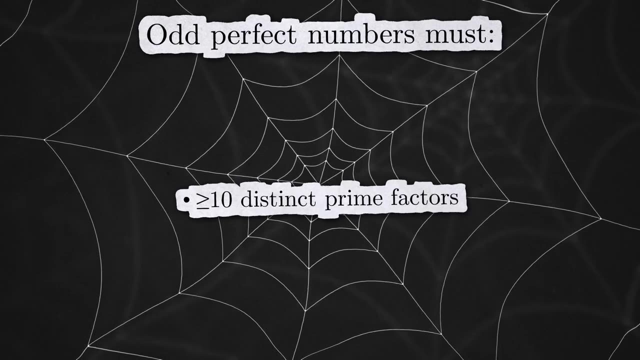 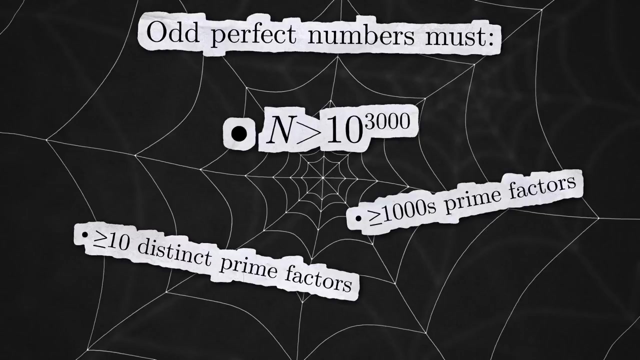 up with more and more conditions. odd perfect numbers have to satisfy. it's called this web of conditions, where it has to have 10 prime factors- now that we know- and maybe thousands of non-distinct prime factors, and has to be bigger than 10 to the 3000, and it has to do all these different things and we hope that eventually, 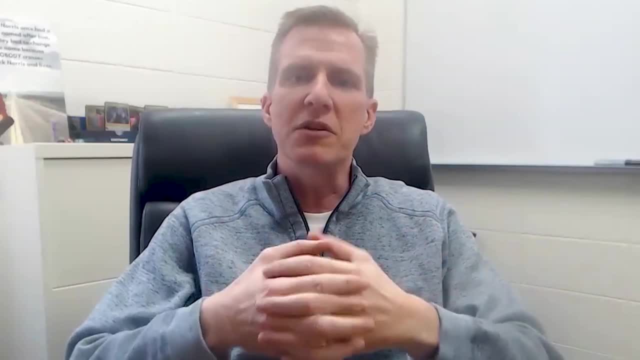 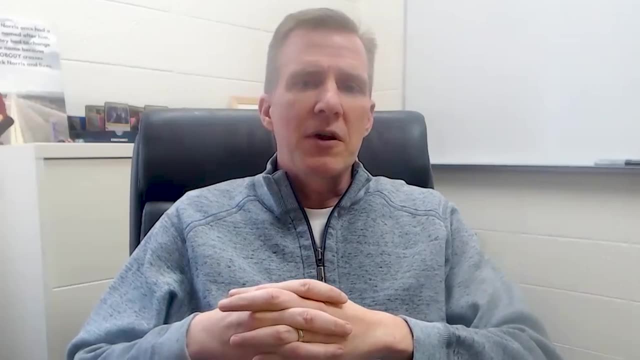 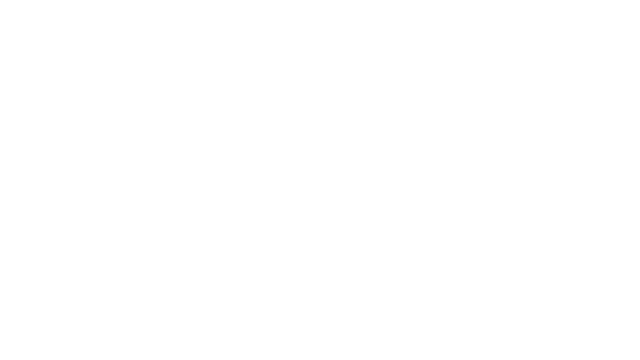 there's just so many conditions. they constrain the numbers so much that they can't exist. since euler, mathematicians have kept adding new conditions to this web, but so far it hasn't worked. but there might be another path. when descartes was looking for odd perfect numbers, he came across 198 billion 585 million 576 189. 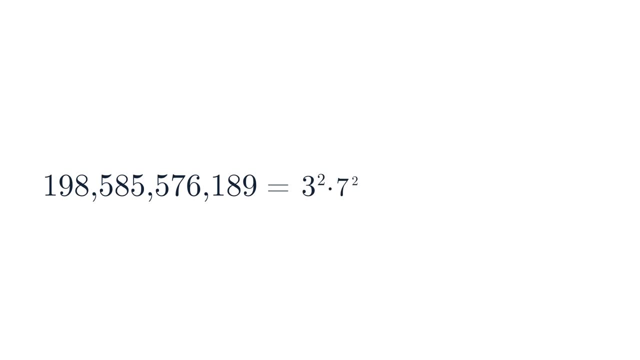 which you can factor as 3 squared times 7 squared times 11 squared times 13 squared times 22 021. put this into euler's sigma function and you find it is equal to 2 times the original number. in other words, it is perfect. 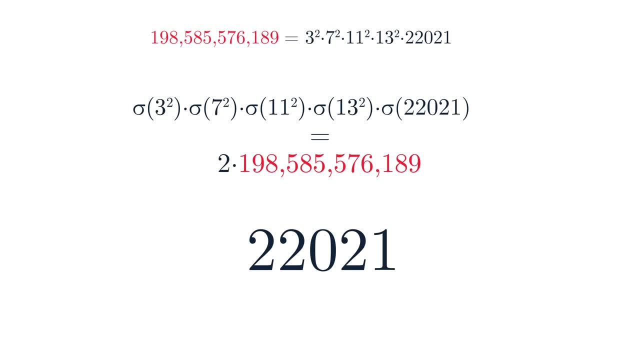 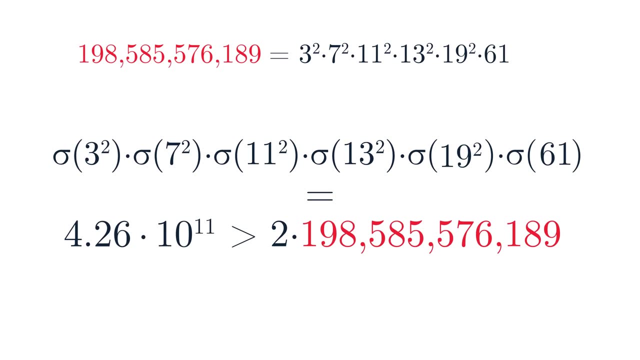 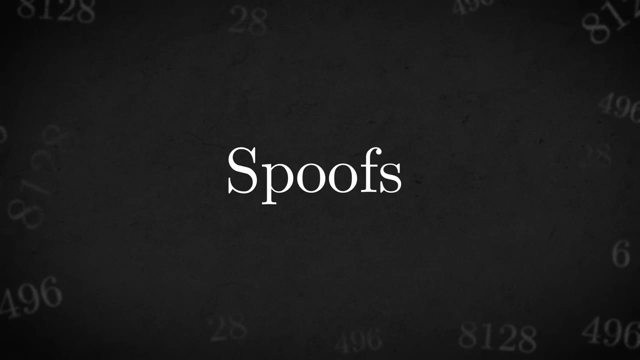 that is, if 22 021 were prime, but it's not, because it is equal to 19 squared times 61 and filling that in shows that it is not perfect. numbers like this that are very close to being odd perfect numbers are called spoofs. spoofs are a larger group of numbers, so odd perfect numbers share all properties of spoofs. 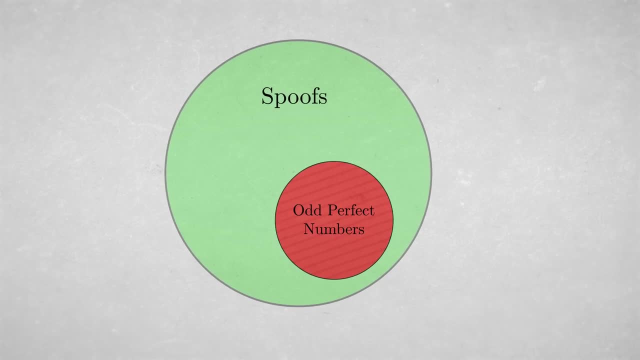 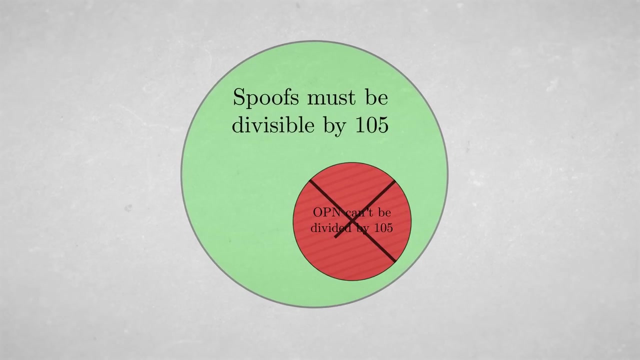 and then a few extra ones, and the goal is to find properties of spoofs that ultimately prevent the them from being odd-perfect numbers. For example, one condition of odd-perfect numbers is that they can't be divided by 105. So if you find that spoofs must be divisible by 105, then this would prove that odd-perfect. 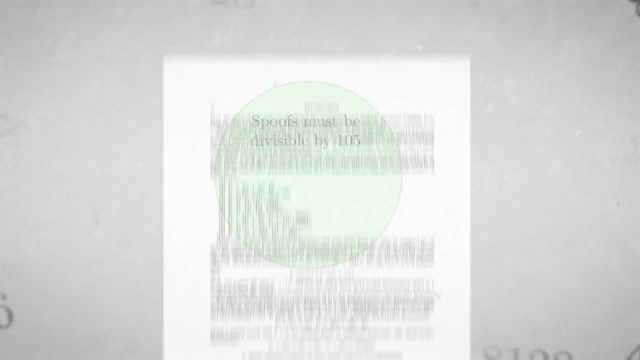 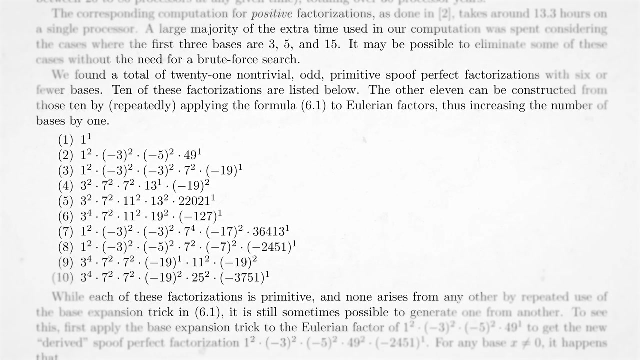 numbers can't exist. In 2022,, Pace Nielsen and a team at BYU found 21 spoof numbers, including Descartes' number, And while they discovered some new properties of spoofs, they didn't find any that rule out odd-perfect numbers. 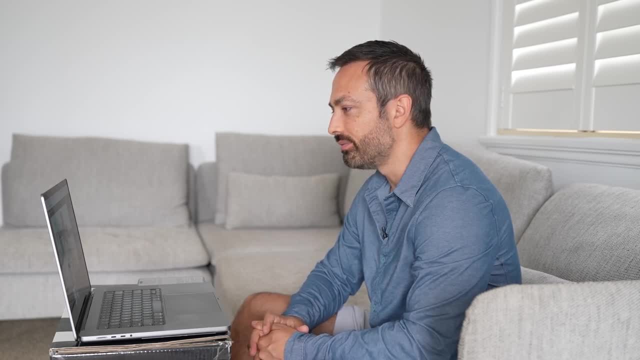 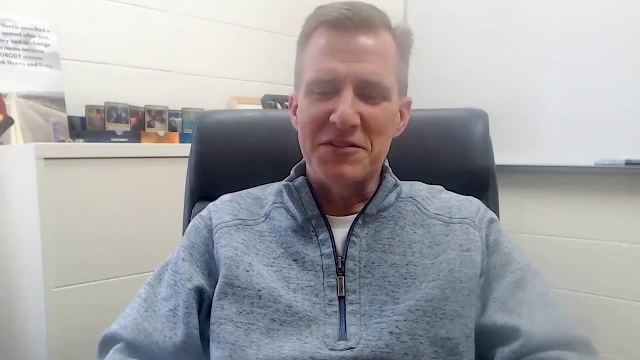 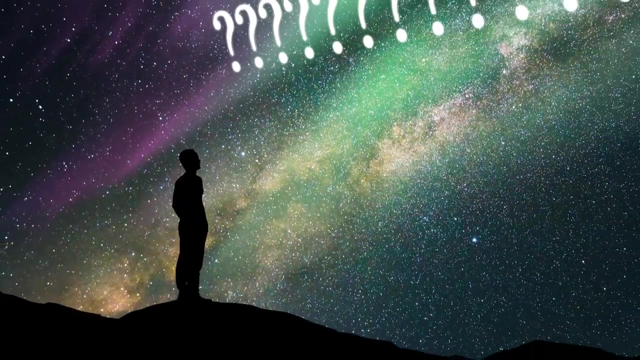 So how large would an odd-perfect number have to be? They don't exist. You don't think odd-perfect numbers exist. No, they don't exist. I wish they did. that'd be really cool if there was just this one gigantic odd-perfect. 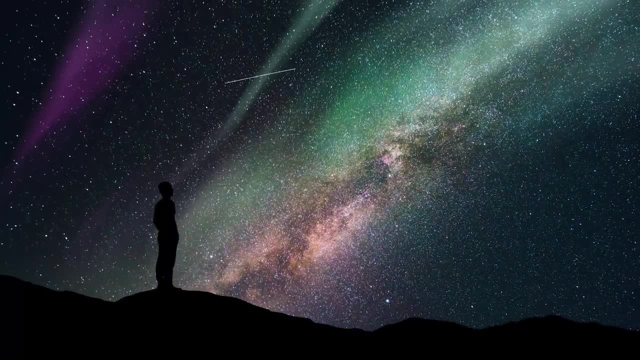 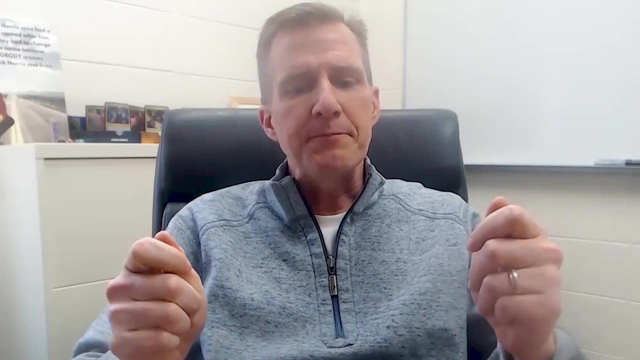 number out in the universe. They don't exist. No, How are you convinced that they don't exist? There is. There's something called a hierarchy. It's a heuristic argument where it's not a proof. so if we had a proof, we'd be done. 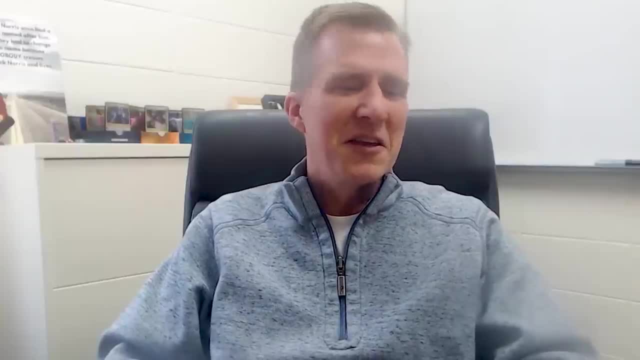 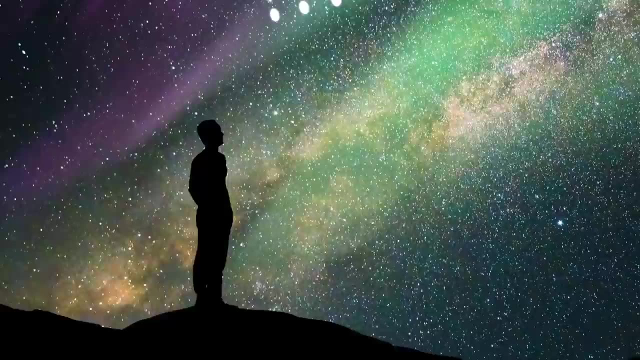 You don't think odd perfect numbers exist. No, they don't exist. I wish they did. that'd be really cool if there was just this one gigantic odd perfect number, Gigantic odd perfect number out in the universe. they don't exist, no. How are you convinced that they don't exist? There is something called a heuristic argument where it's not a proof. So if we had a proof we'd be done. It's just an argument from okay. we think primes occur this often of this type and 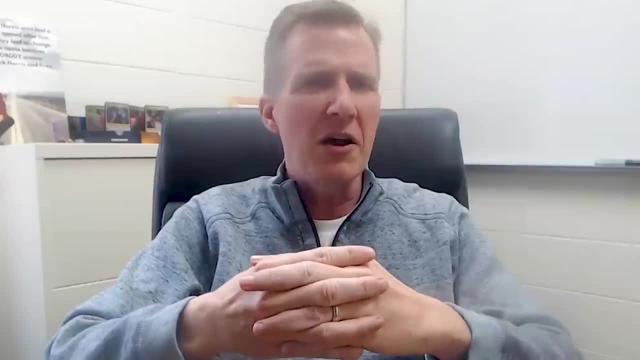 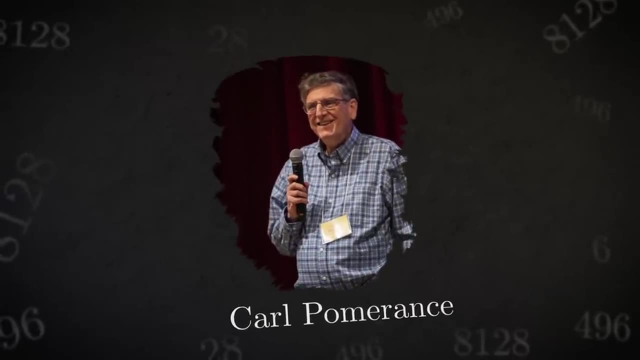 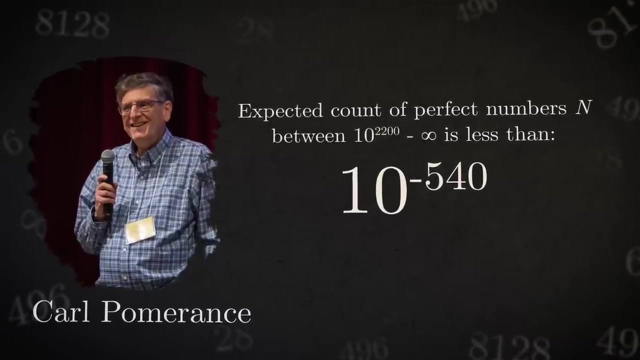 you put those pieces of information together and you think: okay, on average, how many numbers should be perfect? This argument, which was made by Karl Pomerantz, predicts that between 10 to the 2200 and infinity, there are no more than 10 to the negative 540 perfect numbers of the form n. 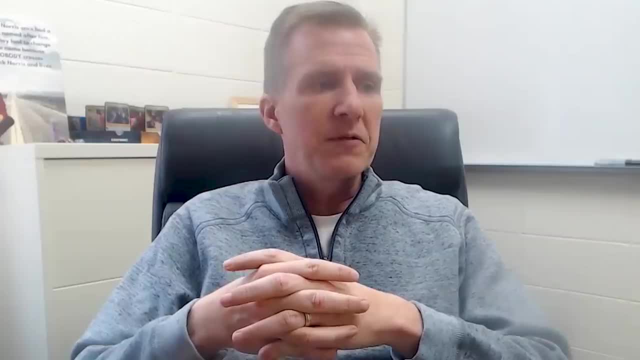 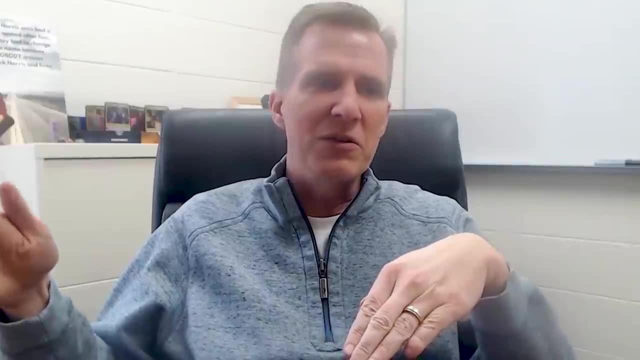 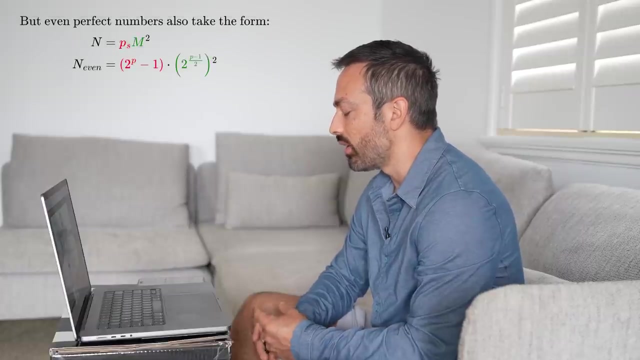 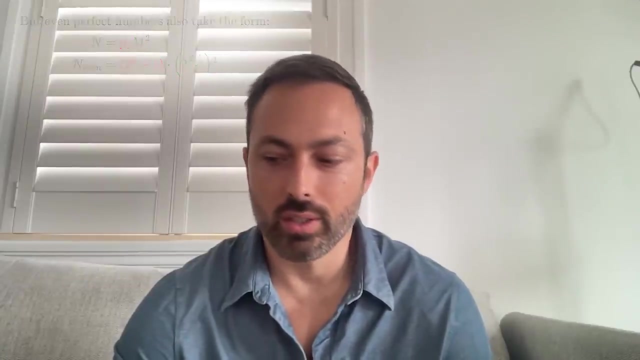 equals p, m squared With odd perfect numbers. the heuristic says: we shouldn't expect any. we've searched high enough. now that we think we have enough evidence, they shouldn't exist anymore. My understanding is this heuristic argument. It also predicts that there are no large perfect numbers, even or odd. 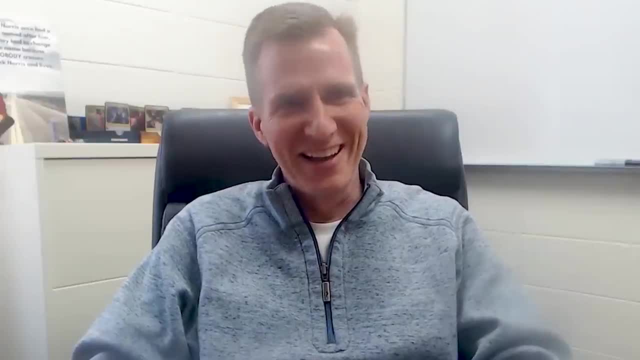 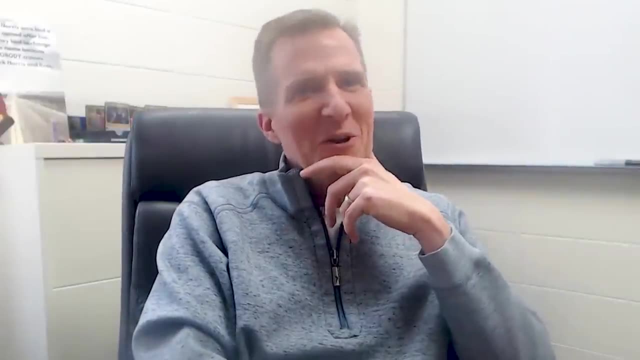 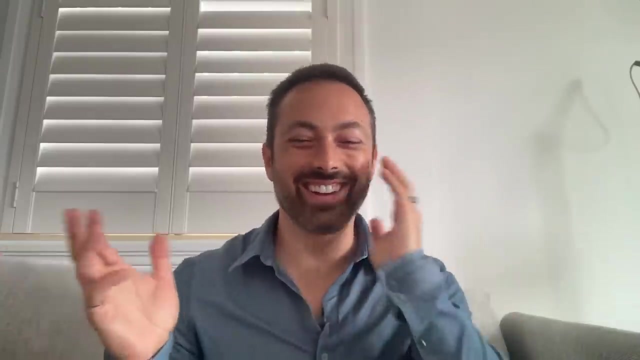 That's true. So there's a downside, because it says there shouldn't be large, even perfect, numbers, and we actually expect there to be infinitely many And so okay. so why do I believe the heuristic in this case and not this case? 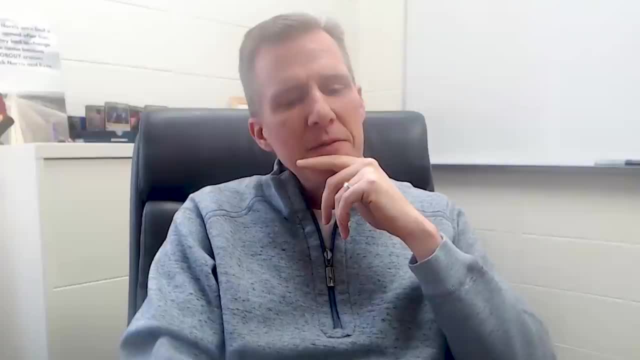 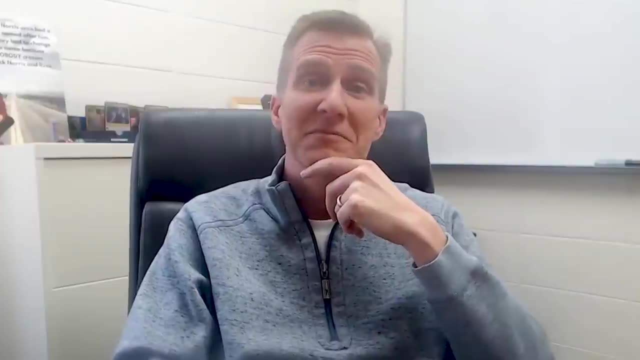 You're right. Am I being hypocritical about that? There are other aspects you can add on to the heuristic and make it stronger. Let me put it that way. But you're right, It's not a proof For now. this is still the oldest unsolved problem in math. 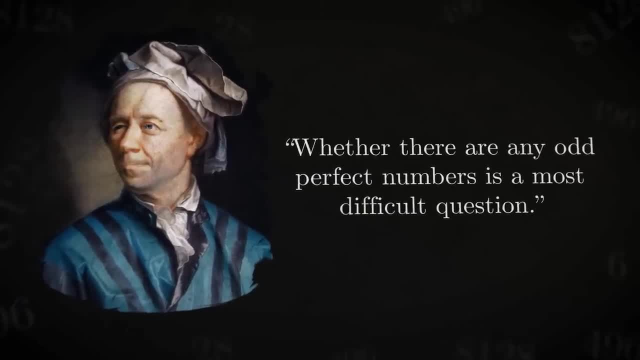 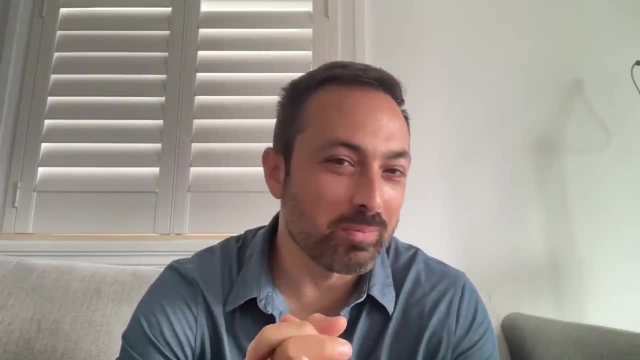 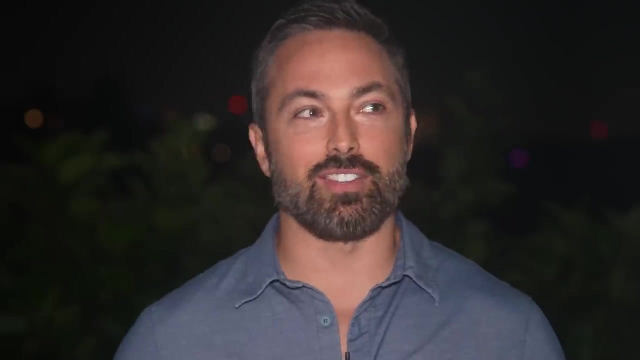 Euler was right when he said whether there are any odd perfect numbers is a most difficult question. So are there any applications of this problem? I can say no. Now many people may think that if there are no applications to the real world, then there's no point studying it. 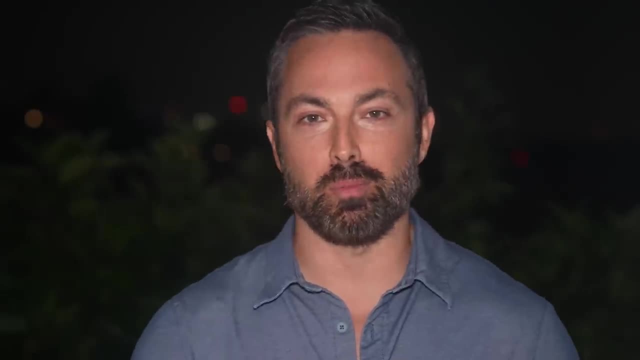 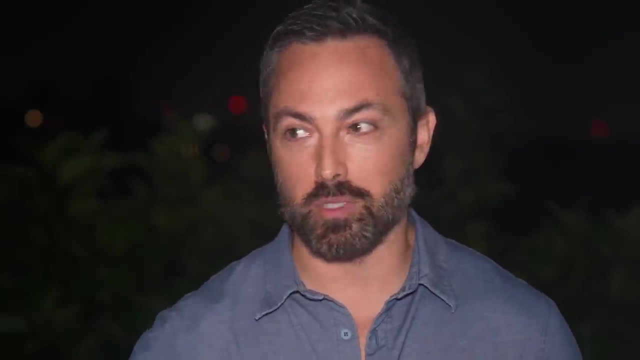 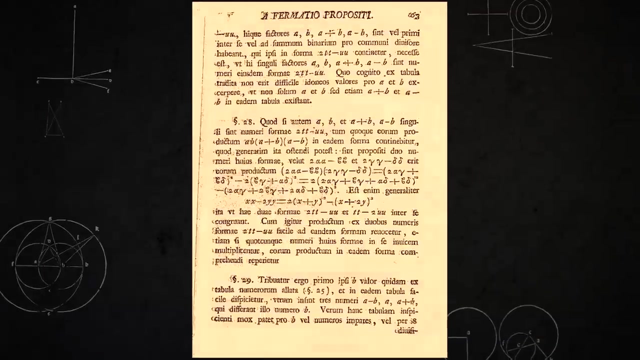 Why should anyone care about some old, unsolved problem? But I think that's the wrong approach. For more than 2000 years, number theory had no real world applications. It was just mathematicians following their curiosity and solving problems. they found interesting proving one result after another and building a foundation of useless mathematics. 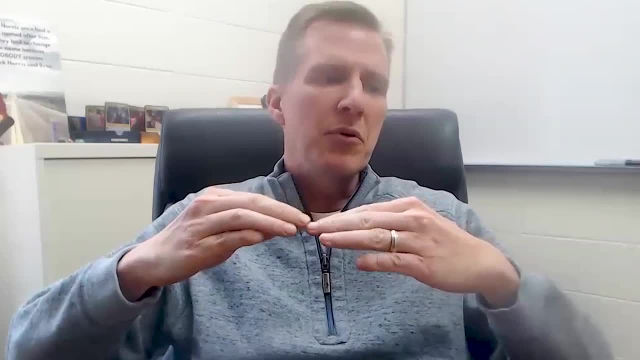 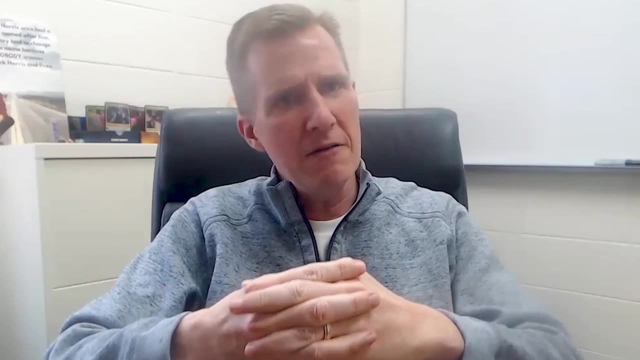 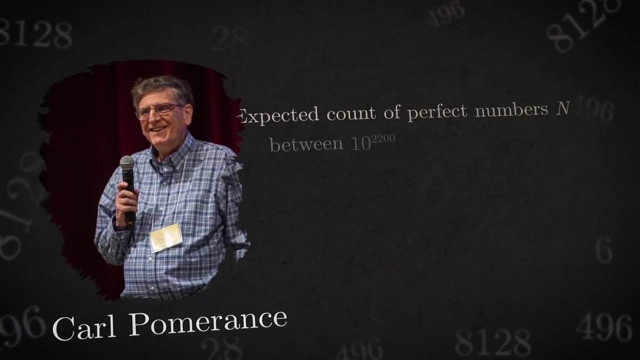 It's just an argument from: okay, we think primes occur this often of this type, and you put those pieces of information together and you think: okay, on average, how many numbers should be perfect? This argument, which was made by Karl Pomerantz, predicts that between 10 to the 2200 and infinity. 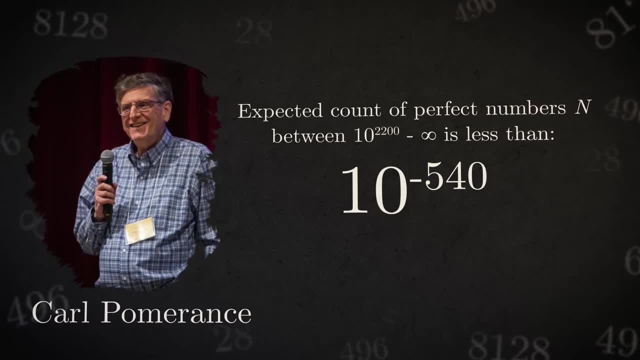 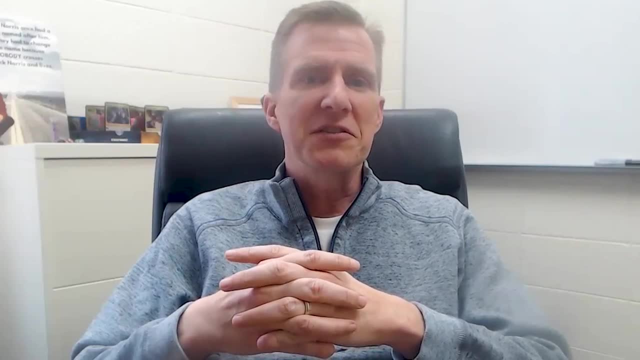 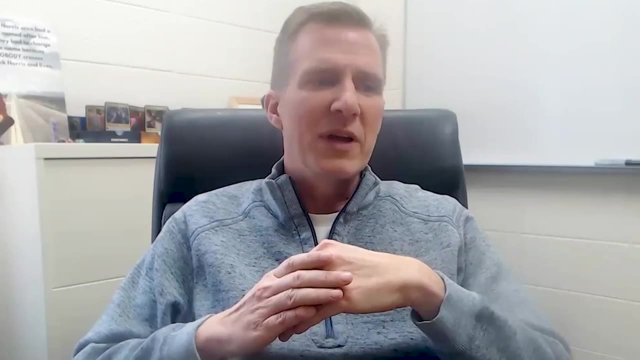 there are no more than 10 to the negative. 540 perfect numbers. It's just the numbers of the form. n equals pm squared With odd-perfect numbers. the heuristic says we shouldn't expect any. we've searched high enough. now that we think we have enough evidence, they shouldn't exist anymore. 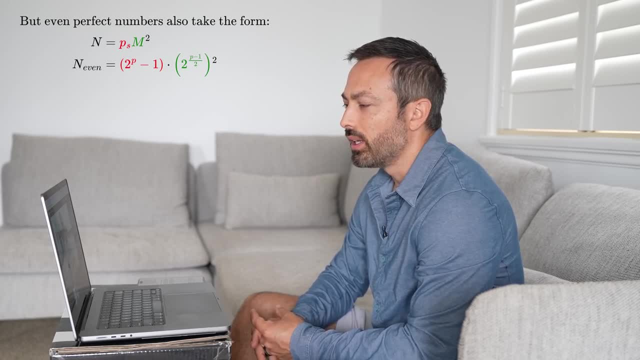 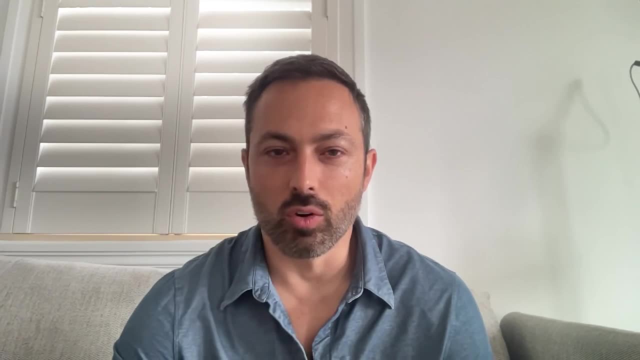 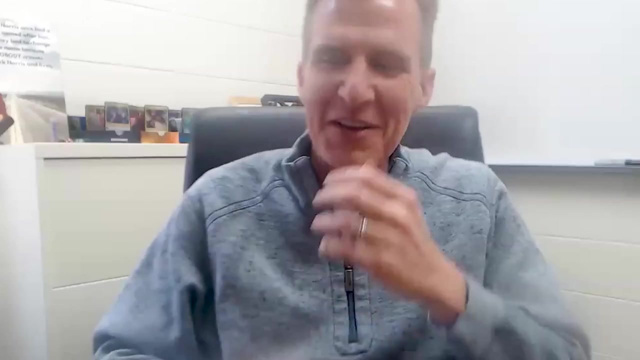 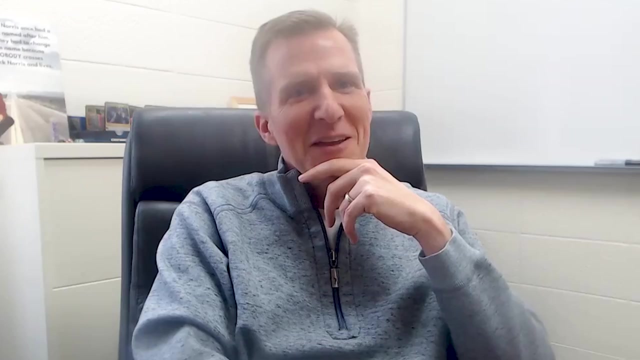 My understanding is this heuristic argument: it also predicts that there are no large, perfect numbers, even or odd. so That's true. So there's a downside to the heuristic. yeah, there's a downside, because it says there shouldn't be large, even perfect, numbers, and we actually expect there to be infinitely many. 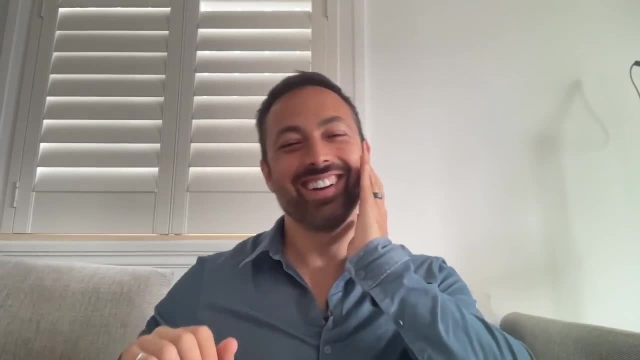 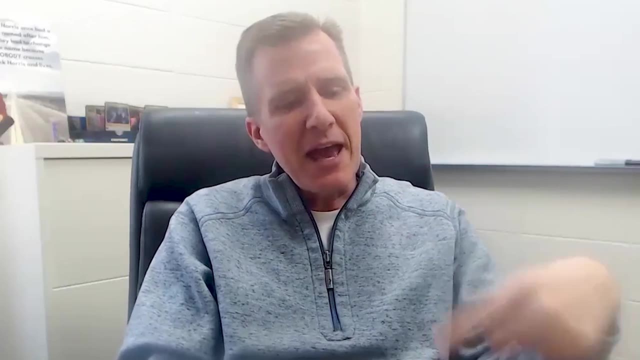 And so okay. so why do I believe the heuristic in this case and not this case? You're right. Am I being hypocritical about that? There are other aspects you can add on to the heuristic and make it stronger. let me put it that way. 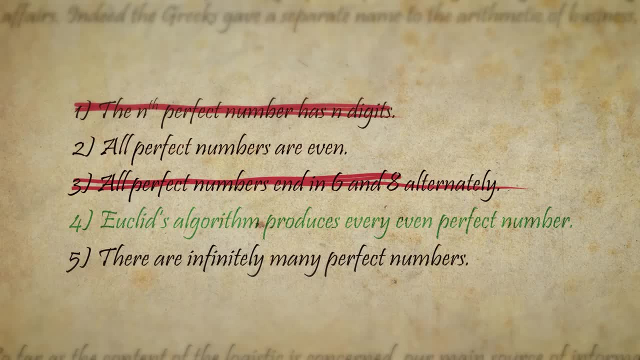 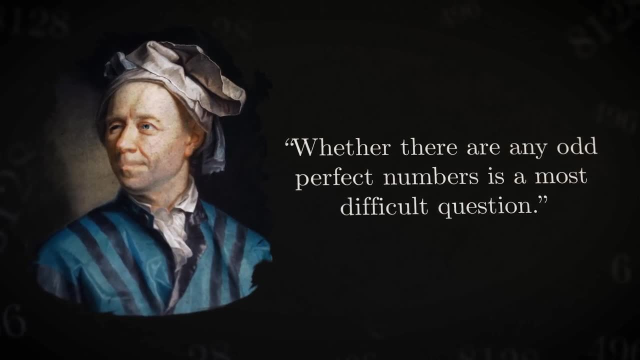 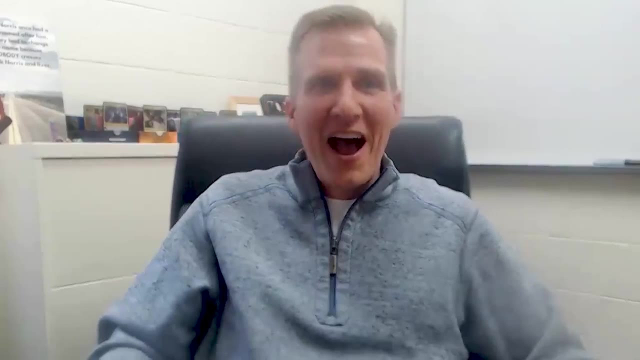 But you're right, it's not a proof For now. this is still the oldest unsolved problem. Euler was right when he said whether there are any odd perfect numbers is a most difficult question. So are there any applications of this problem? 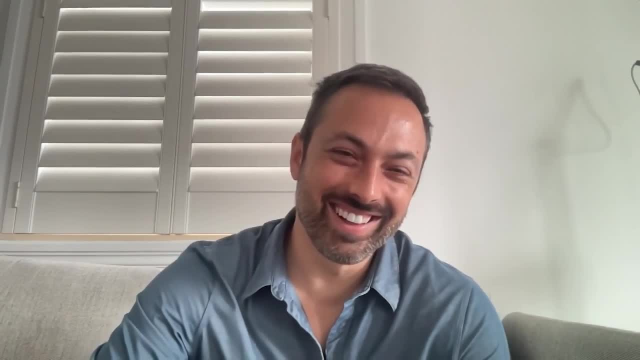 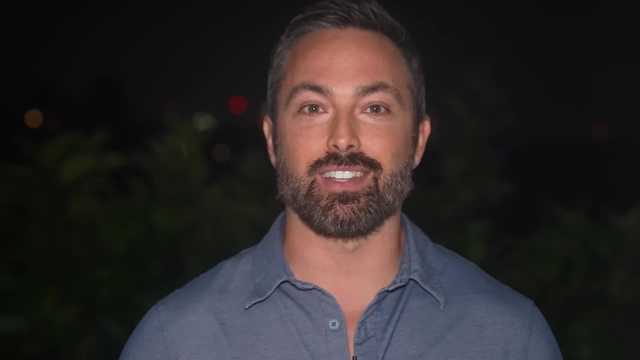 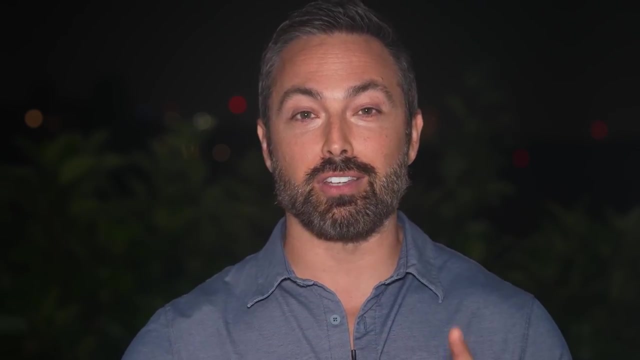 I can say no. Now many people may think that if there are no applications to the real world, then there's no point studying it. Why should anyone care about some old, unsolved problem? But I think that's the wrong approach. For more than 2,000 years, number theory had no real-world applications. it was just mathematicians. 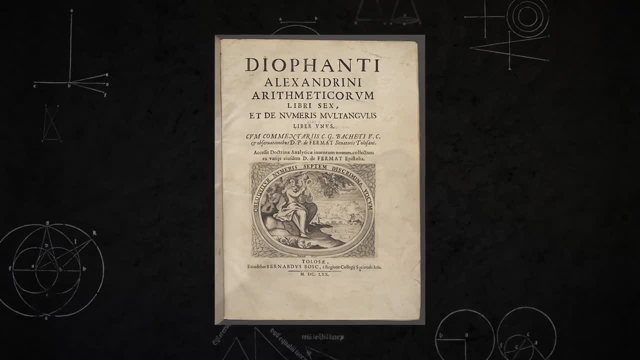 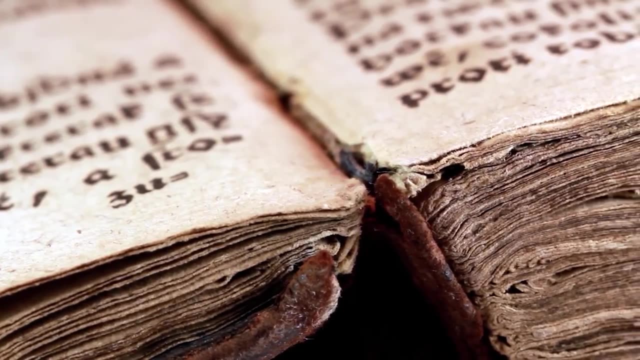 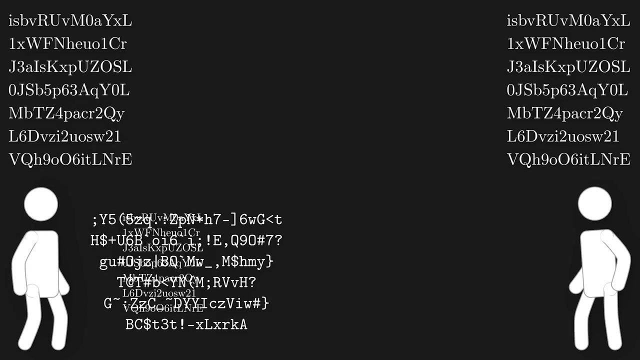 following their curiosity and solving problems. they found interesting proving one result after another and building a foundation of useless mathematics. But then, in the 20th century, we realized that we could take this foundation and base our cryptography on it. This is what protects everything from text messages to government secrets. 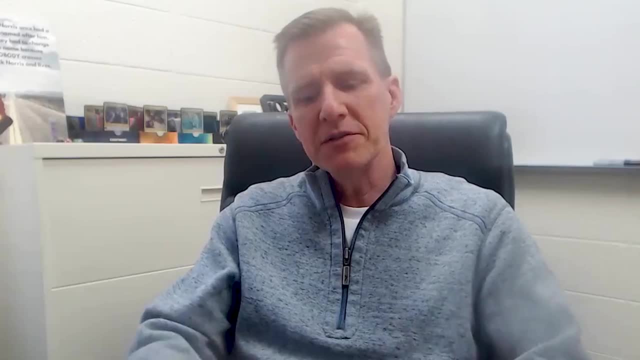 Whenever you have a group of people put their minds to war, they're not going to do anything. They're not going to do anything. They're not going to do anything. This is our problem. This isn't a problem. They're not going to do anything. 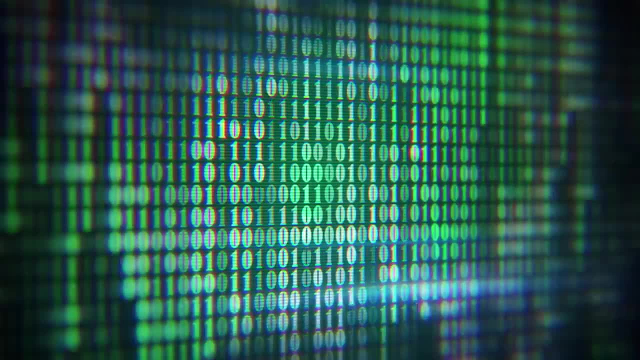 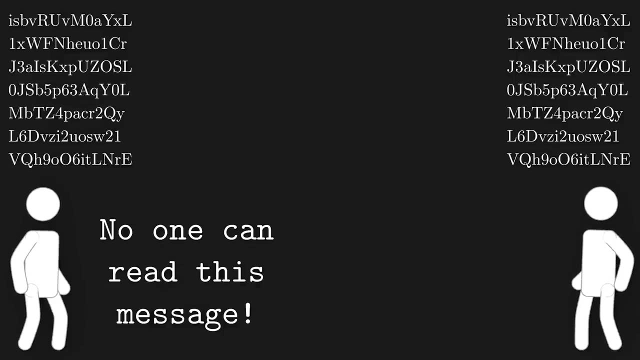 But then, in the 20th century, we realized that we could take this foundation And base our cryptography on it. This is what protects everything from text messages to government secrets. Whenever you have a group of people put their minds towards a problem, something good's. 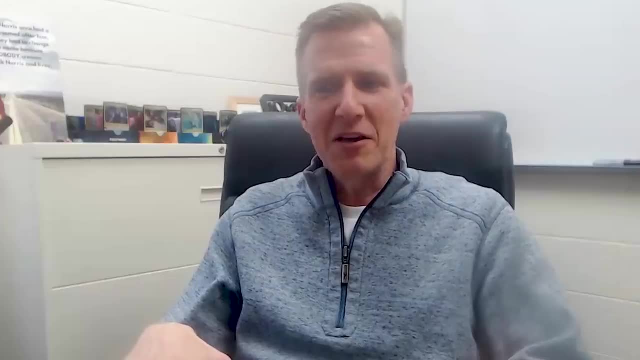 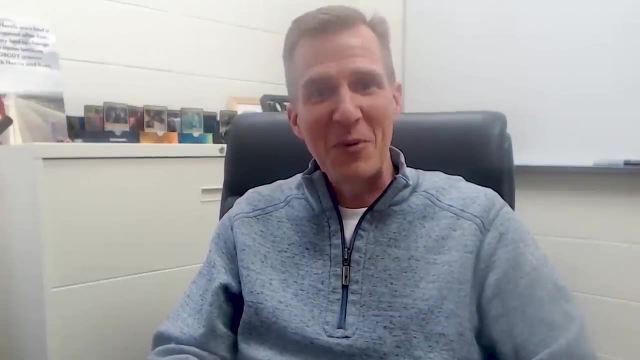 going to come out of it. If it's only at the beginning, this doesn't work. Okay, well, as Edison said, I learned 999 ways of not making a light bulb. eventually, I got a good way to do it. It's the same with math. 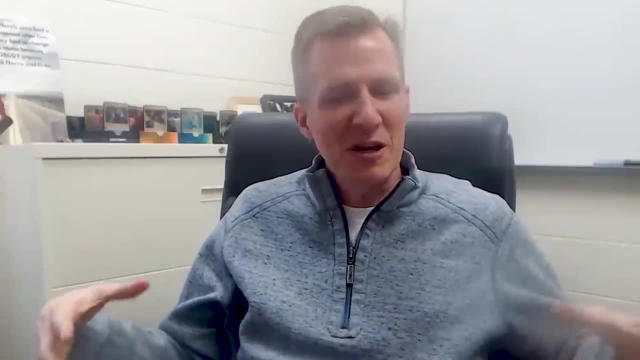 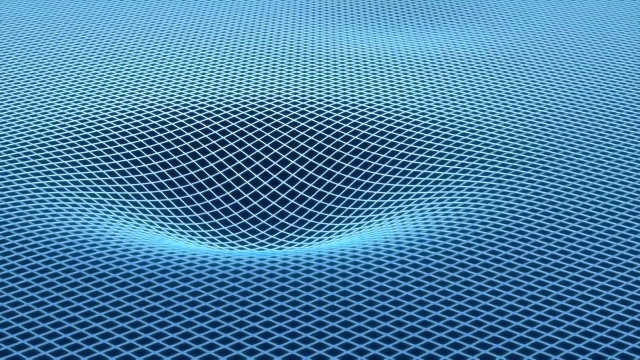 You have a problem And you throw your mind at it, And others do too, And you come up with new ideas, And eventually something good comes from that process. Einstein's general relativity was built on non-Euclidean geometries, Geometries that were developed as intellectual curiosities without foresight of how they 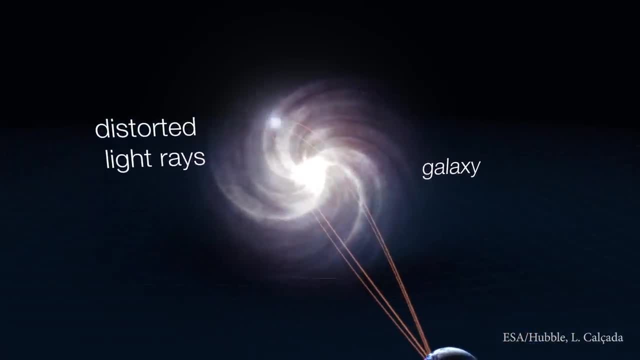 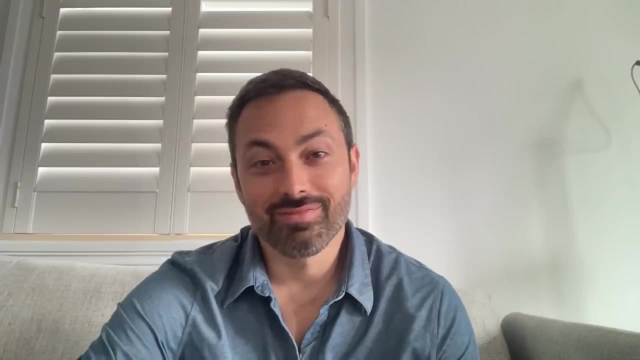 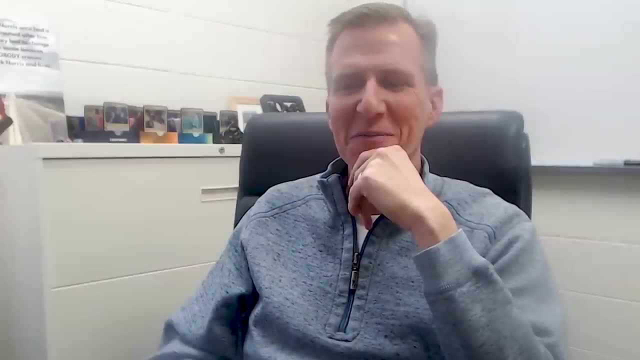 would one day change the way we understand the universe. How many people do you think are working on the problem of perfect numbers right now? I guess around 10 people currently have papers in the area 10 to 15.. If you're a high schooler and you just love mathematics and you think I want a problem, 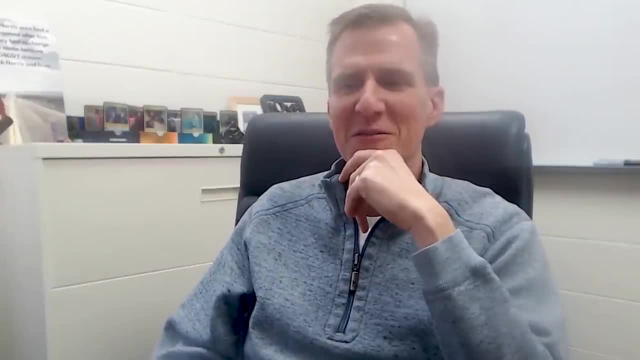 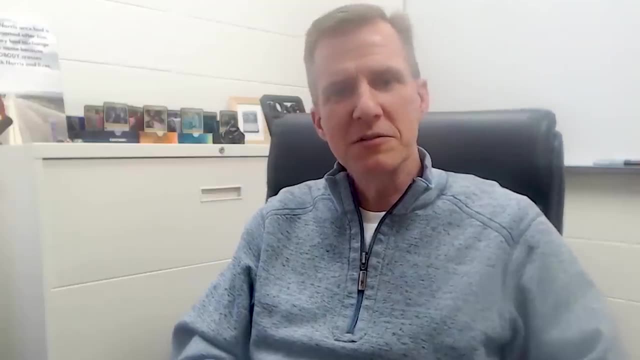 to think about. this one's a great problem to think about and you can make progress. you can figure out new things. yeah, don't be scared. Hundreds of people have thought about this problem for thousands of years. What can I do? 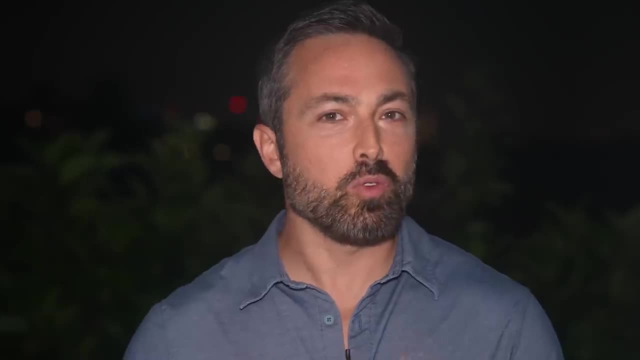 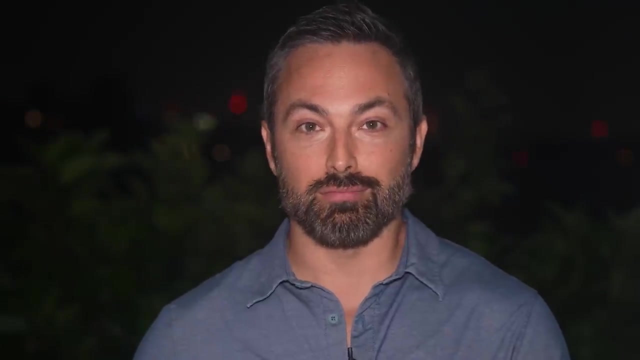 You can do something. Why should you do math if you don't know that it will lead anywhere? Well, because doing the math is the only way to know for sure. You can't tell in advance what the outcome will be Like. this problem might turn out to be a dud. 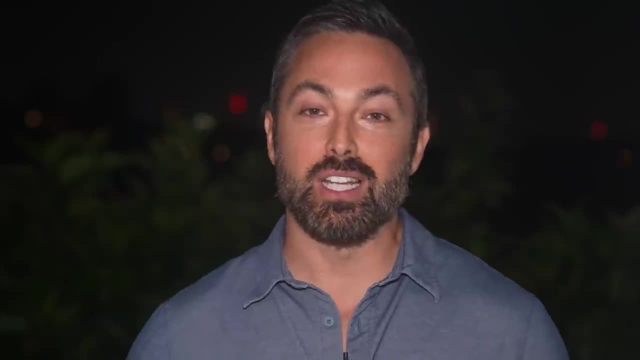 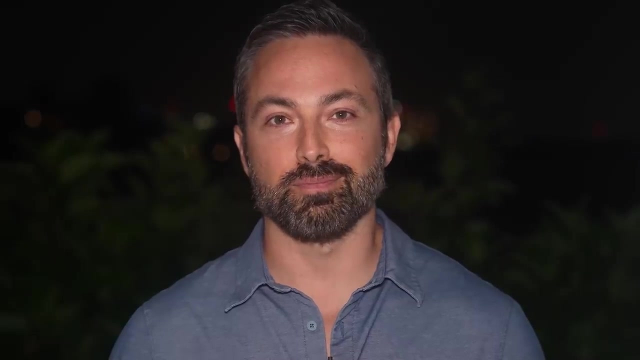 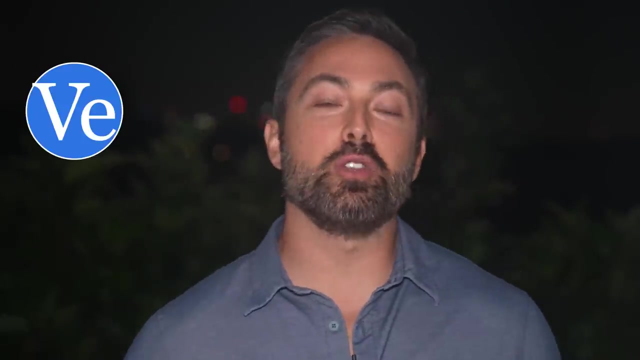 We might solve it, and it might not mean anything to anyone, Or it could turn out to be remarkably helpful. The only way to know for sure is to try. In today's world, it often feels like you've got to choose between following your curiosity. 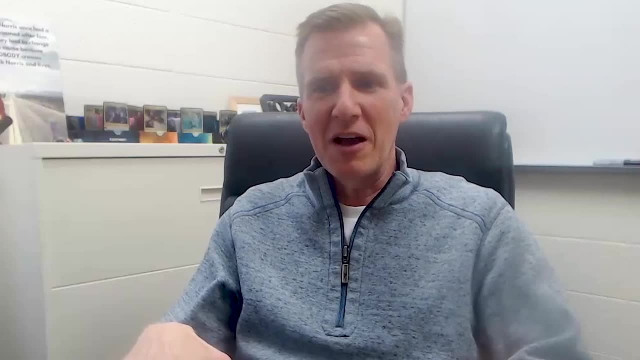 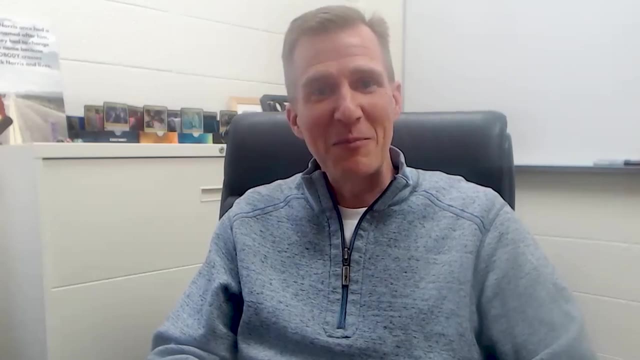 This is not a problem. If someone sets their minds towards a problem, something good's going to come out of it. If it's only at the beginning, this doesn't work. Okay, as Edison said, I learned 999 ways of not making a lightbulb. 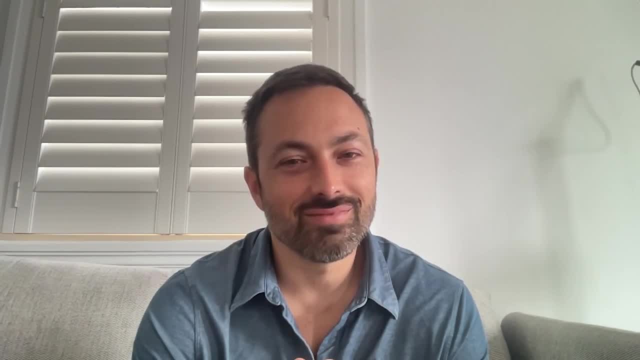 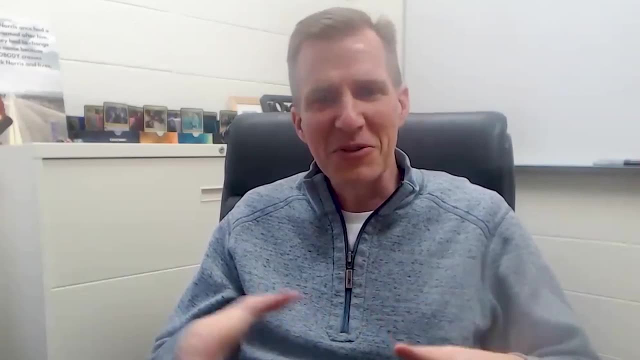 Eventually, I got a good way to do it. It's the same with math: You have a problem and you throw your mind at it, and others do too, and you come up with new ideas and eventually something good comes from that process. Einstein's General Relativity was built on non-Euclidean geometry. You don't have to be that fast to figure out what your problem is. It's not going to set you straight if you don't know. and if you don't know, you won't wanna. 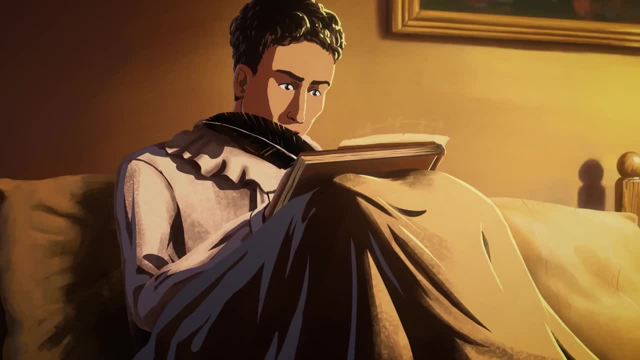 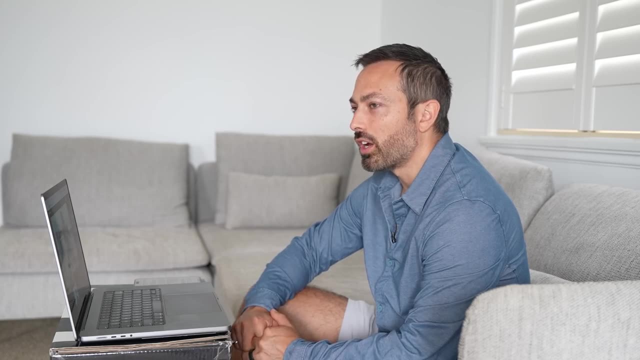 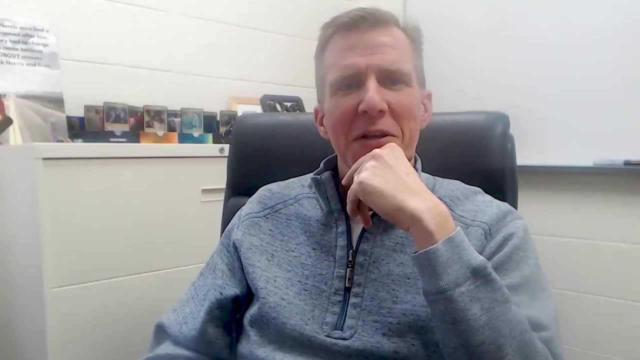 think about it: geometries, Geometries that were developed as intellectual curiosities, without foresight of how they would one day change the way we understand the universe. How many people do you think are working on the problem of perfect numbers right now? I guess around 10 people currently have. 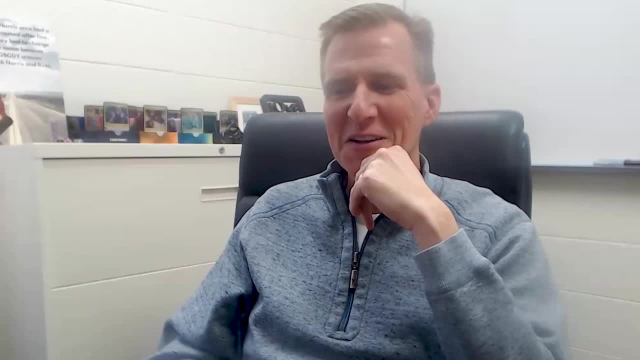 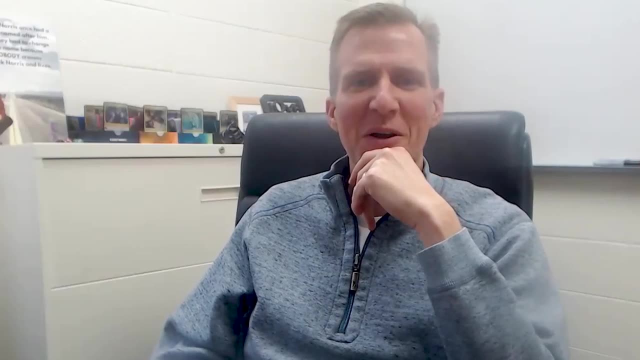 papers in the area 10 to 15.. If you're a high schooler and you just love mathematics and you think I want a problem to think about, this one's a great problem to think about and you can make progress. You can figure out new things. Yeah, don't be scared. Hundreds of people have thought. 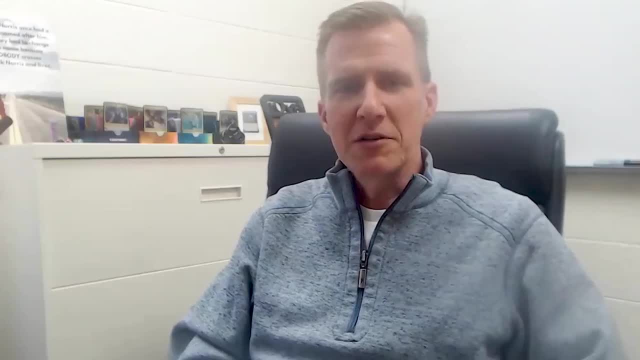 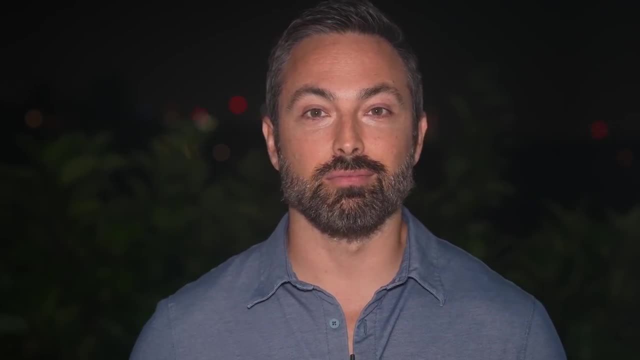 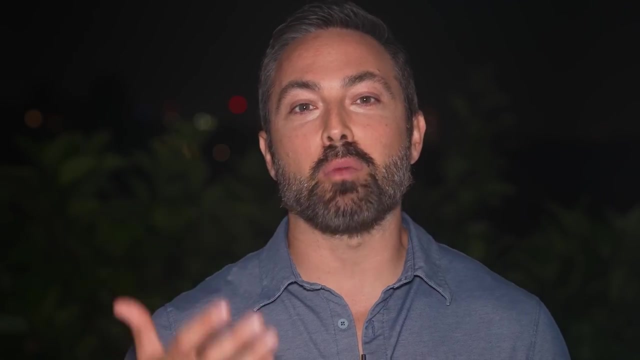 about this problem for thousands of years. What can I do? You can do something. Why should you do math if you don't know that it will lead anywhere? Well, because doing the math is the only way to know for sure. You can't tell in advance what the outcome will be. Like this: 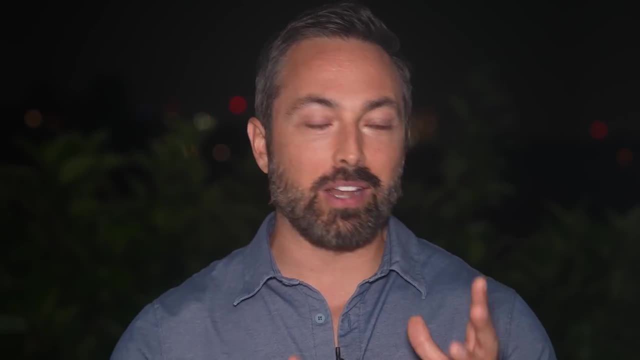 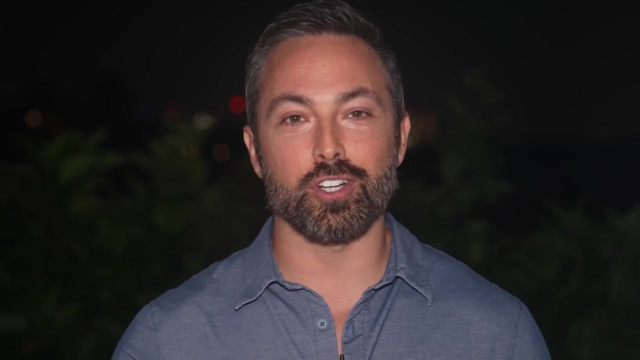 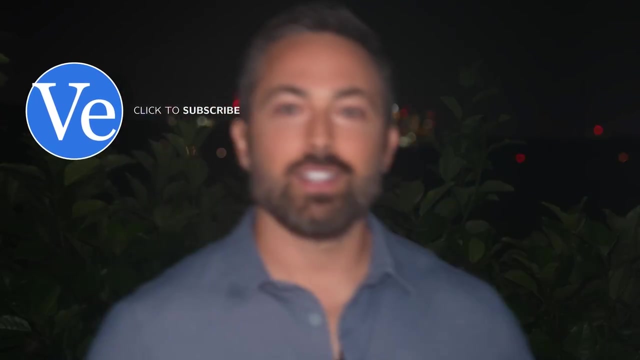 problem might turn out to be a dud. We might solve it and it might not mean anything to everybody, Or it could turn out to be remarkably helpful. The only way to know for sure is to try. In today's world, it often feels like you've got to choose between following your curiosity and 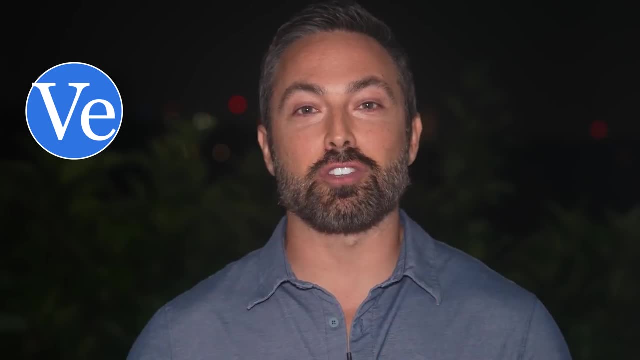 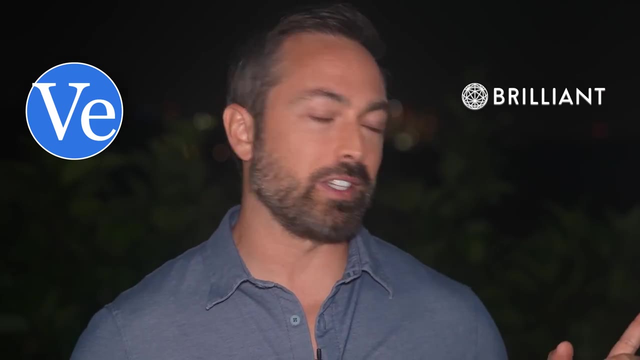 building real skills you can apply, But the truth is, it's essential to do both. Fortunately, there's one learning platform which allows you to do just that, And it's this video's sponsor, Brilliant. Brilliant will make you a better thinker, and 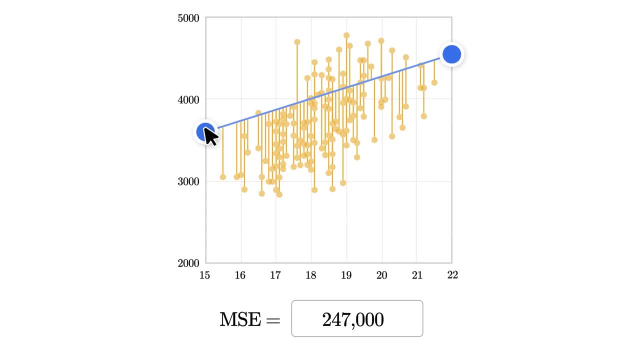 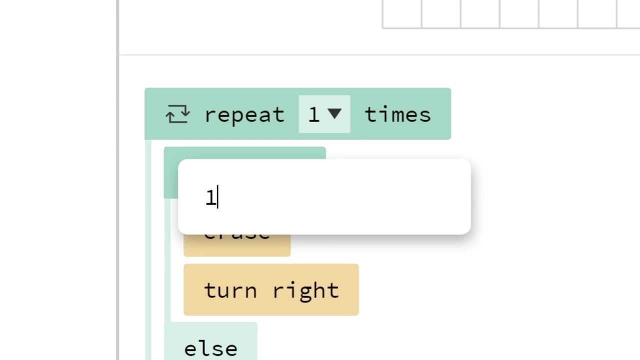 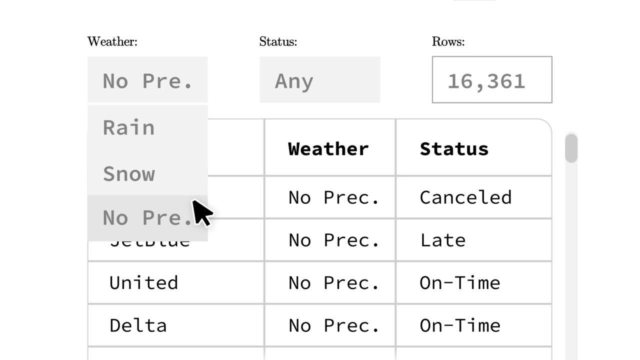 problem solver, And it's a great way to learn more about the problem of perfect numbers. Brilliant has thousands of lessons for you to explore, so you can follow your curiosity wherever it leads you, And you won't just learn key concepts, You'll actually apply that knowledge. 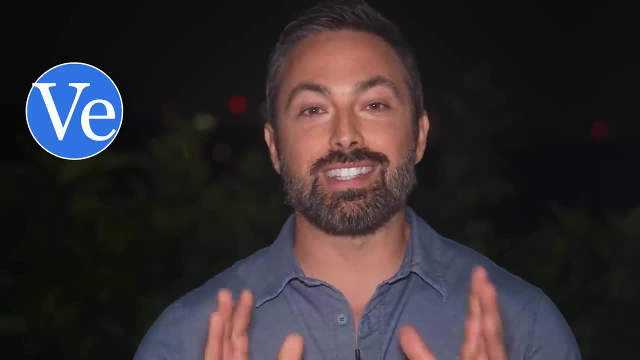 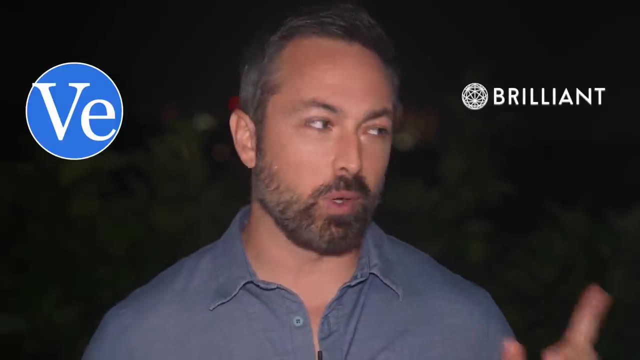 and building real skills you can apply, But the truth is, it's essential to do both. It's essential to do both. Fortunately, there's one learning platform which allows you to do just that, And it's this video's sponsor, Brilliant.